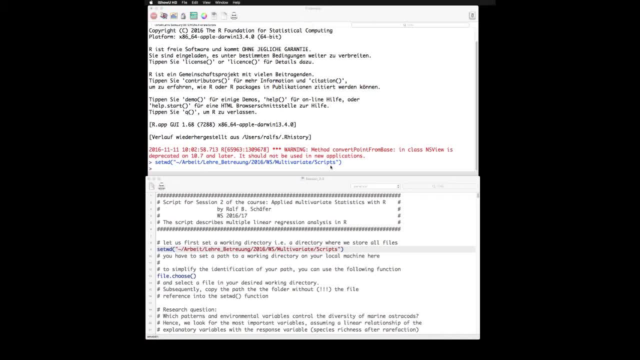 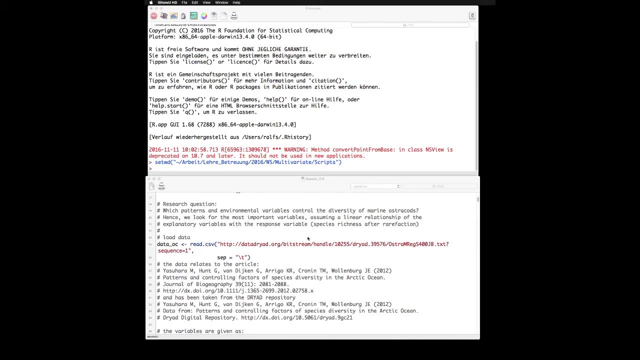 directory to your machine. In RStudio you have a direct option to set the working directory and move to the desired directory. Otherwise, you can use the filechoose command that has been shown in previous session. I won't deal with that here. The research question that we try to answer today is which patterns and environmental variables 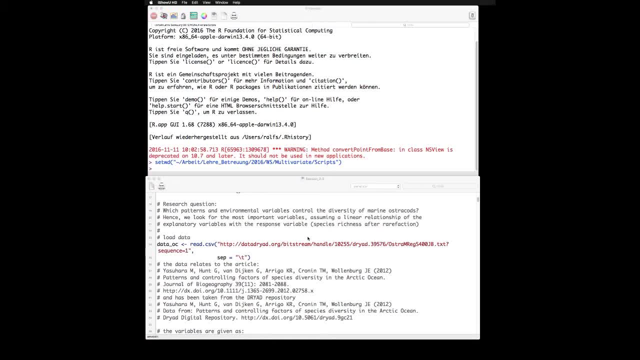 control the diversity of marine ostracodes, And this research question is a very important one. It is a very important one. This question is not just one that has been virtually constructed by me or anything. This is a research question related to a pattern. You find the article here. 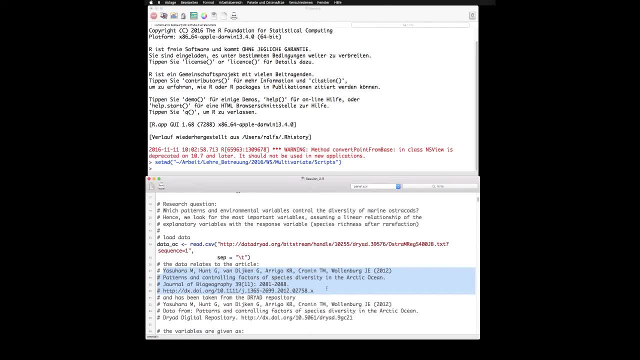 It has been published in Journal of Biogeography And the authors provide the full data in the Triad repository So we can use this original scientific data To repeat the analysis. Although we won't repeat it exactly, We will focus on the different 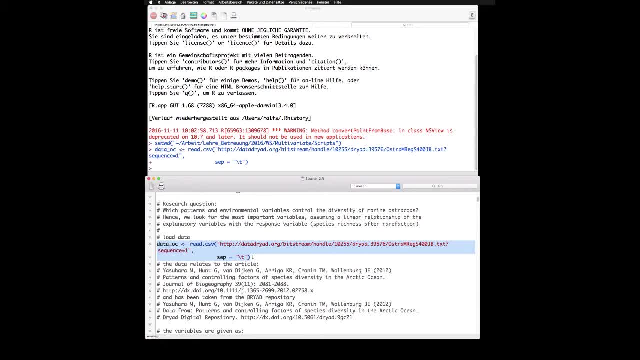 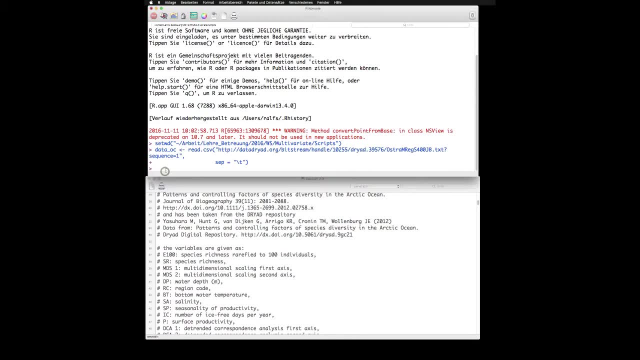 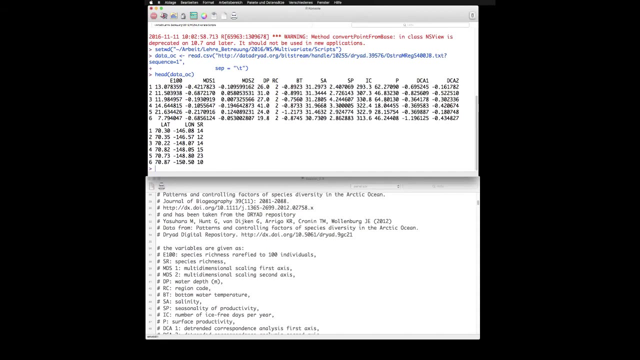 techniques that I explained in the lecture. So the first thing that we do is we load the data And once we have done this, we can have a look at the data. Everything went fine During loading. we see we have several variables here, And these variables 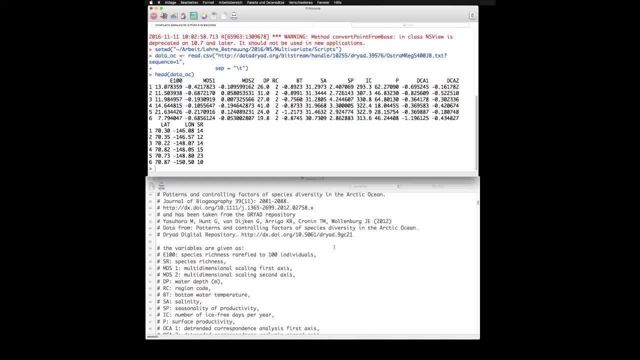 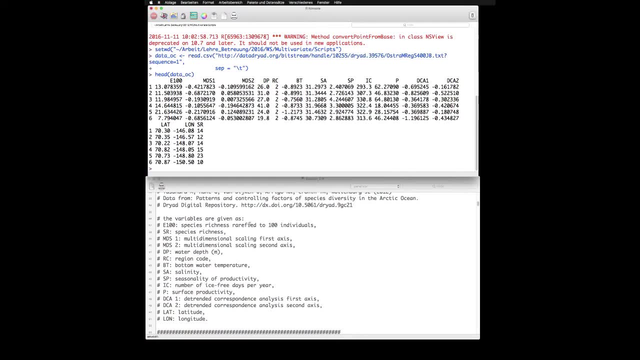 are all more or less numerically. The meaning of these variables is not discussed in detail in this course. I refer you to the paper to read about the different variables and their meaning. However, we should know that E100 is our response variable. 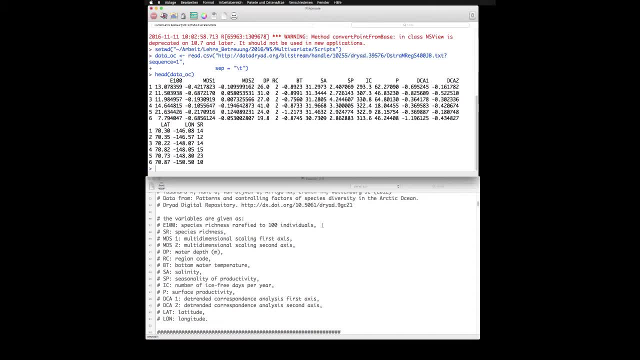 It's the species regions rarefied to 100 individuals. This means if you count 100 individuals, how many species will be in the response? This is the number of variables you find in a sample. We've also several variables, That's the MDS1, MDS2, DCA1 and DCA2 variables. 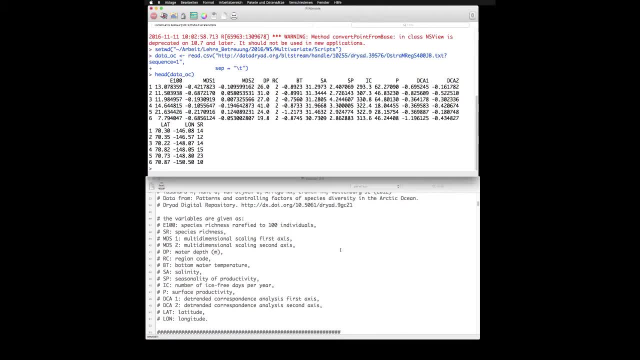 These are outputs of community analyzes And to predict an endpoint of the community, such as species richness, we can't use the community data itself, So authors use these as endpoints- The article for other analyzes. We won't do this here, so we'll remove these variables from the dataset in the first place. 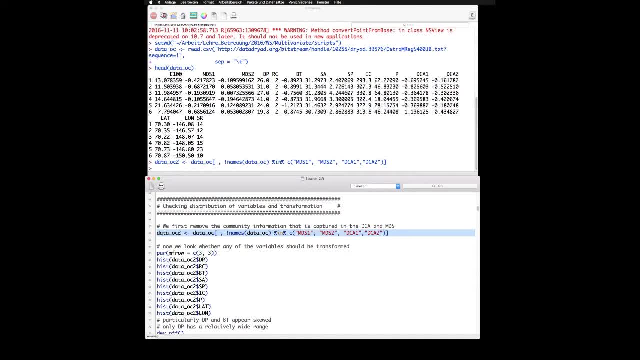 So we remove this. This is done. You see, here this looks a little bit complicated. The crucial aspect is that you have- and this is something that you certainly know- you have square brackets that you use for subsetting data of a dataframe or also of lists. 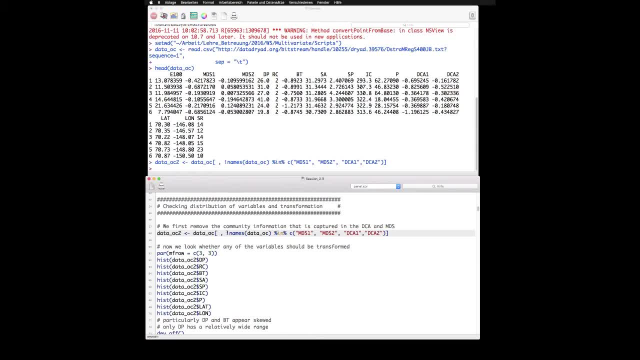 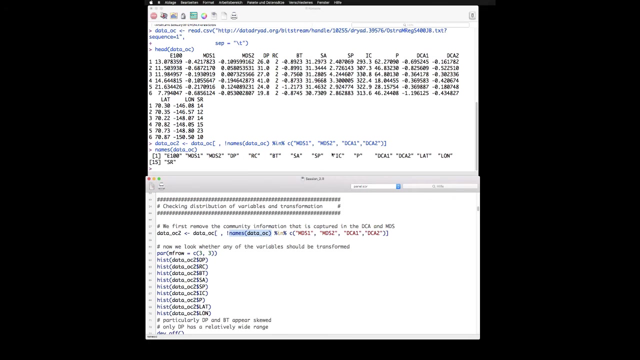 and or matrices, and here we have a function that tells our which columns should be used. crucial aspect is here this command and this tells our that every of the names that are found in the data, or sees or people- just execute this bit. let's see. this calls different columns in the data set: the names of the. 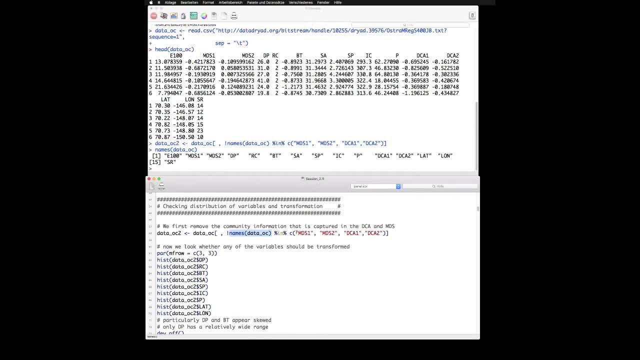 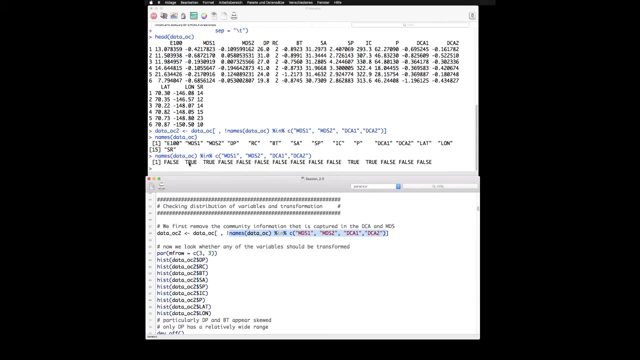 columns, to be precise, to identify those that equal mds1, mds2 and so on. so if you just execute this bit, we see we obtain a vector of false and true, so a logical vector, and with the exclamation point mark we produce the opposite of this vector. we reverse, we could create the. 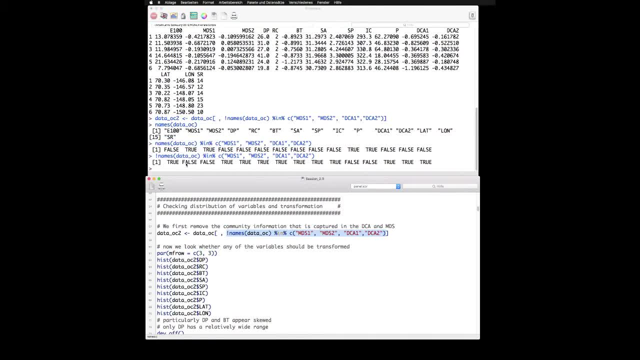 inverse of this vector. so false becomes true, true becomes false and this amazingly means that those information or those columns that have community information can be removed. because if you have column, if you have a logical vector provided for the different columns, true tells are to keep the column. 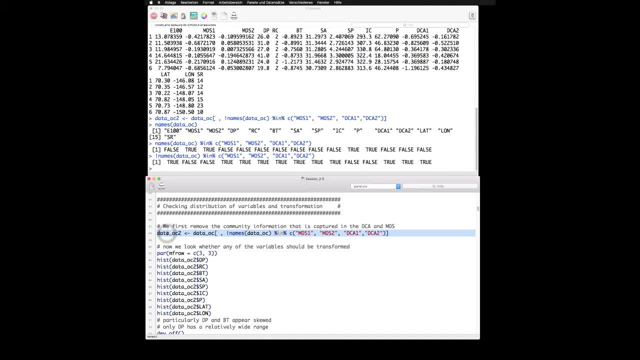 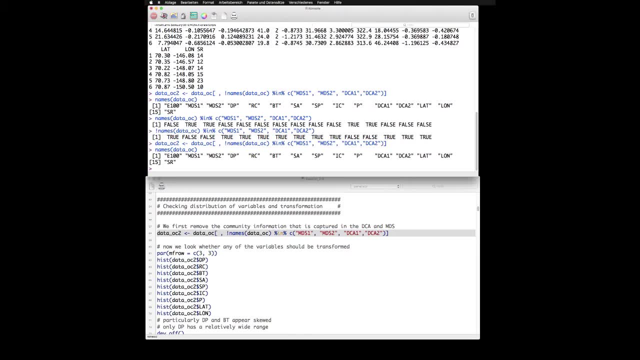 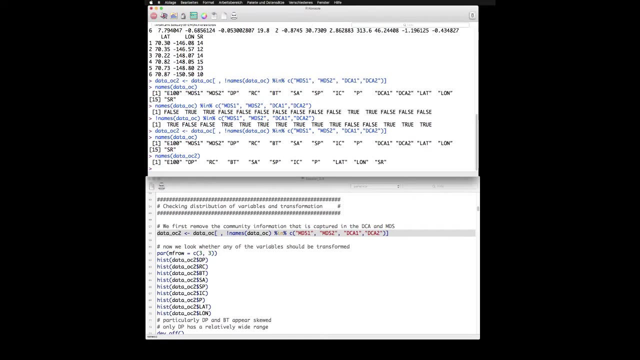 false means to remove that column from the data. so the executors- and have a look at the data set again- who we see that these columns have been removed now compared to the data. or see the head of the data set again and see that we were successful and removing the. 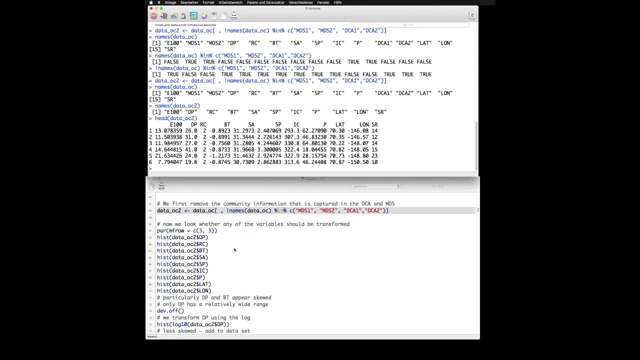 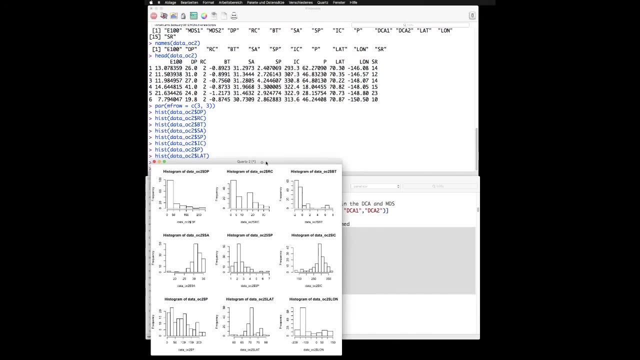 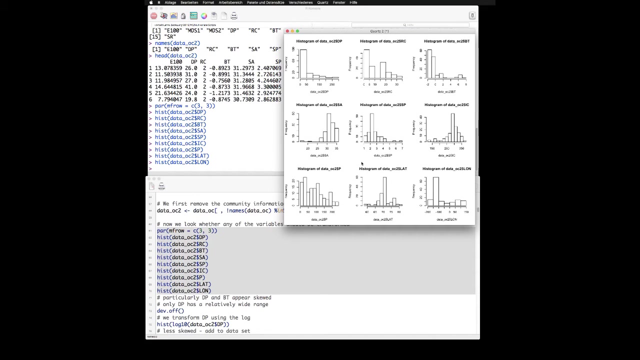 variables. now the question is, should we transform any of the variables before we run the multiple regression analysis? so we have a first. we have first look at the data and on the histograms what we see here is that particularly DP. so that's for the depth, and this variable is shown here, and the variable bt. they look fairly. 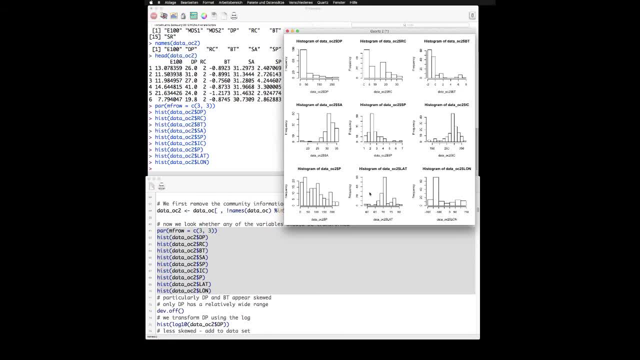 skewed. Of course, not all of the other data show perfect normal distributions. We don't really need a perfect normal distributions, but for data that has a wide range and that is very skewed- it's more it's- it's advantageous to transform the data before analysis, And this is 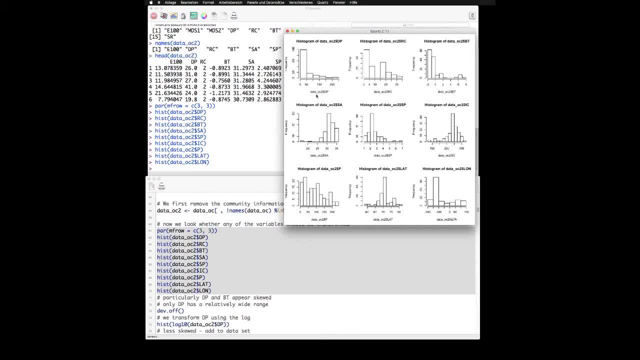 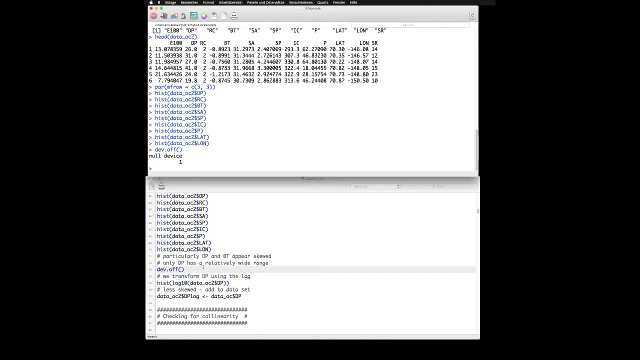 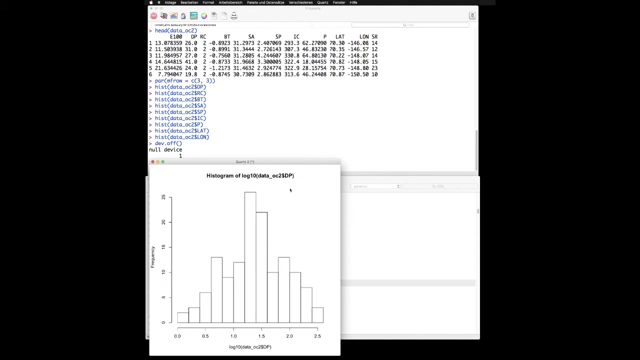 particularly the case here, for depth Depth has a range from, apparently, a few meters to 250 meters, so spans almost two orders of magnitude, while bt as a relatively narrow range of data. So we transform depth, and that's actually what the authors of the original study did as well. We look at the data. 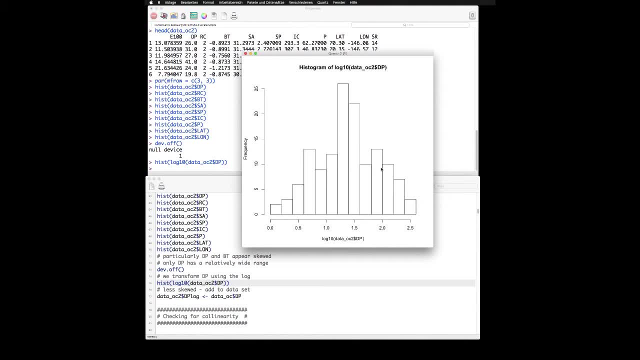 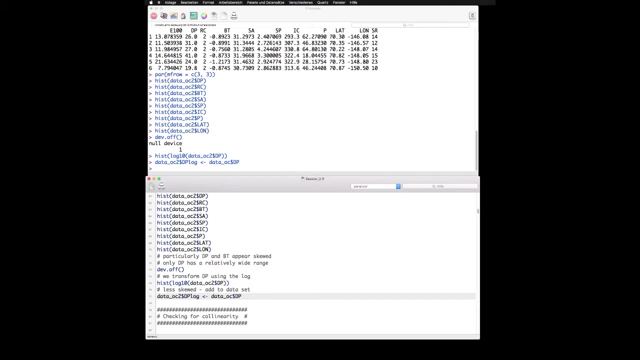 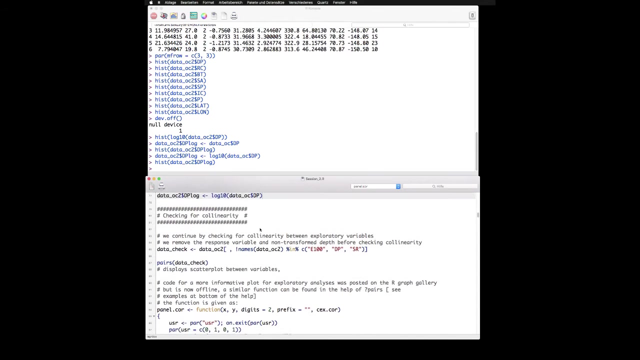 again and we see that now we have removed the skewness of the distribution, have a fairly normal distribution of the data. So we add this to the data set. After we have added the variable, we move on to check for collinearity- Collinearity. 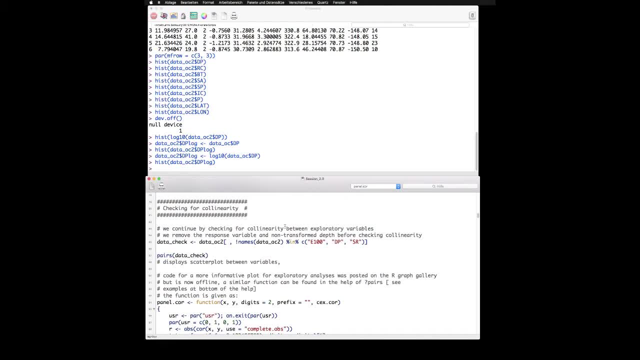 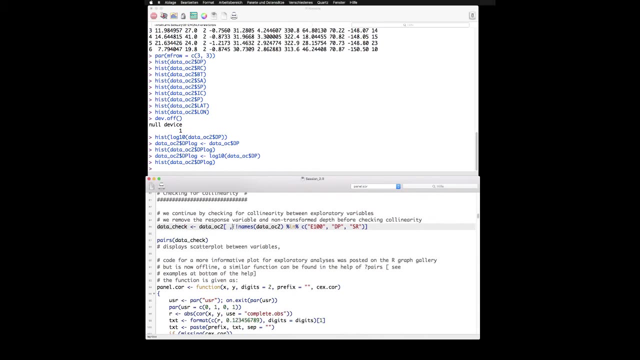 means that we look for a variable that has a wide range of variables and that is very glue In the given tray. here we have the contribution of in different analyses and than for the proportion of variables we use base ading variance. that gives us the endlessly stream of data that we argue. 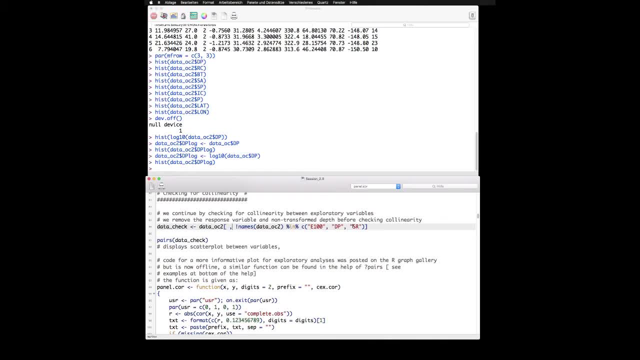 with. We also remove theOSwd variables, which areary class variables. We explain one t and provided that it is a variable that only seduces in the space of 10.5W, it's not actually a variable but a real variable. We consider only it. We lightly replace that number. 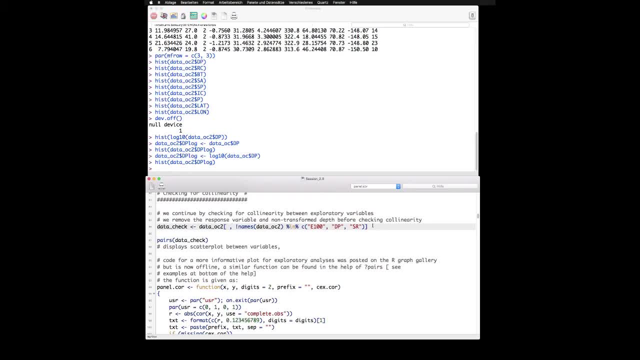 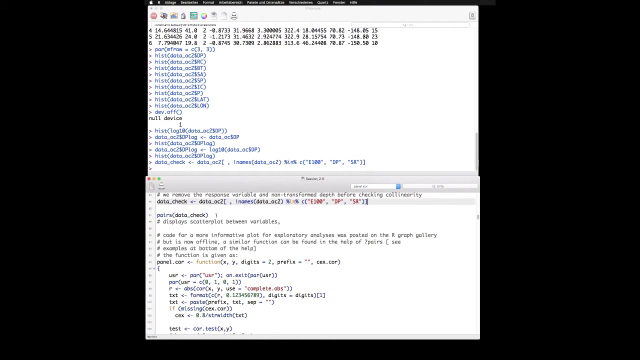 and we have the shifts In the species regions. we won't use for explaining an explanation, so we remove all these variables and we do this using the same function as before. I have explained that with searching for the names of data or C, we can remove these columns, A function that is very handy to look at. 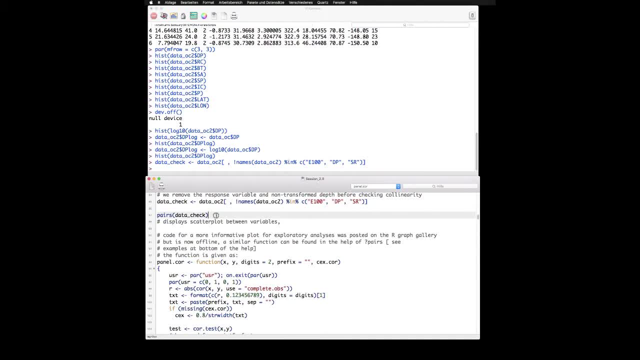 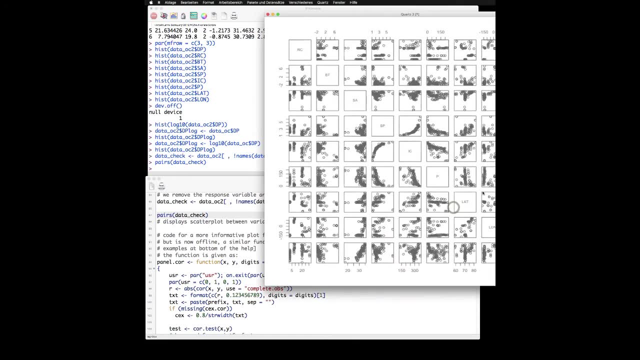 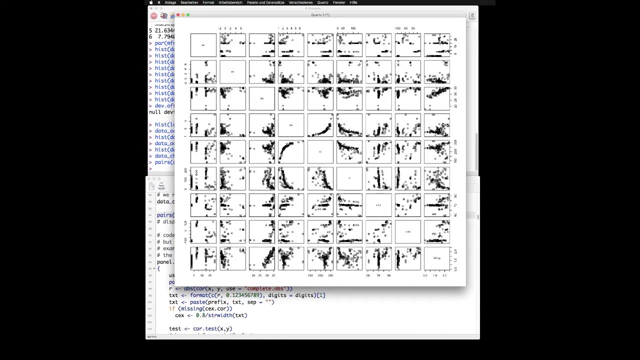 b-variant relationships between explanatory variables, between predictors, is the pairs function. So here we can see the relationship between variables and we see that for some of the variables in C we see a relatively close relationship, for example between IC and P, between IC and SP. 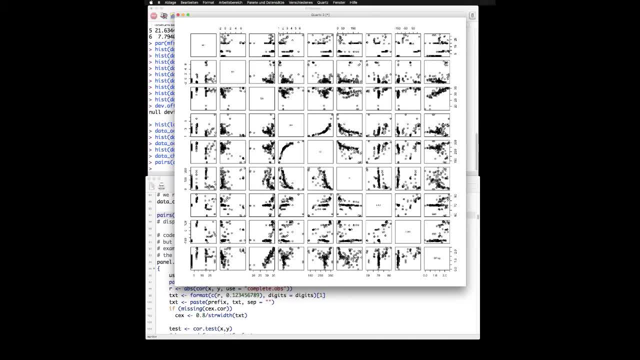 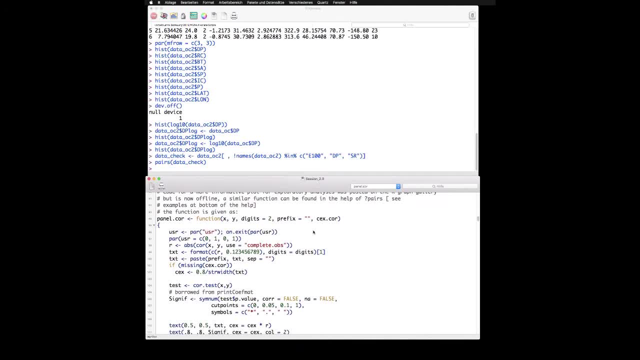 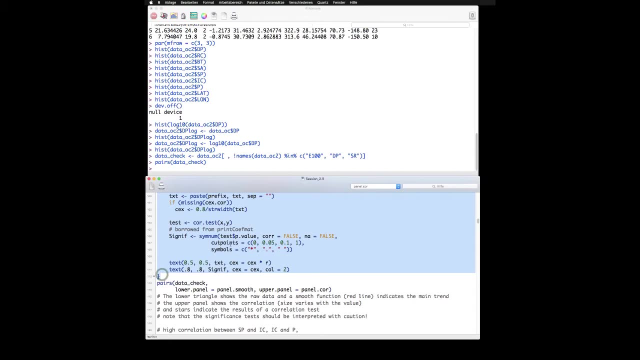 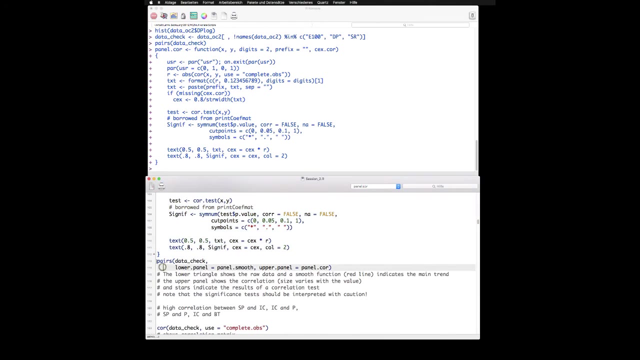 Although these are curved relationships, we see that there is a clear pattern. The plot is not particularly nice. we can obtain a little bit nicer plot if we execute this part of the code. I won't go into details here. this basically creates paired scatter plots that have different information in the upper 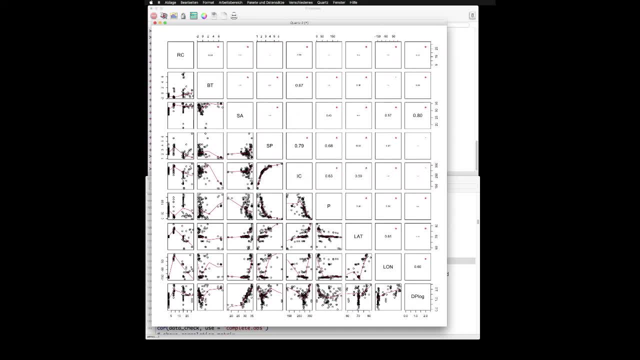 and lower triangle of the plot. So what we see here, we see below the relationship with a smoothing line and we see here the hypothesis test on relationships, the correlation coefficient, along with a star for statistical significance. The larger the number that is displayed means, the higher the correlation. What we see is that, indeed, IC and P are very similar. The 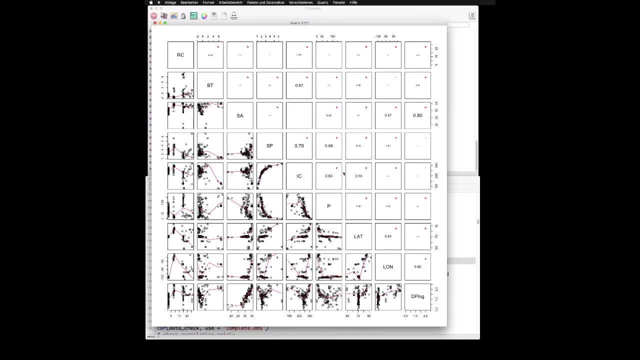 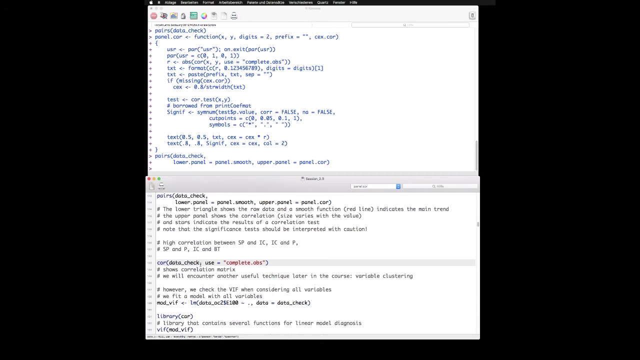 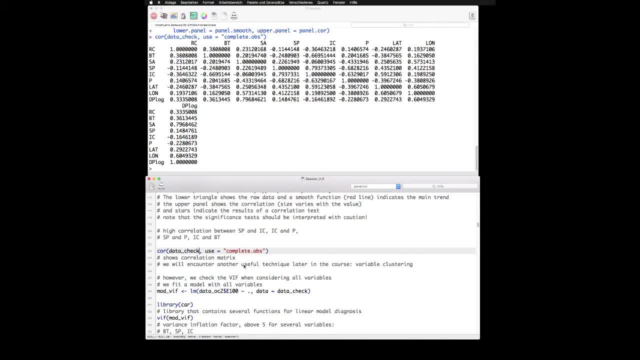 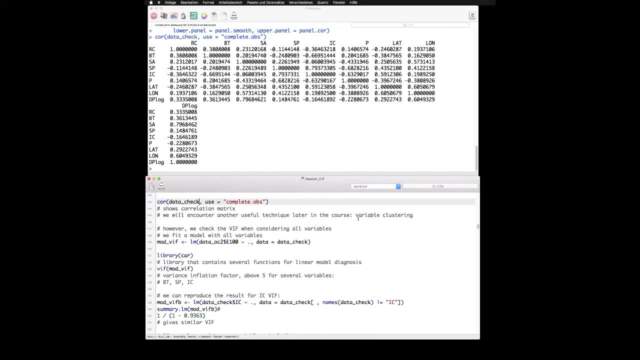 is extremely close for the purpose of demonstration and we check the variance inflation factor. Later in the course we will also demonstrate how to use another technique, variable clustering, and this is done later when we discuss cluster analysis If we want to check the variance inflation factor for details on 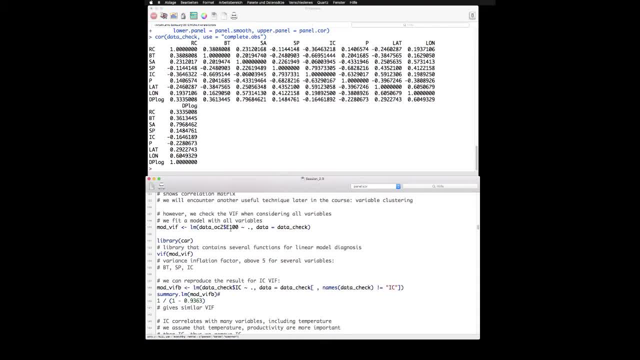 this factor. I refer you to the lecture slides. Then we first have to fit a model with all variables. So this is basically the start model, a linear model. You've already fitted a linear model for two variables, so one explanatory and one response variable. What we do here is we create this model for 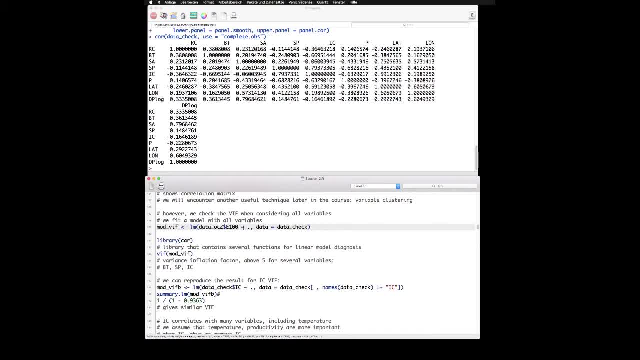 multiple explanatory variables. The nice thing in R is here that we don't need to enter individually each of this variable in the formula, but we can just enter a point, and this point is a placeholder for all variables that are contained in the data set data frame. 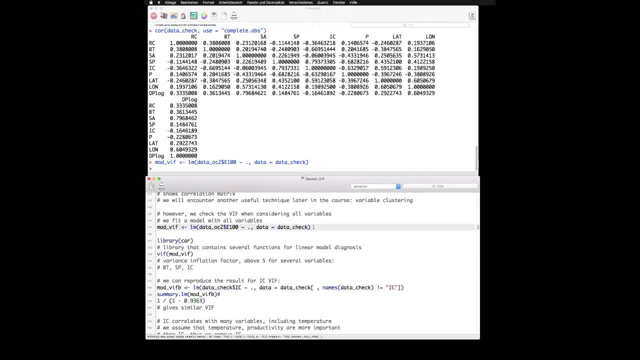 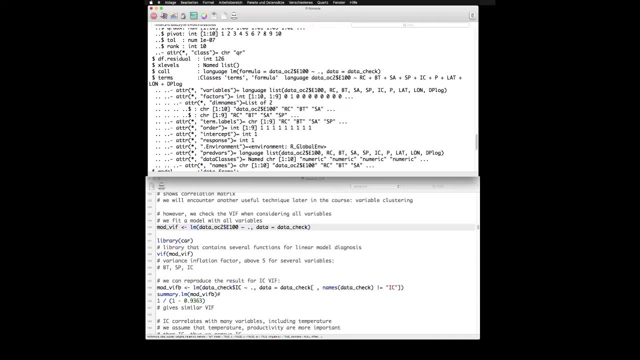 data check. We execute this. Let's have a look at this object, a long list. We see that there's a formula of the terms. They are displayed here. We see the E100, so the verified species richness as explained by RC, BT, SA, SPI and so on for all the individual variables, and we 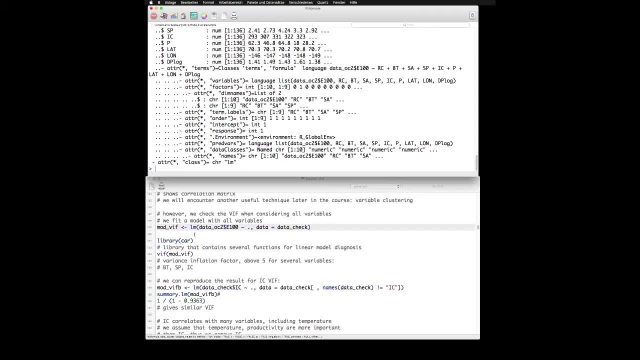 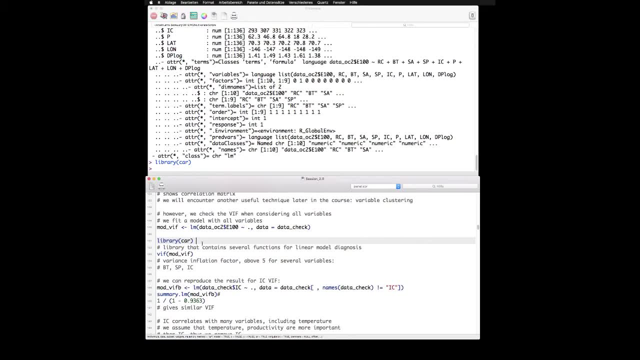 don't need to bother entering data. We load the library car. This library can be used to calculate the variance inflation factor and this is done with the function with bracket open, then the model object where you want to calculate the variance inflation factor for bracket close. We obtain here: 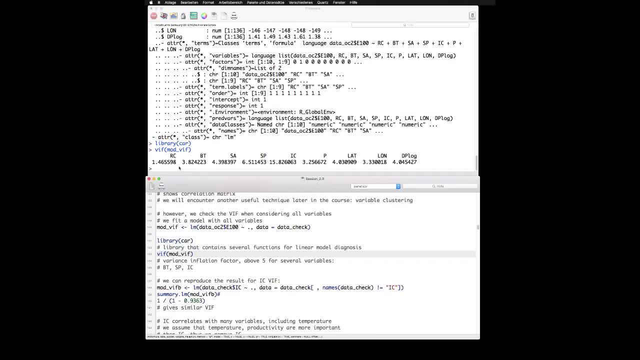 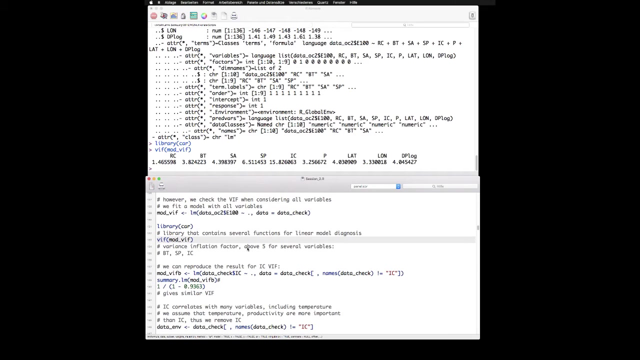 the result results for this computation. What we clearly see is that IC has the highest variance inflation factor. It means that it's most explained by other variables. It has the highest R-square when explained by other variables. There are rules of thumb when the variance inflation. 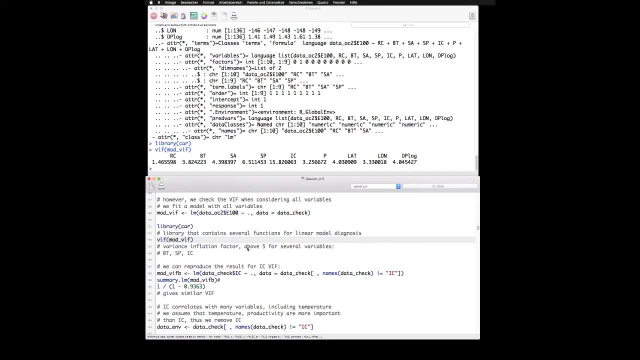 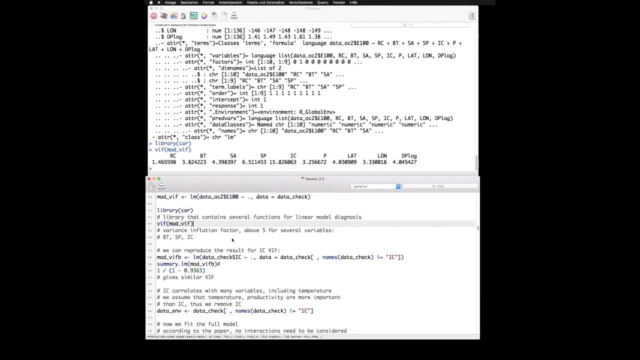 creates a problem. The rule of thumb is factor 4 or 5.. We see that, basically, IC is the only variable that strongly exceeds this threshold, whereas SP, SA and other variables are just above this threshold. The first thing we do is we remove the IC variable from the data. 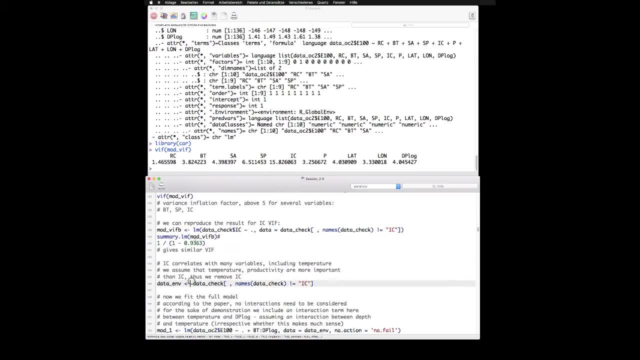 set. That's done in this line. Here we introduce an Asian model to show you how to reproduce the result for the variance inflation factor for IC. So let's say we fill in the assessed variable with a model for IC, explaining IC by all variables except for IC, This you should. 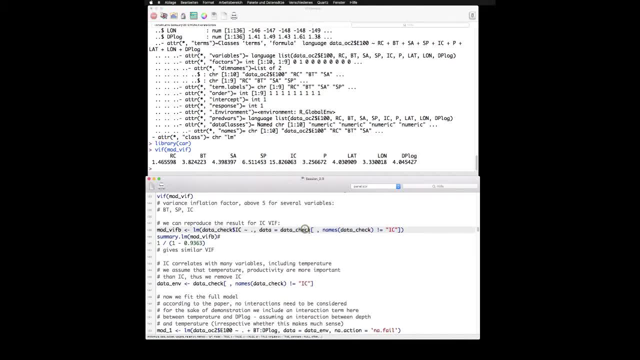 be able to read by now. We click on the subject part again and select the subset. The 18 validation leave-in variables that we have proposed現在 eris the result of the asset class data check to columns, and the columns that you remove is IC. So we create a. 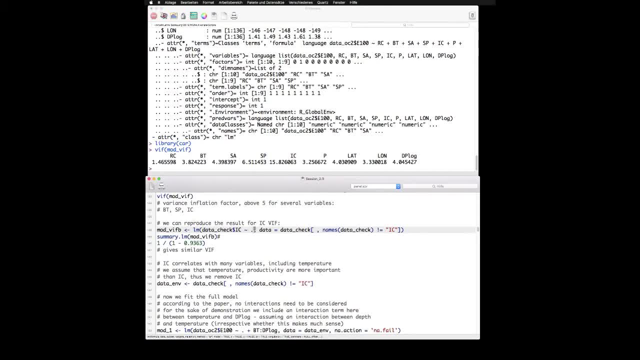 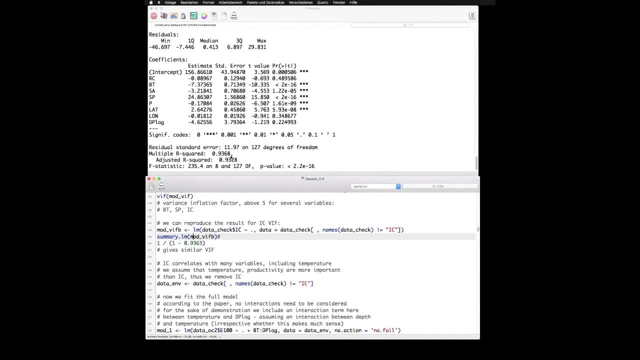 linear model again, where we try to explain IC by all other variables, We see that 94 percent of the- even for the adjusted R squared- about 93 percent of all variation in the IC variable- is explained by the other variable. So most of the information is somehow captured and the variance inflation factor is. 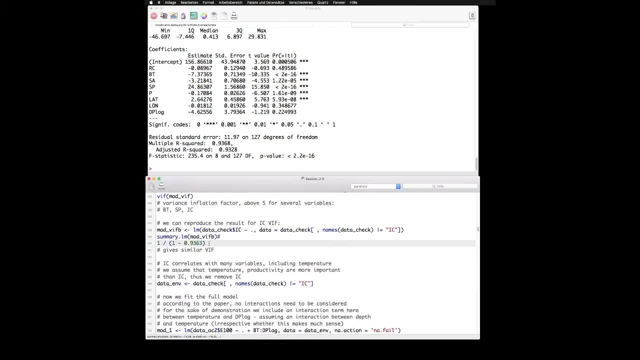 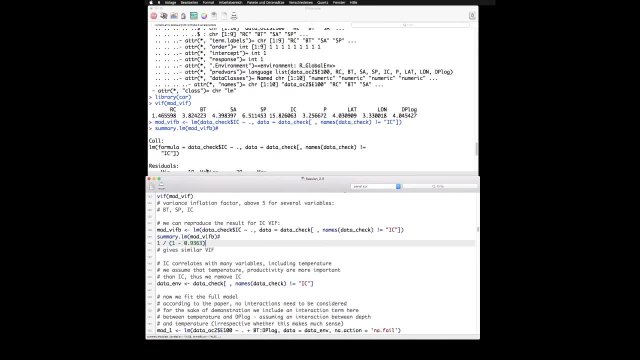 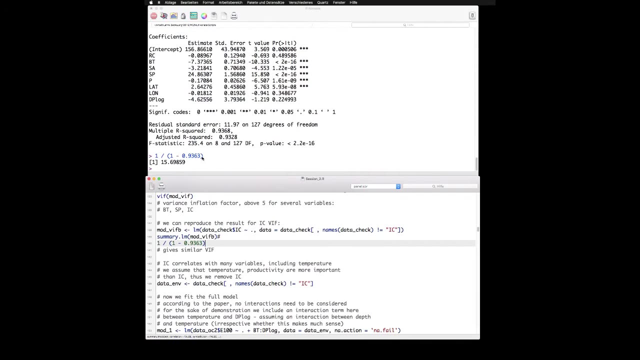 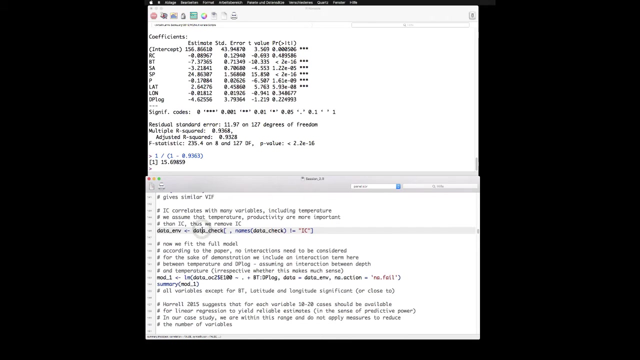 calculated by 1 divided by 1 minus R squared, and it shows you that the result is 15.7.. That's the same result, more or less, as we have been provided by the function here. Ok, we remove this variable and we keep all the other variables We could. 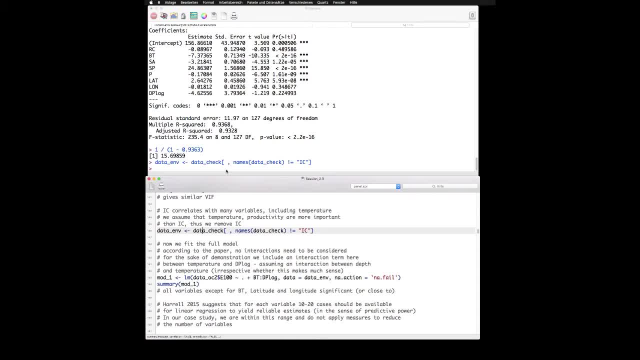 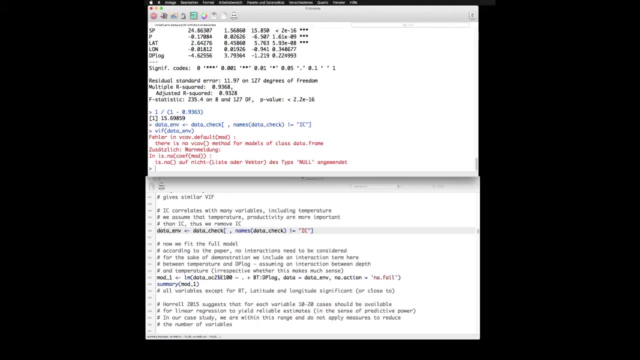 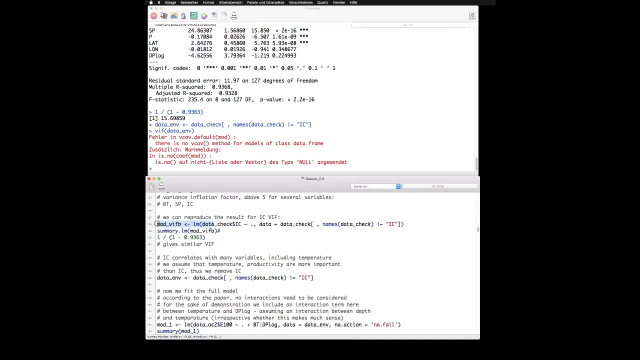 recalculate the variance inflation factor again, for example by typing with data and the new data set. This actually fails, because this is just a data frame. of course, We would need to fit again the model like that. So let's do this Just for the purpose of showing you how it works. 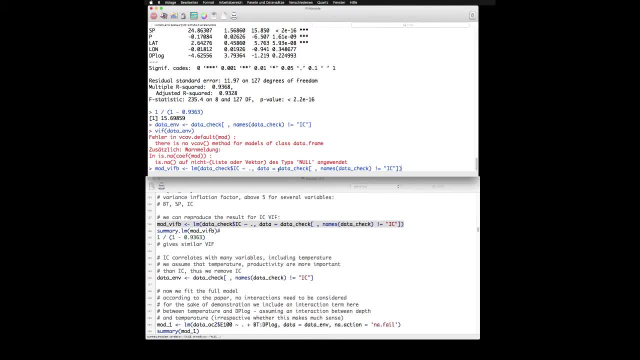 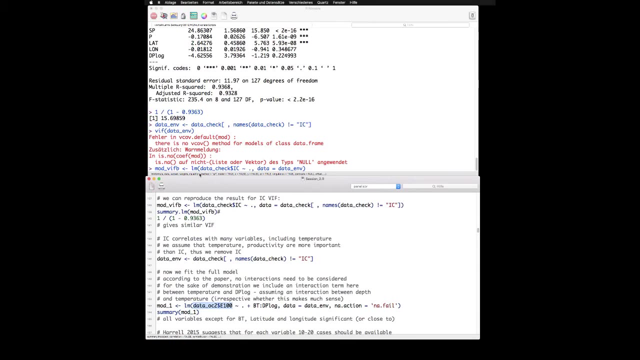 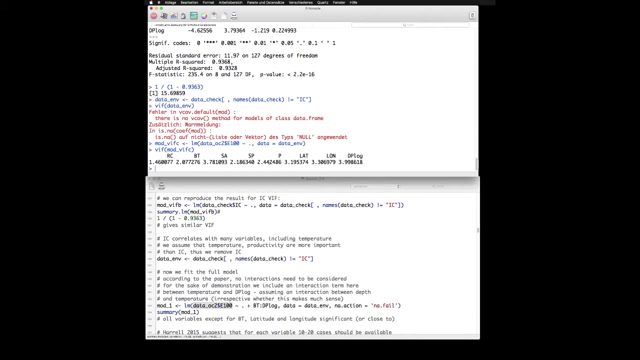 Just for the purpose of demonstration. So we use the data in V and we again we explain: graph right: species richness. Now we execute the variance inflation factor For this model again and what we see is that by removing IC from data set we have got rid of the problem of collinearity, more or less. So there still. 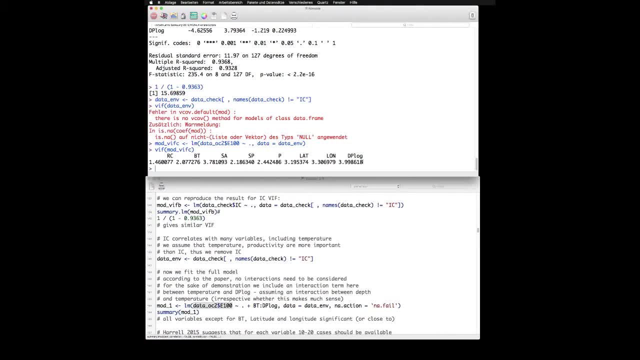 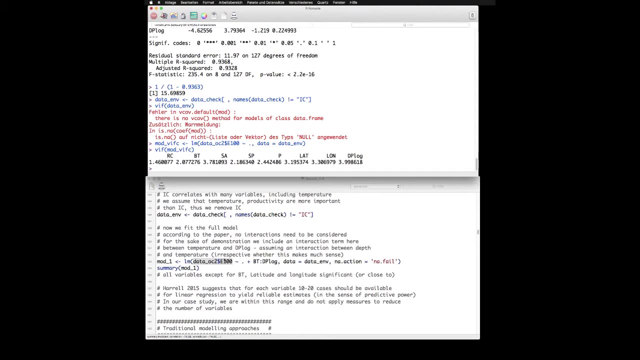 a couple of variables, like SA or logarithmic depth that are relatively close to this variance inflation threshold provided in the literature. But we don't bother about this here and I think, unless you have several variables where this is the case, that they are close to this variance inflation threshold, we shouldn't. 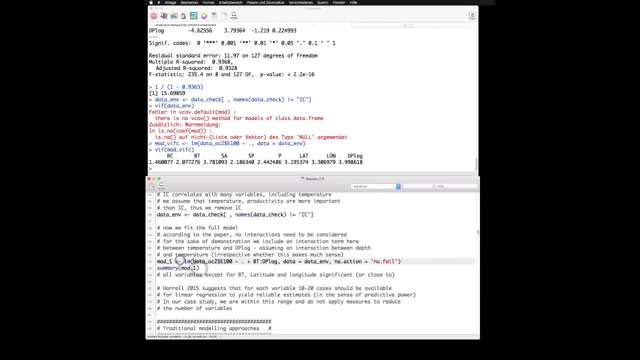 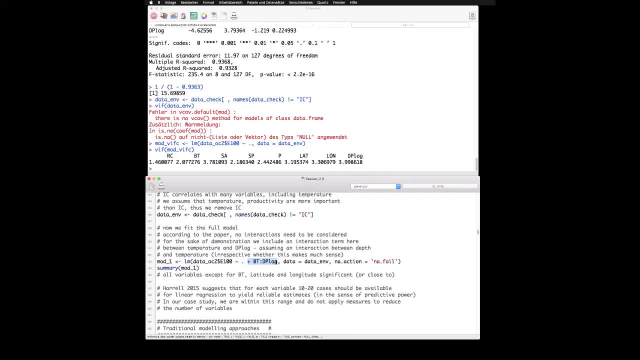 So we account for the possibility that at low levels, that the effect of one variable or that the level of one variable affects the outcome for another variable. Let's say you have a high and low depth, that at low depth the temperature effect is much higher than at low depth. 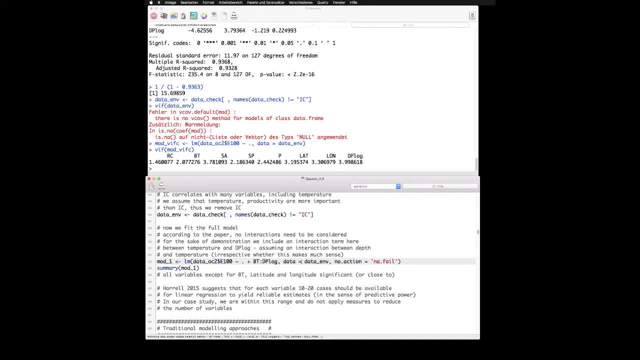 at high depth. So this is such an assumption- as no scientific basis or something of which I make this This is just for illustration purpose- that an interaction effect could be present and how to implement such an interaction effect in the linear model. What you see here is the interaction. 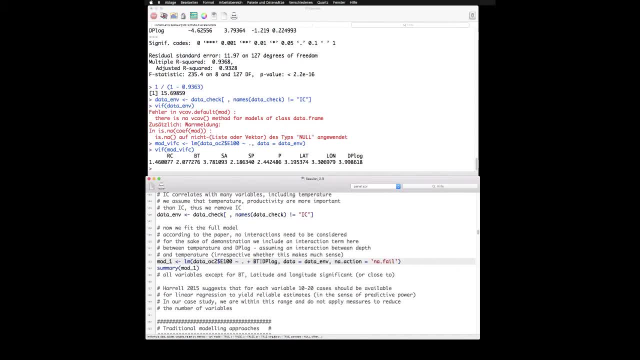 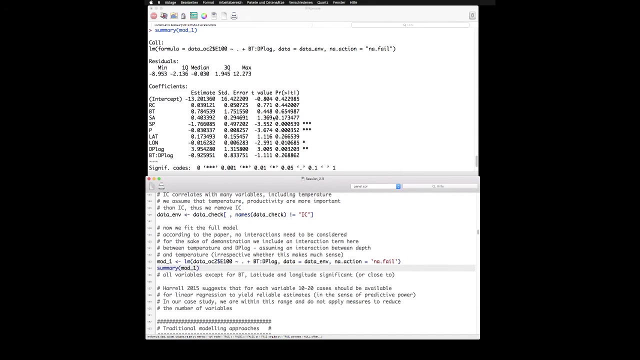 effect is included by the variable. Then you have two points and then you have the logarithmic depth. Run this model and we see in the summary of this object: In the summary we see the call, which function has been called, we see the residuals or the median of the residuals. 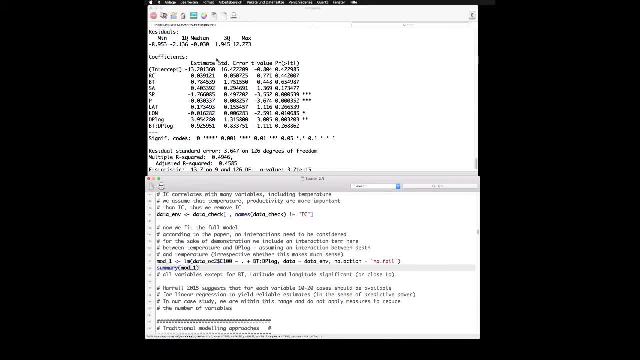 So is explained by the deviation from the ordinary, at least cl Ev suite, Where we obtain the co-efficient for the different parts of this model, for the different variables that are included in the model. On the one hand, we have the estimates for the different variables, as well as for the intercept, and you obtain the standard error. 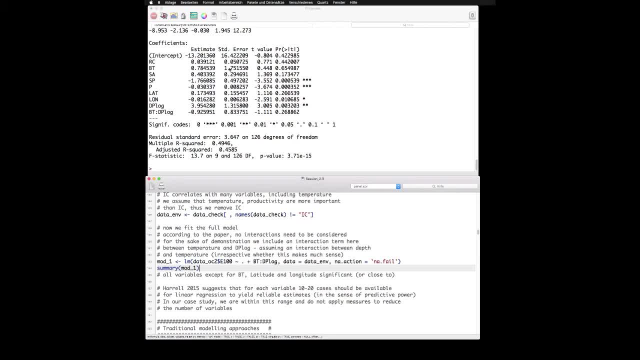 The higher the standard error, for example, for v-t. this means that it is unlikely. DAN and HV: It is on the probability of multiplication error. However, here you obtain theisk, the higher data body of it, the higher the standard error, for example, for v-t. this means that it is unlikely, that it is unusual that we automatically have Rs. 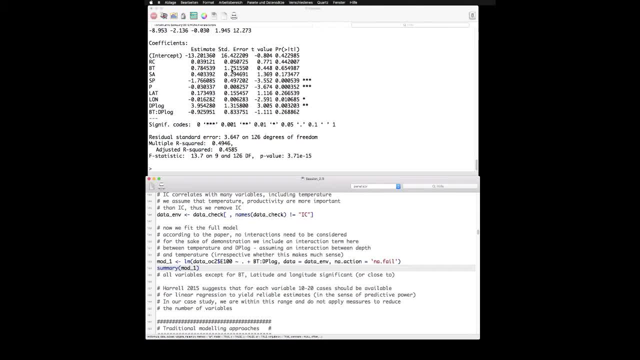 And here we have a 1986 value, the general error of Rs. and because the likelihood of the弧ial deviation is, to the least ordinary, it's higher than the standard error- the less certain this coefficient is, and we see this expressed in the p-value related to this, to this coefficient, if 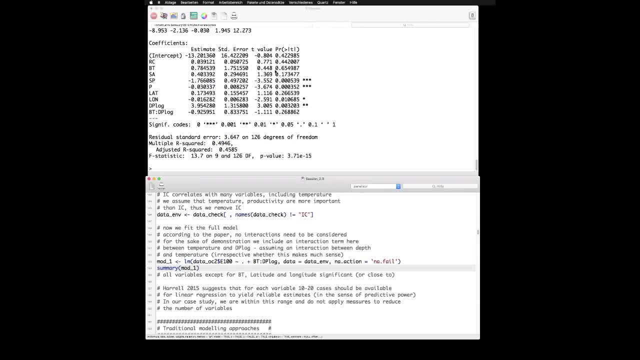 the standard error is larger than the coefficient itself. that means that we have a variation that is so strong that the zero, that the variable coefficient could always be zero as well. and that is the test that is tested here with the t-value and then the p-value: whether the regression coefficient for a 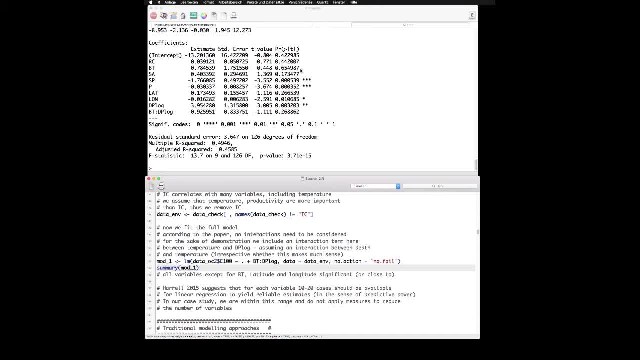 variable is significantly different from zero. this is not the case in this type of model of the variables, as well as for the interaction term. well, we know that such a model, this is the full model. now, now for this model, we would be able to interpret the coefficients. that's what herald suggests, that only for the full. 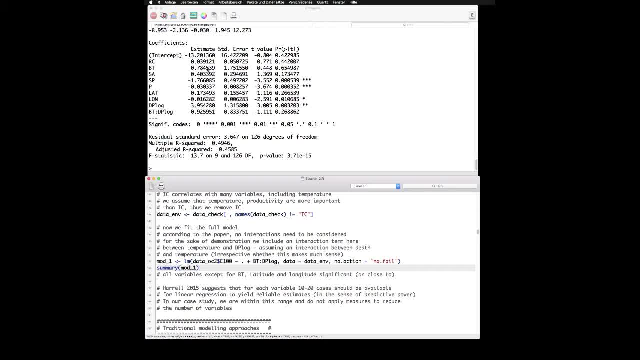 model, we get what we get, obtain precise coefficients. but if we now remove variables from this model and have sequential testing, then what happens is, if we want to separate, like how much polar value we'll get from two 1 for 0, we obtain some bias, We obtain too low confidence intervals or standard errors. 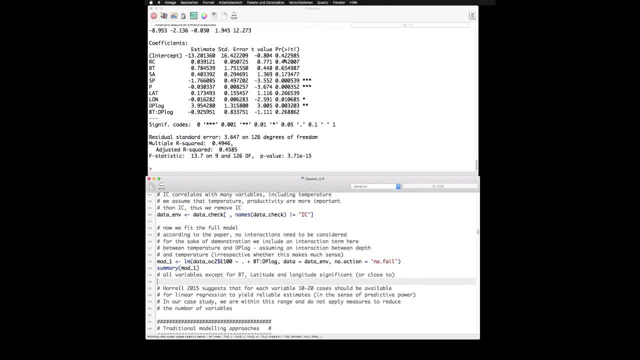 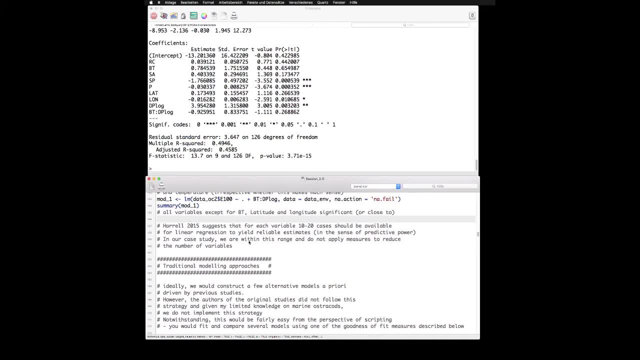 and the p-values cannot be are biased low. So generally we should have about 20, 10 to 20 variables per observation that we include in the model. We check this here. in our case. we ask how many rows this data set has. We see this: 100,. 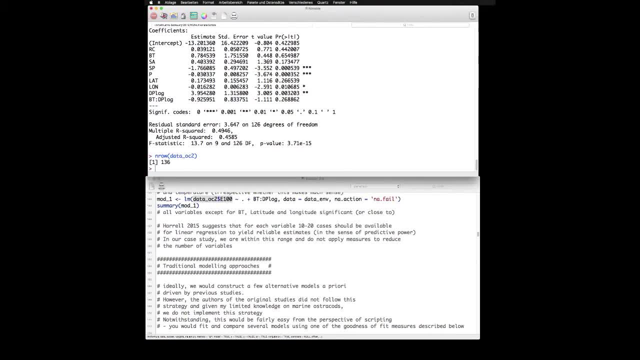 but 110, observations 135. we need a couple of degrees of freedom to estimate the intercept so that the others other aspects of the model. So we have about 130 degrees of freedom left for the parameters. if we now say we have here 1, 2, 3, 4, 5, 6, 7, 8, 9, 10, so we 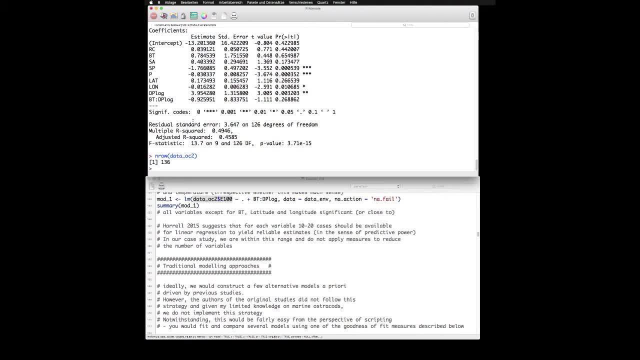 have about 13 degrees of freedom per variable. that's within the range where you can fit a linear regression model with reliable estimates. doesn't mean that you can't fit it if you have a lower amount of data. but i discussed what you need to take care of in the lecture. we won't go. 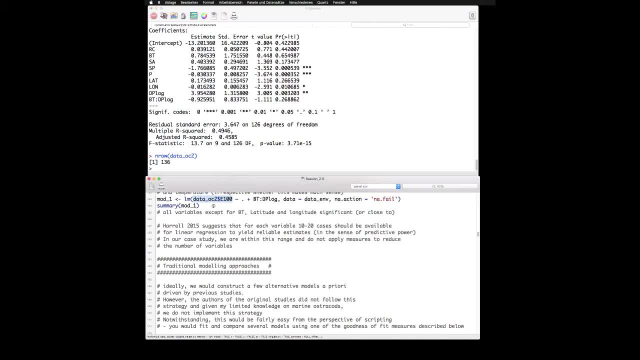 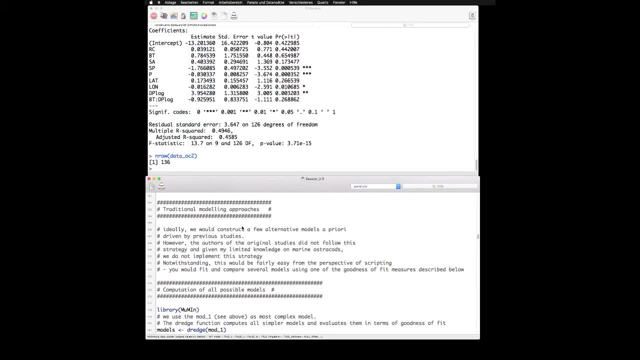 into details here. the traditional modeling approach would be, or the traditional approach as we first discuss. one of the approaches is that you just construct a few alternative models, you choose the goodness of fit measure and then you compare these different items- alternative models. however, i'm not a expert on marine ostracodes and the original study authors. 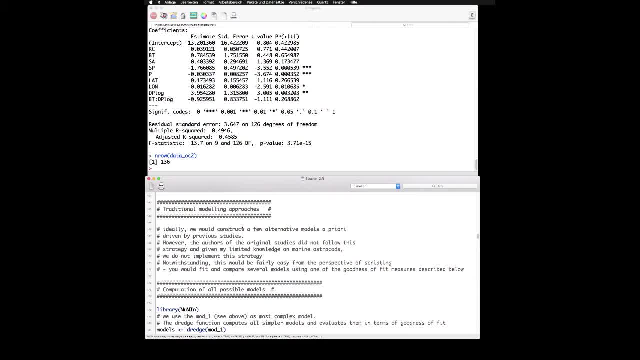 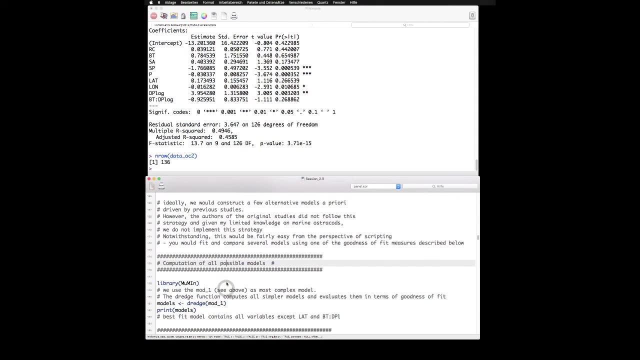 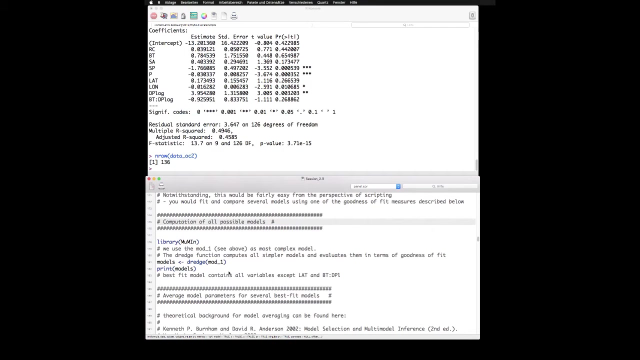 also did not do this, but they used a modeling strategy and that's why they used- they use- stepwise regression modeling. however, we are not starting with that here. what we are doing first is we compare all possible models and again, i won't go into all theoretical problems of this approach, i just show you how to do this. 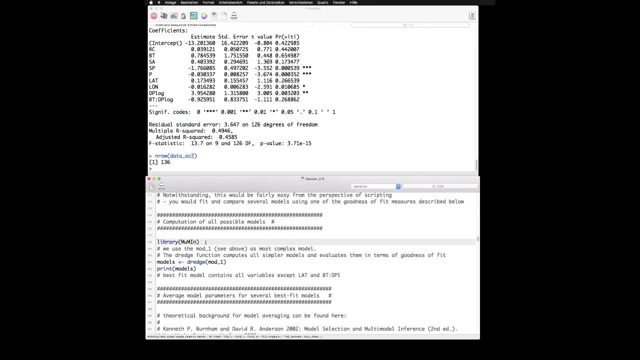 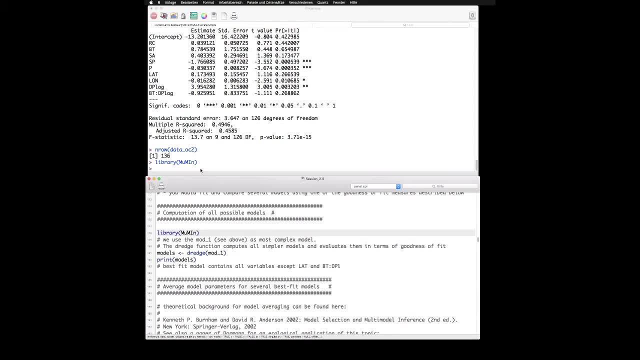 please recruit or refer to the lecture slides to know more about the appropriate appropriateness of this approach. so for multi-model interference we use this library moomin and to calculate all possible models. so that's the type of ours we just determine here. so we will use this map and this one. multimon Jamie, we need a table. it's there. we will take soil. that it's going to connect a frequency parameter to T on a one- county basis and then, by that way, a map. every branch of the system will be taking a cousin two. so, like every agency, every charge will take four points, a third and an elite퍼centage pork. so all these settings will be separate and the 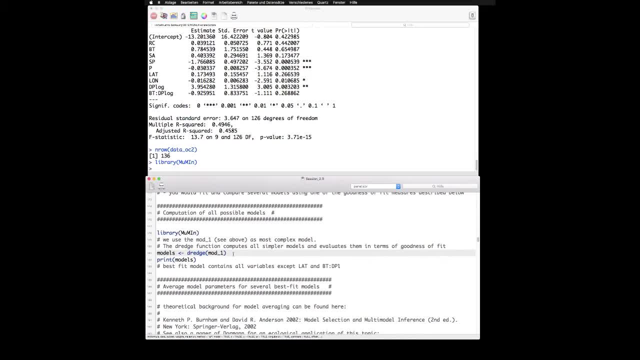 that means you calculate all models where you have just one variable included, or combinations of two, and so on and so on. that's it. that's heaps of models, as you can already see. so this is easily done by the drag function. we just enter your model and then we print the model. what we have here is we. 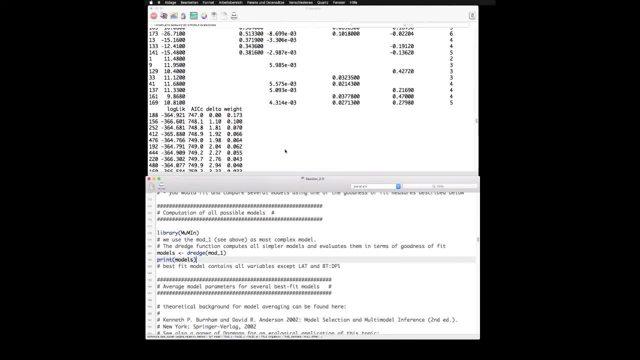 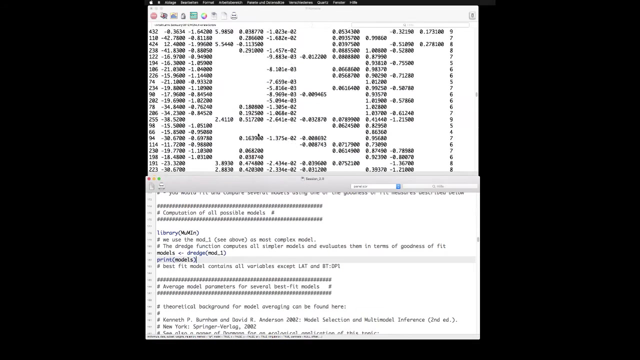 have different models, get a whole lot of output. for all the models we have to look likelihood, the corrected AIC, the Delta, IRC, so the difference and the corrected other C and the weight this model would obtain if we would use all of the models based on the AIC, on the corrected, I see to be precise. 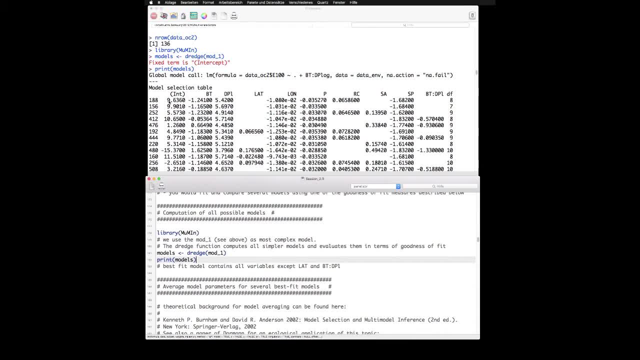 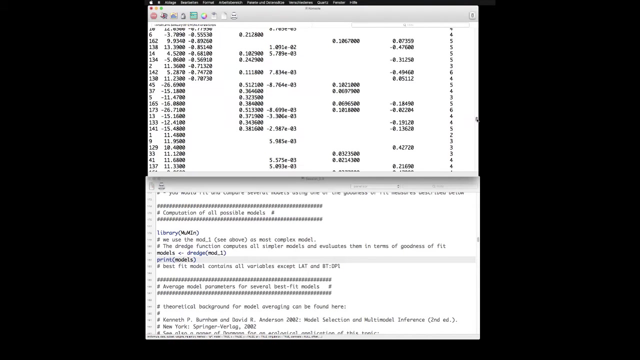 so in the next step we see that in the model selection table latitude has been removed, was not included in models with a IC. same holds for SA and in addition for the interaction term, BT, DPL, the AIC. again, The AIC of these models is pretty close. There's a rule of thumb. 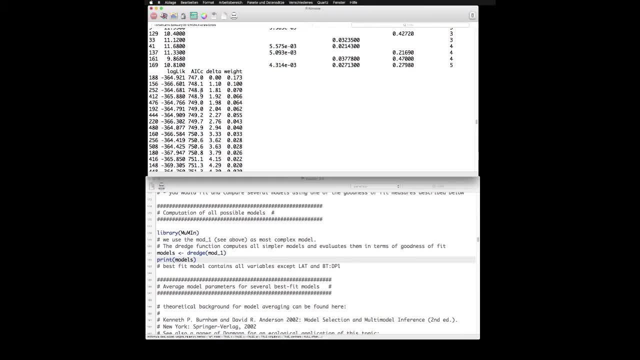 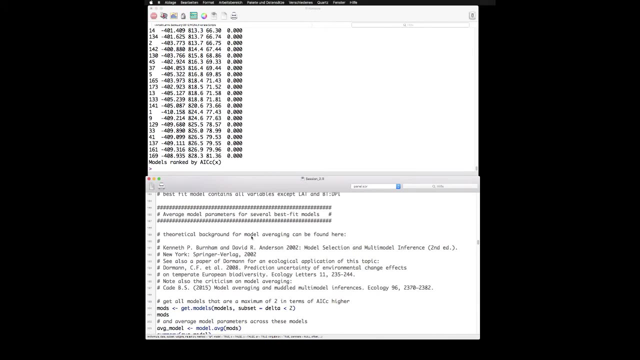 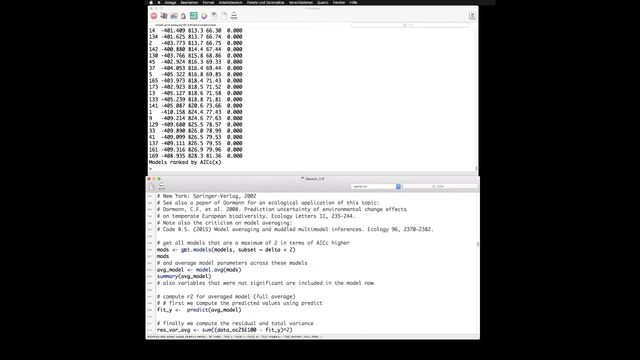 again, There are problems to this rule of thumb, but the rule of thumb says well, within an AIC of two, these models should be considered. We do not just consider the best fit model, but we would follow a strategy to average the model and not going into details here. Then we could do this using this rule of thumb. that 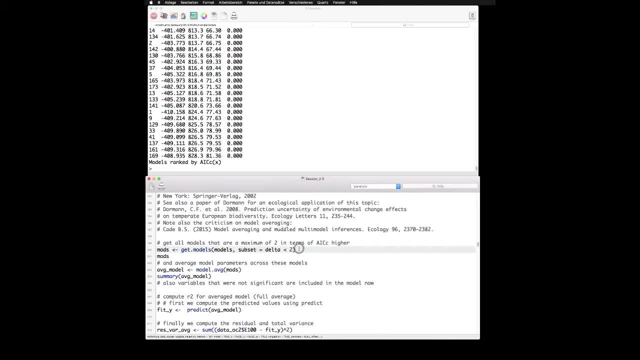 within the delta of two. these models can be used. Use the function getModels. that identifies all models that are a delta corrected AIC within the value of two. maximum difference of two to the best fit model. These models are selected. Call this. We see here the different types of models. It's one, two. 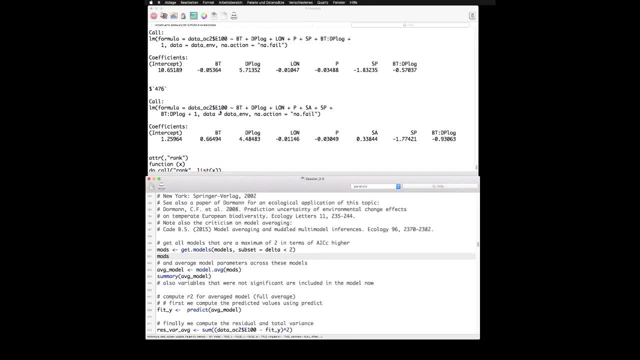 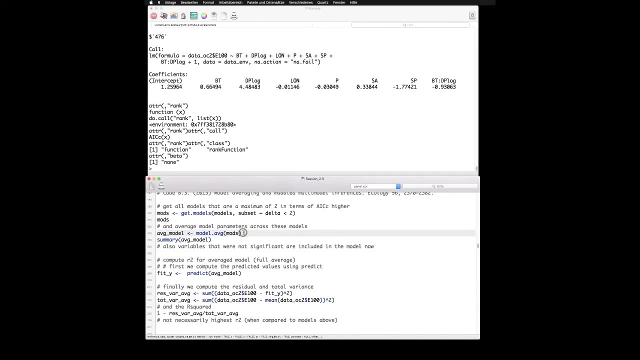 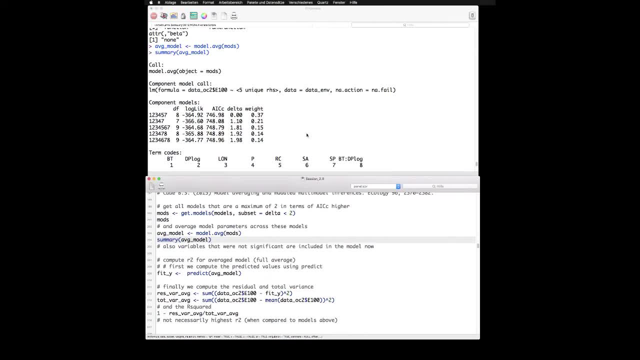 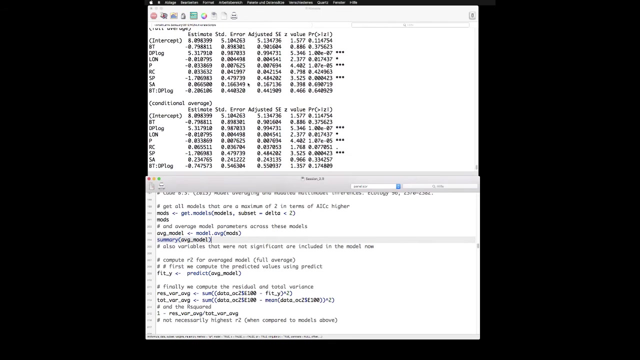 that we have here an averaged model from five different models and we see which variables have been included in the different component models that were used for the model averaging. We see the coefficients of the model, average coefficient. So that's the full average, where every model has the same weight, and we see the conditional average if every model has the weight as defined by the different component models. 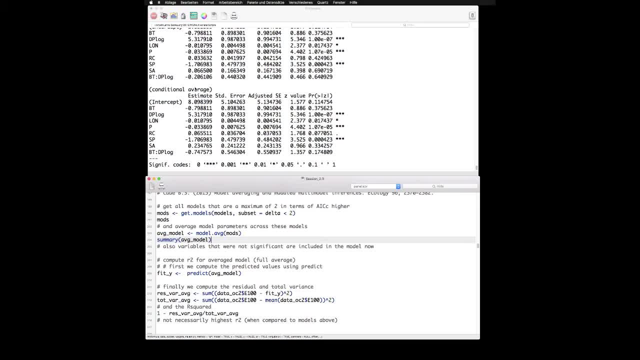 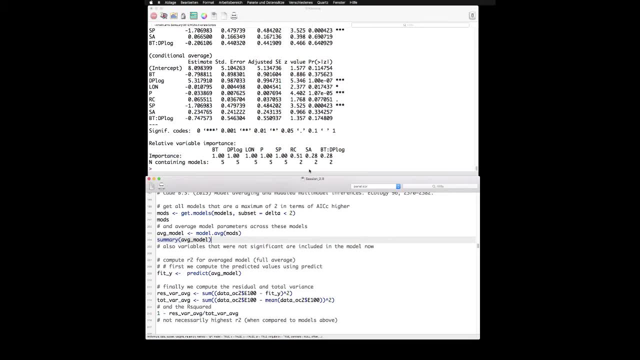 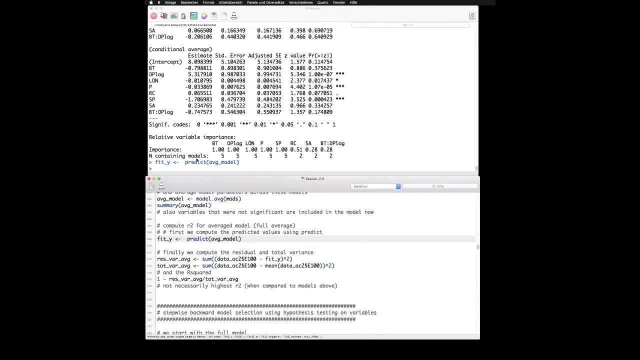 We see this only varies, for example, for SA and for the interceptor. Yeah, so far. we could now use this aggregated model, this average model, and check the fit of this, the R squared of this model. We do this with the predict function, So we have obtained the fitted model, fitted values. 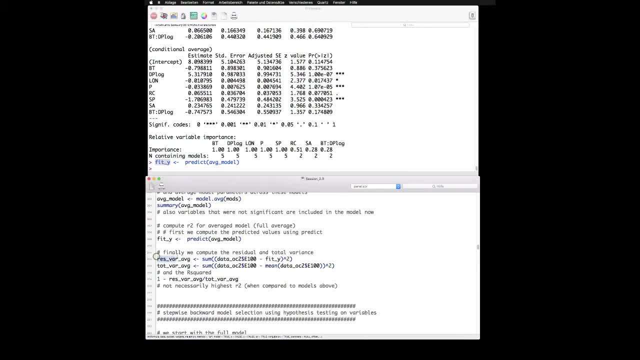 And we can calculate the residual and the total deviance for this model. We do this with the sum, So we sum up the squares between the observed rarefied species richness and the predicted species richness, and we take the sum of squares, And the same thing as we do for the total variance. 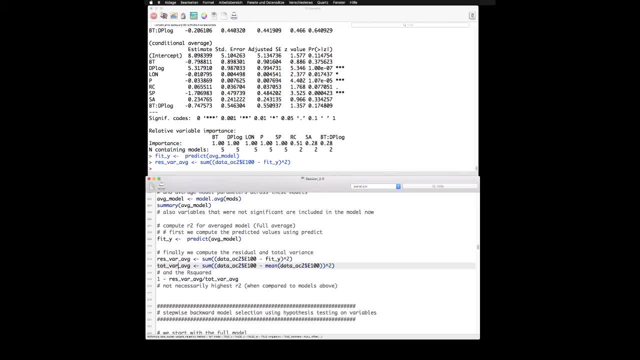 calculate the species richness and subtract the mean of the species richness squared. What we then obtain and what we see, is that we have about 50% of the variance explained. so the R-square is 0.486.. If you compare this R-square to the models above, 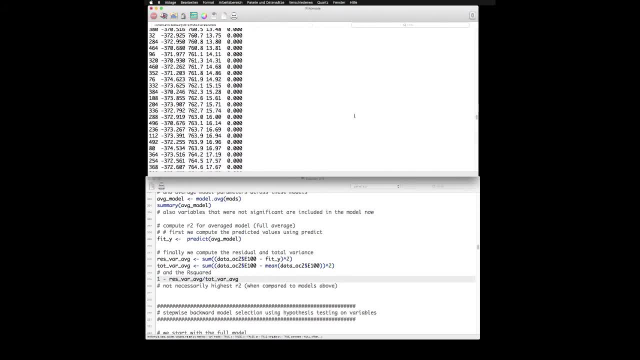 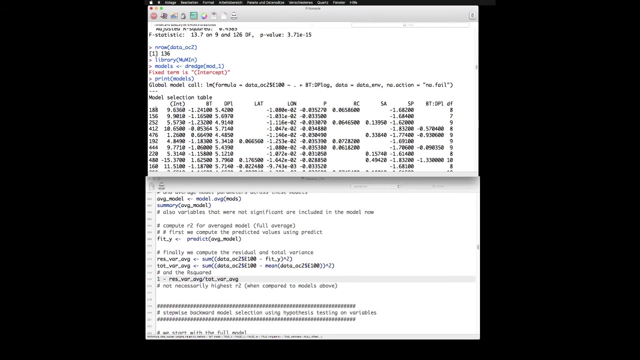 Let's look at the individual models. This is not necessarily the highest R-square. For example, we had here slightly higher R-square each point for this individual model that contained multiple variables. when we would fit this selected model here with the highest AIC, This might also have a. 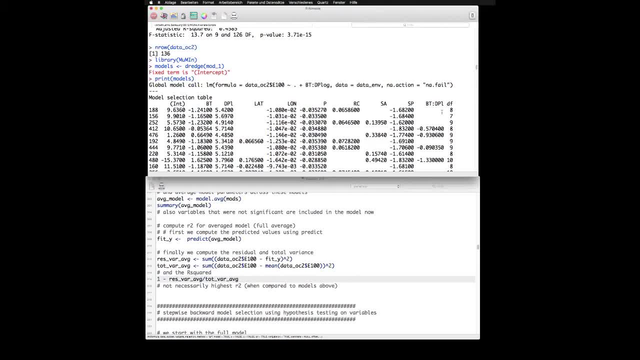 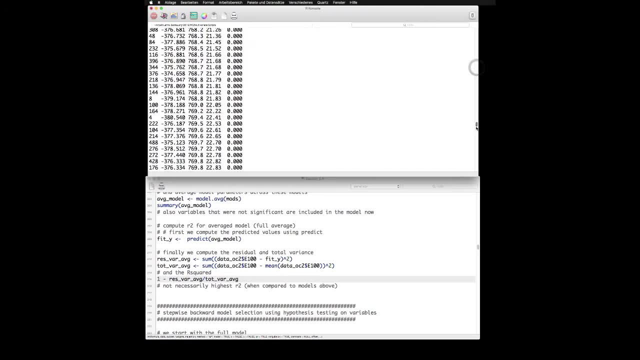 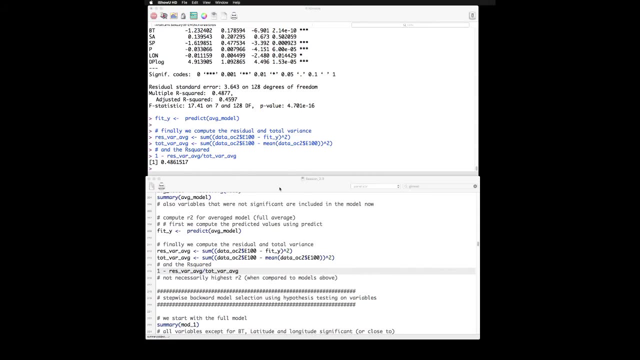 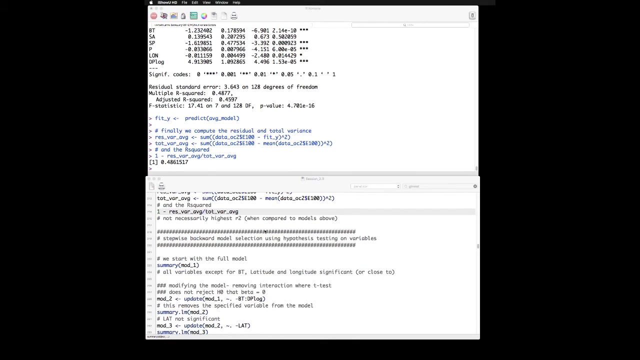 different R-squared. Keep in mind that the R-squared, of course, inflates for every additional variable that is included in the model, so this is not too surprising. The next technique we will look at is stepwise backward model selection using hypothesis testing on variables, and we've already discussed 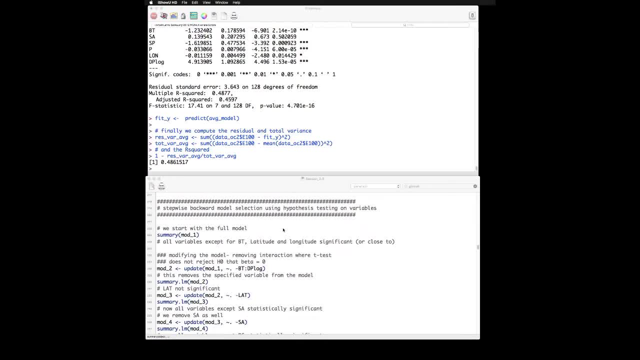 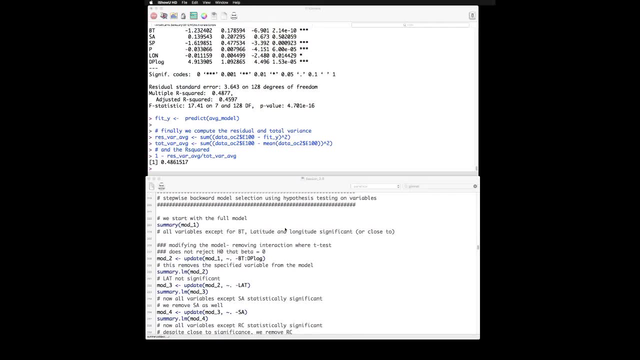 the problems of these techniques in the course, but I will show you how you do it in R and we will compare it later on different options and approaches that you can take to this. So let's start with the full model first, and then we will move on to the next step. 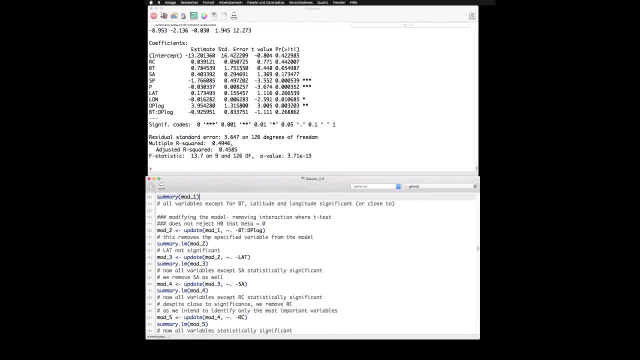 We have fitted this above and we inspect this model and see that this interaction term is not significant. If you start removing variables, you would start removing non-significant interaction terms first. At least you would not remove variables like, let's say, Bt. in this case You would not remove. 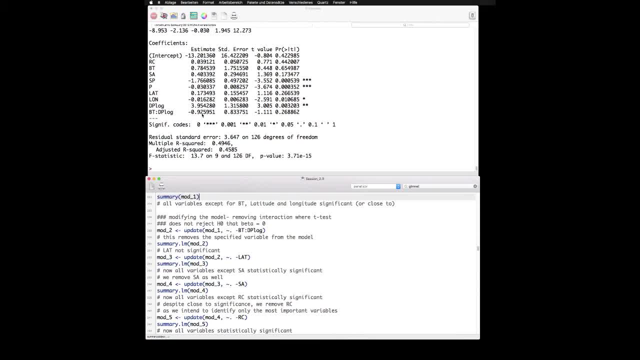 the main variable As long as the interaction term is still included in the model. So we remove the interaction term and that's easily done with the update function. You say update the model, comma for another argument, and it's tilde dot, and then with the minus. 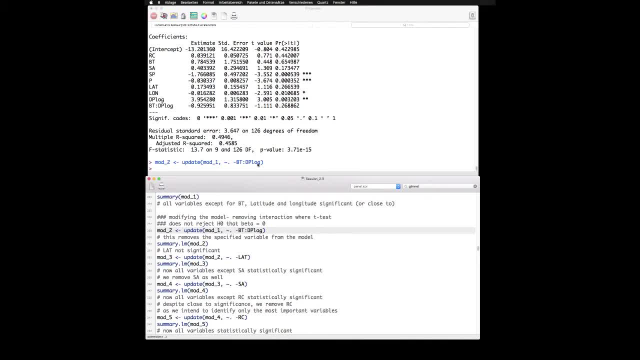 you indicate which variable should be removed, And this could be multiple variables. You could remove them, Remove some, add others. You have several flexibilities with this update function. Let's see how this model looks like after we removed this interaction term. We see then now, except for latitude and SA, which is salinity. 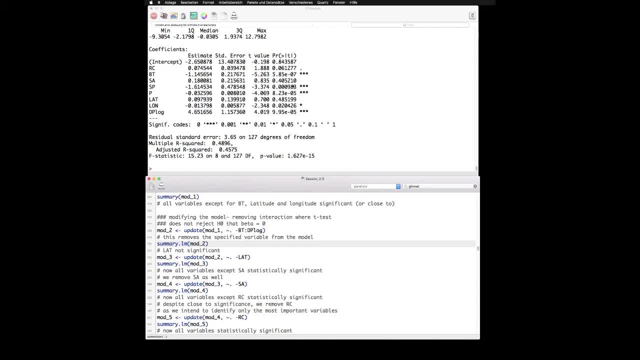 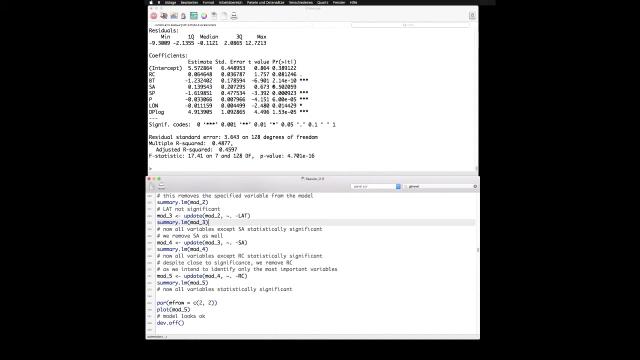 most of the variables, or all of the variables, are now significant RC, at least close to significance. So we remove latitude in the next step And just quickly I removed that and call the summary function again And we have another model to inspect. We see that RC. 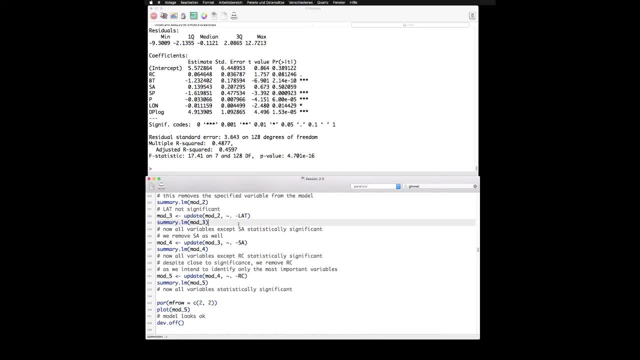 is close to significant, SA shows: no. This is not much different from zero. according to this p-value, That's not significantly zero, Differently from zero. so we remove SA. Next step: now we see that RC is more or less significant. all other variables are significant. Well, we could keep RC. we. 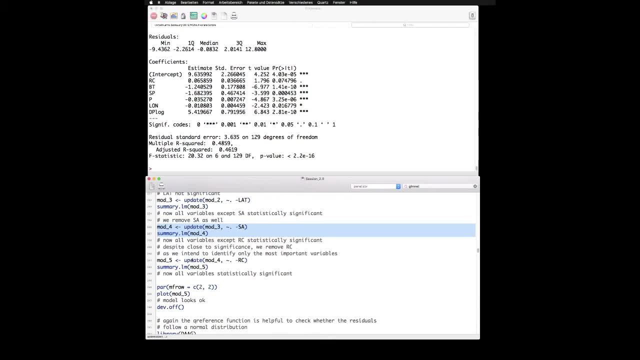 could have, could also have kept SA and other variables. if the aim is prediction, if we expect that the relation structure between the variables is the same for new data sets, In this case we want to know the most important variable, so we get rid of all variables that have not a high explanatory power. 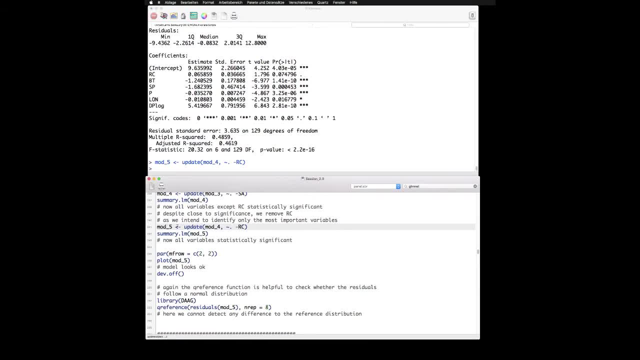 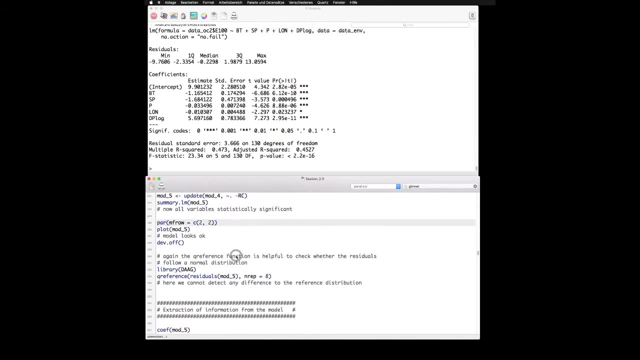 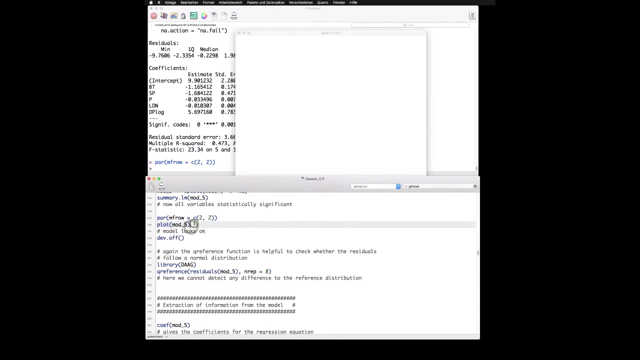 so we also remove RC Summary function again and we see that now all variables are statistically significant, Significantly different from zero, all individual terms of the model. Let's inspect the model First, open the plot window and we define here with MF row that we 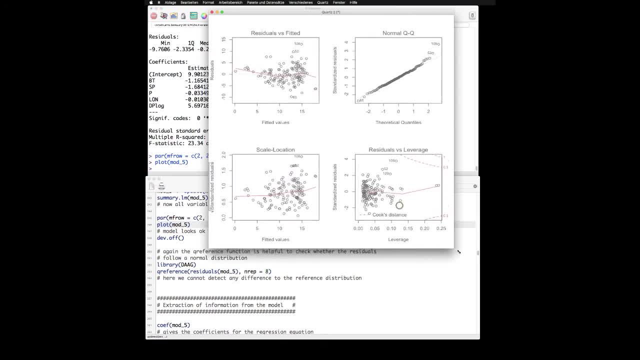 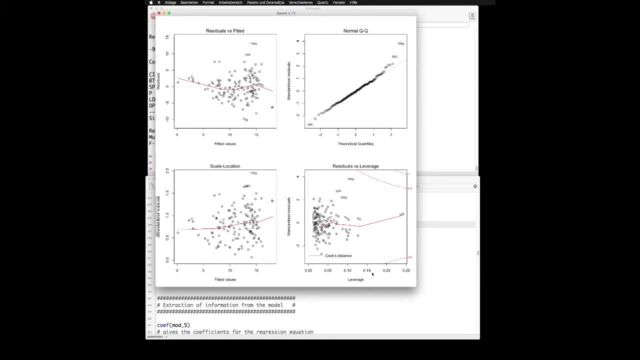 have a two on two window so we can see all four lots for regression diagnosis at the same time. We have discussed regression diagnosis in the lecture, so only go quickly through it here. We see here the residual fitted values plot. Ideally there shouldn't be any increase in variability and it should be more or less a straight. 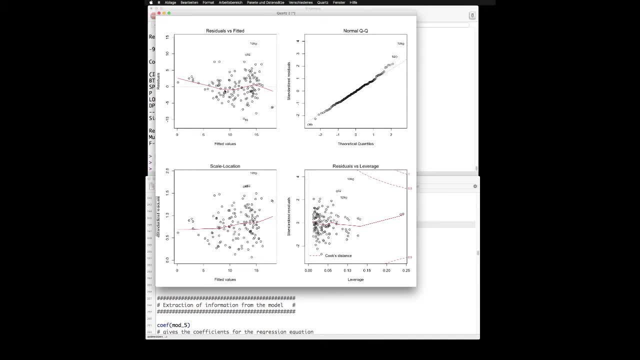 line, We see that this matches relatively well. There may be a slight increase in variability for higher fitted values, as we can see for the standardized or square root of the standardized residual plots as well. Nevertheless, there's nothing to worry if we look at the standardized residuals against the 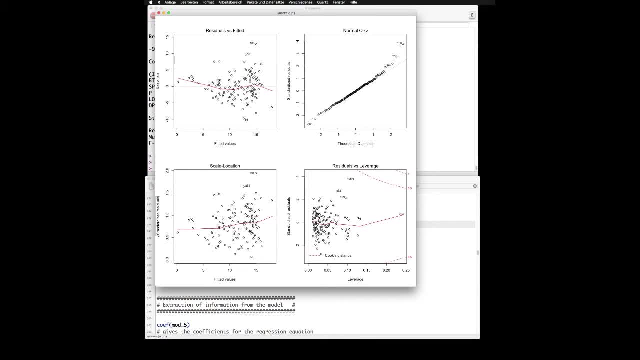 theoretical quanta. as we see, that also fits the line here relatively smoothly. There's not much deviation and if we look at the leverage points and their impact on the model, we have two leverage points, But these have not an high impact on the model And we had a few few points that 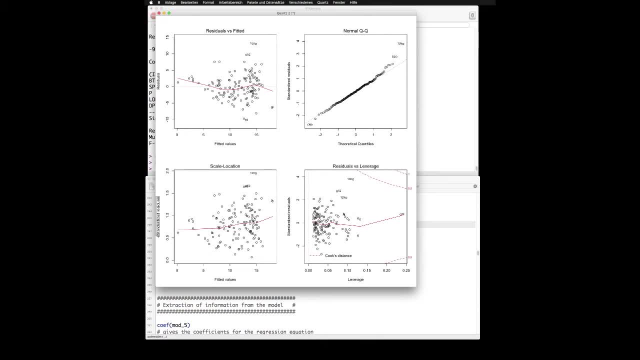 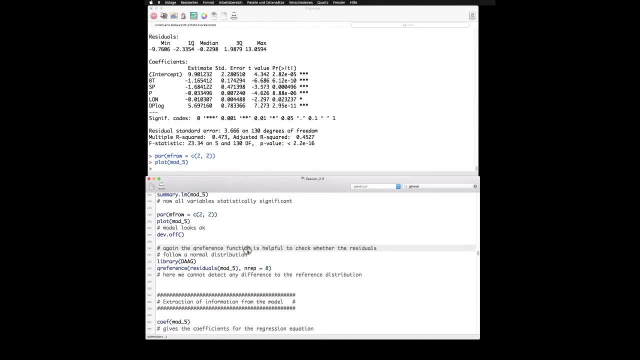 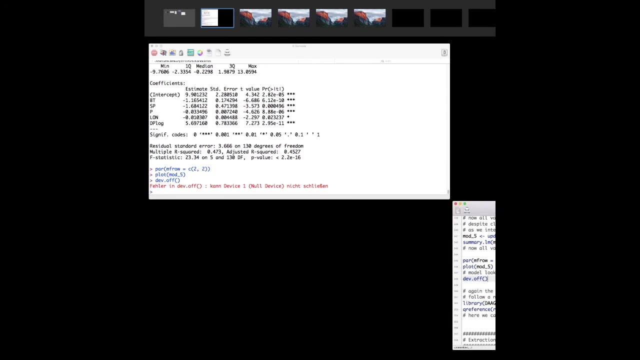 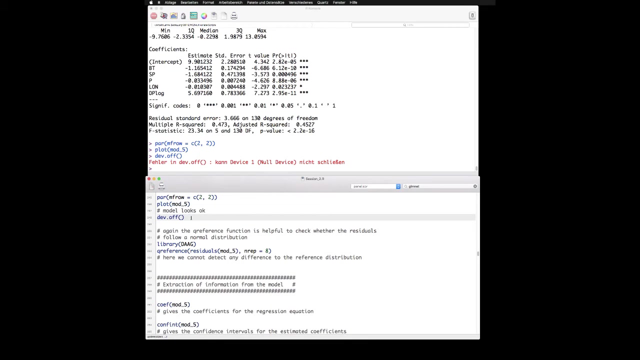 deviate more strongly from the model are buffered more or less by other observations, so there's not much to worry here. So we've already closed window. if you haven't closed it, you could close it with device off. i do this because we have now created a two on two windows of four plots in one window and we don't want to have that in the next. 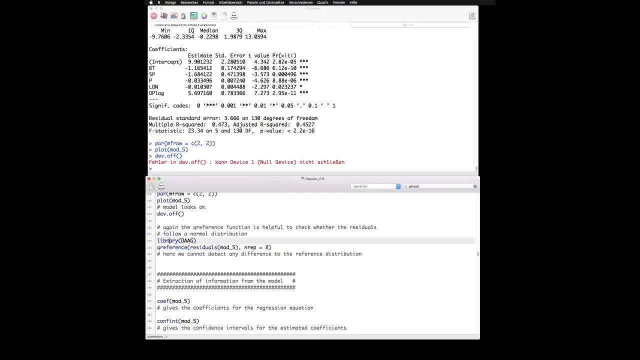 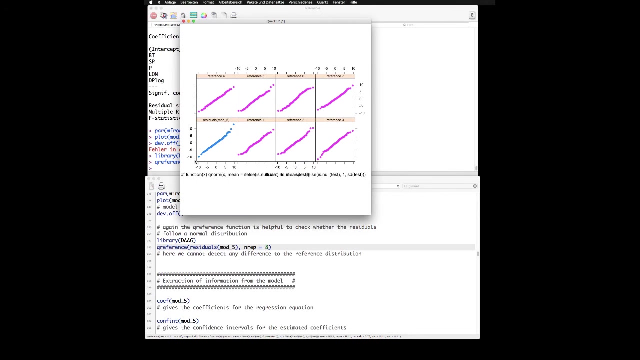 step now. many people say: well, this graphical inspection of models is difficult as a beginner. are there any functions to help me? and one of these functions is the q reference function, because it shows you how residuals from a normal distribution would look like and you can compare this to residuals from your model. so that's how the plot look like. that's the residuals of our 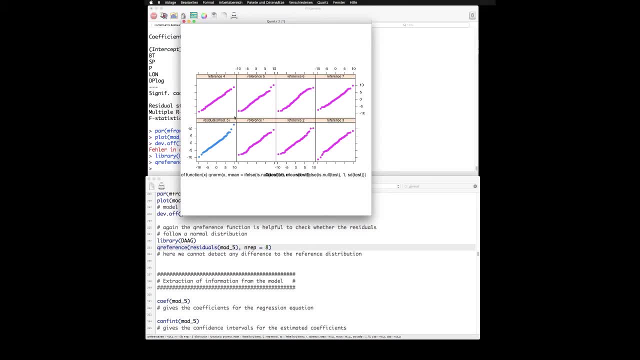 model and you compare these to the residuals that would be observed, or these are actually sampled from a normal distribution and we see the shape of our data points, of our observations are not much, it's not much different to those samples from a normal distribution. so we can conclude: 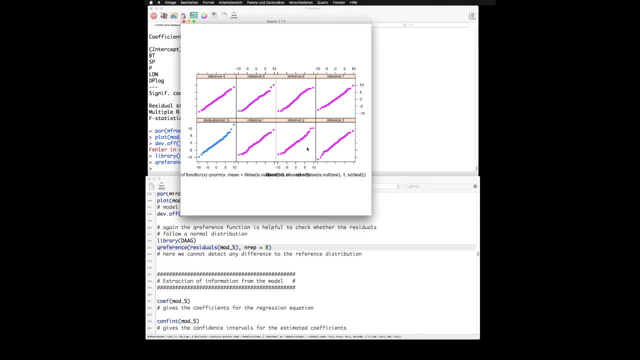 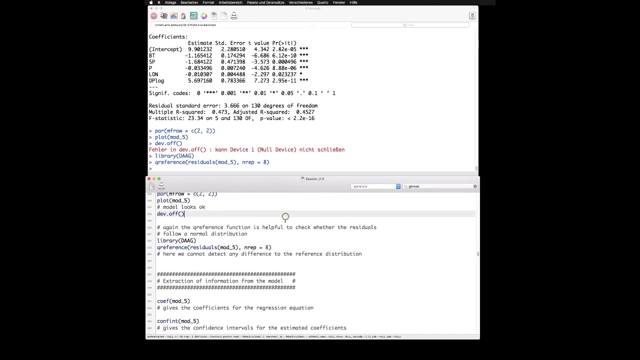 that our data- or we can conclude that it's not likely that we have to reject the hypothesis that our data comes from a normal distribution- looks very, very similar to normally distributed data- not much deviation. if you have fitted a model, you can extract different information from this model. you. 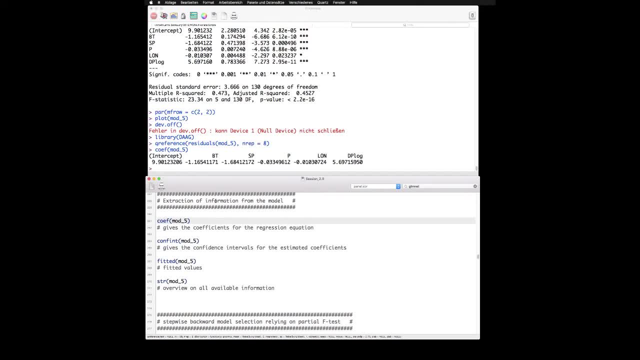 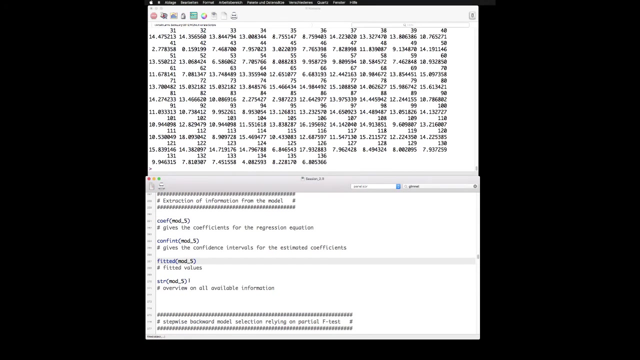 have the cof function that gives you the coefficients for the regression equation we have to convent, and confident function that gives you the confidence intervals for the regression coefficients you can also manipulate, if you look into the function, which confidence intervals you want to obtain. you can receive the fitted models. these are the fitted data points, so, without the error, 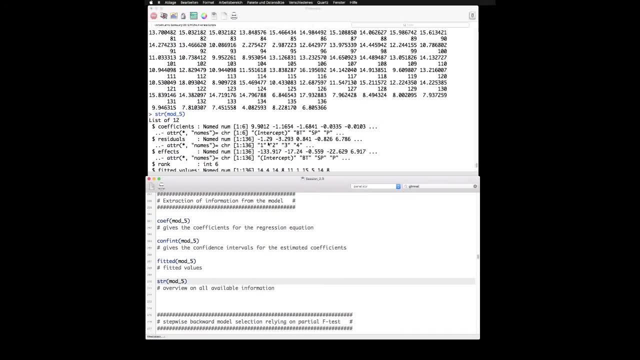 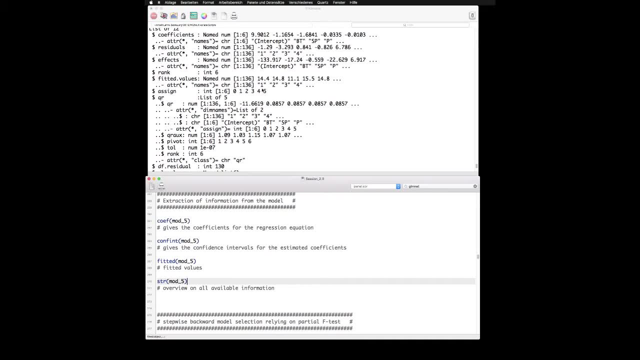 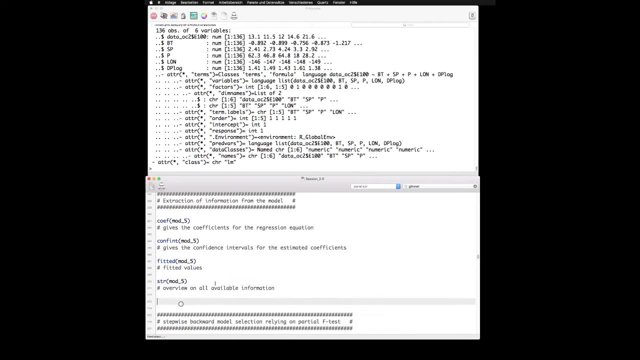 and with string, with the structure, we can look at different elements that you can from the fitted model. So you could also extract the r-squared, the residuals and so on. Now in this example we use the approach of manual model selection, backward selection. We started with the full model and remove variables. Now 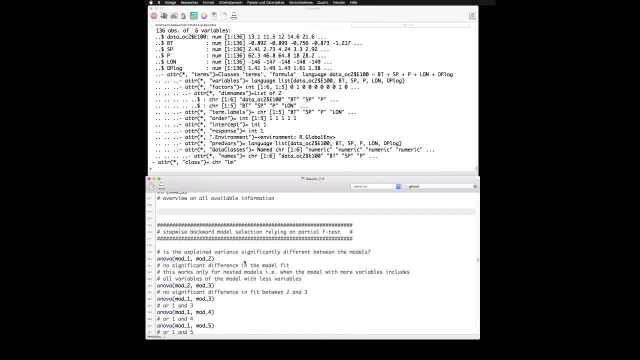 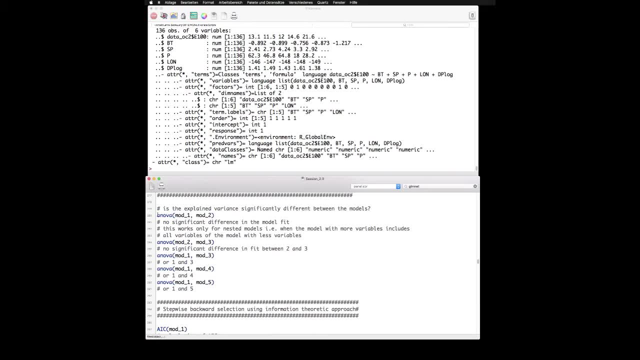 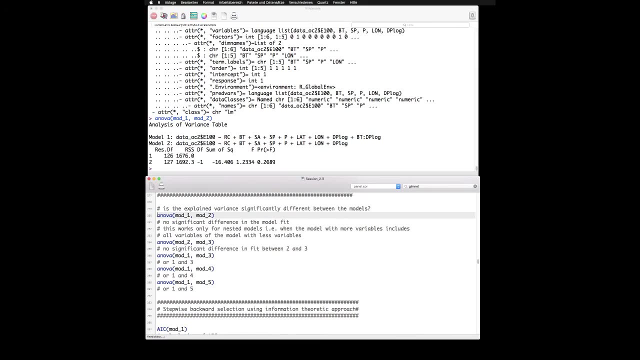 let's see what would happen. We compare this if we would rely on the partial F test. So just compare the models. This would lead in this case to identical results. So we compare here the sum of squares, compare the explained sum of squares between the two models and do an ANOVA. We see that there's 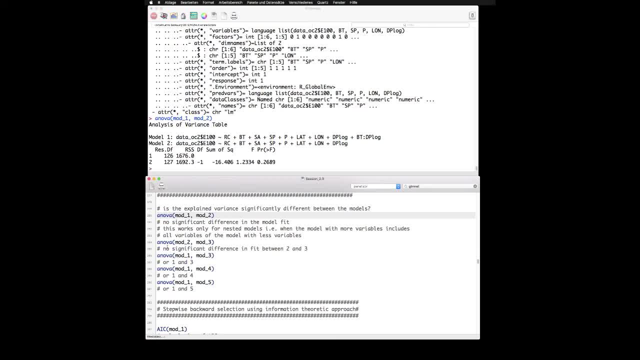 a sum of squares between the two models and do an ANOVA, We see that there's no significant decline from the model with 1 to 2 when the interaction term has been removed. The same holds if we compare model 2 and model 3.. The more parsimonious model has 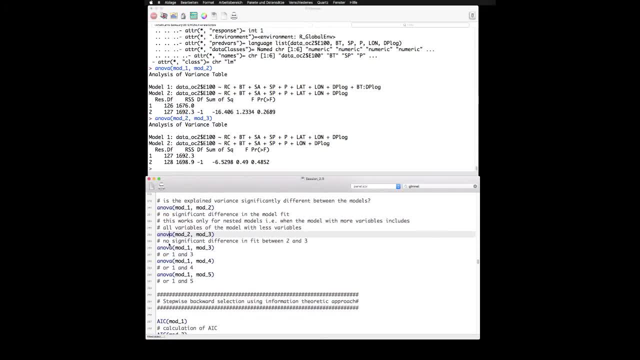 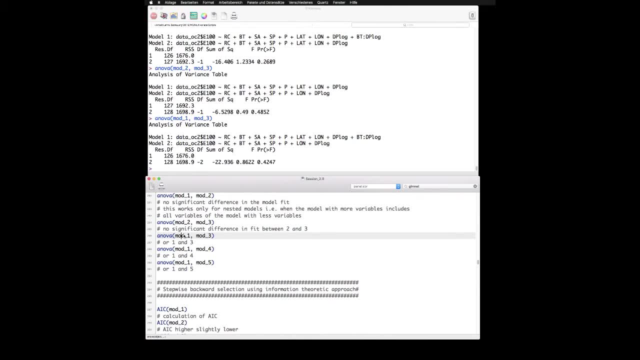 still no significantly lower sum of squares. We do this for several other models. again, No sign that we have a problem here: Model 1 and model 4, model 1 and model 5.. And we see that any of these comparisons is. 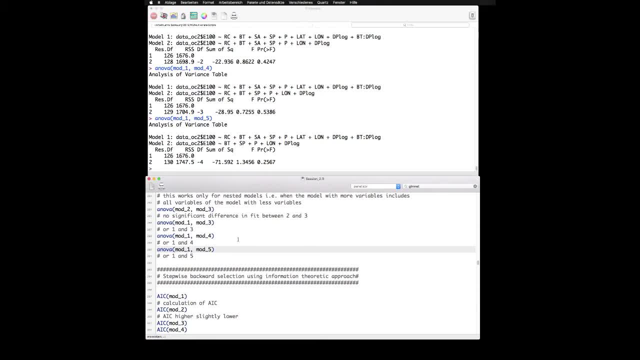 statistically significantly different. So that means we have nested models. we can use the partial F test to see whether we have statistically significant difference in the variance that is explained by the model. This is not the case here between any of the models, So what does this mean If we have a similar? 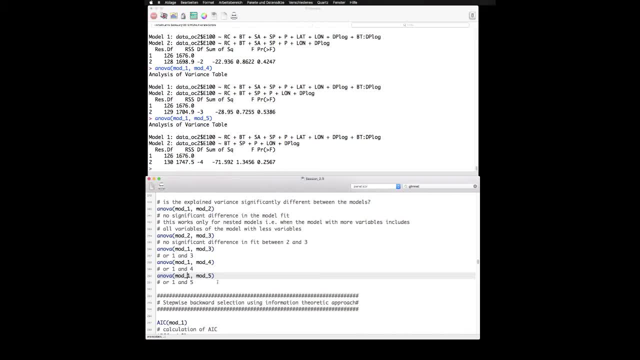 explanatory power. so we cannot reject the hypothesis that explanatory models have a similar power. the power differs between the models. then we should of course use the model that has the lower amount of variables, Because if you can explain something with fewer variables, why should you use more variables? 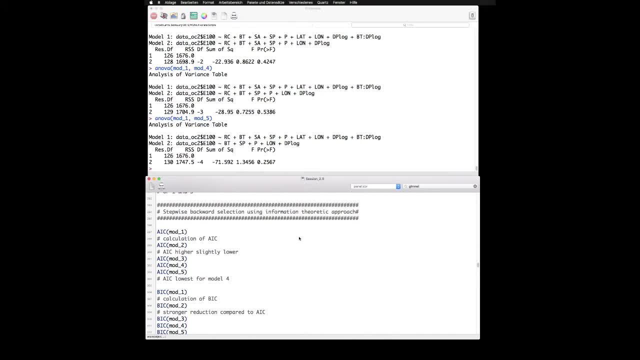 Another approach or another goodness of fit measure other than hypothesis testing. we have discussed in the lecture are information criteria And we have, on the one hand, we have the Bakayike information criterion, We had discussed the Bayesian information criterion And finally we 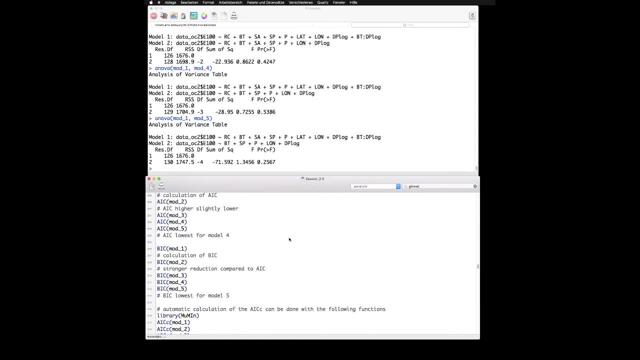 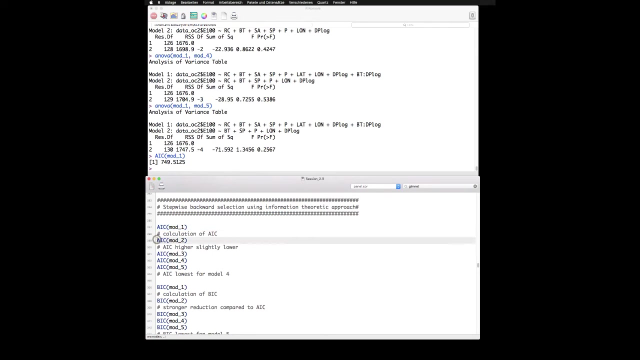 have the corrected AIC for lower sample sizes. So we calculate all of them here and see what they would suggest for identification of the best fit model. So let's fit the AIC First. we see we just obtained the result for the AIC. Note that the smaller the 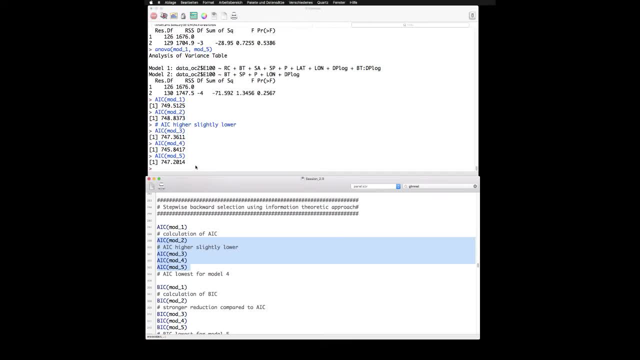 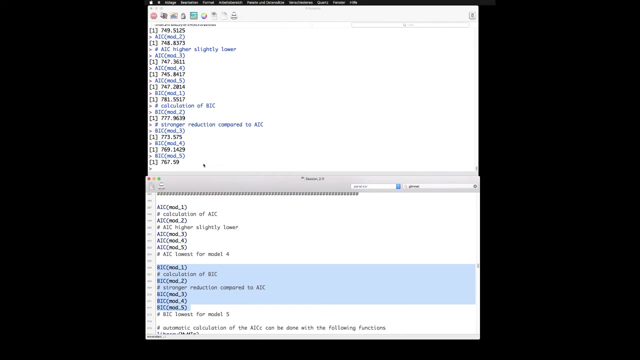 better is the model fit based on this information criterion. We see here that the AIC would actually suggest that model 4 is the most parsimonious or the most appropriate model. If we use that, the BIC just fit all this. then we see we have for the BIC, we have a constant. 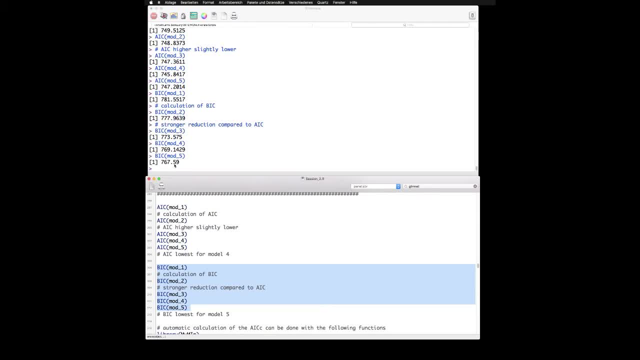 decline from 780 to 767.. So we would also this would also suggest that we keep the model 5.. But note, I mean in this case, if we would do this manually, we would remove another variable and check whether the BIC is correct. 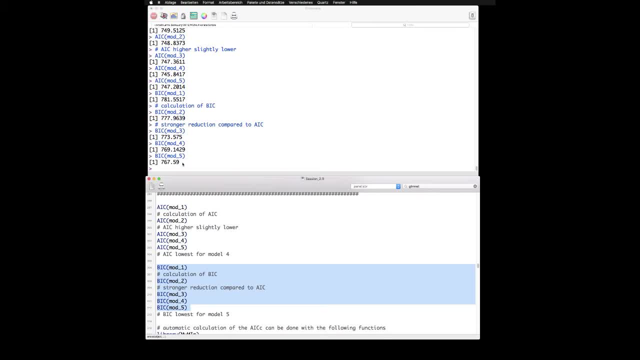 So this gaps in clause the highest I Chelsea ubine Dväg感謝, for example, would be declined if another variable is removed from the model. to do Finally, I just showed us here, in this case it's not necessary. all this is not. 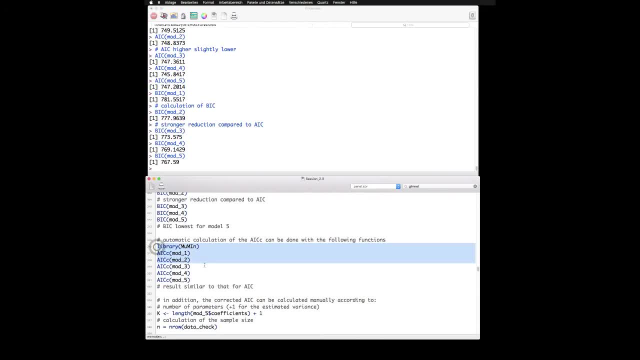 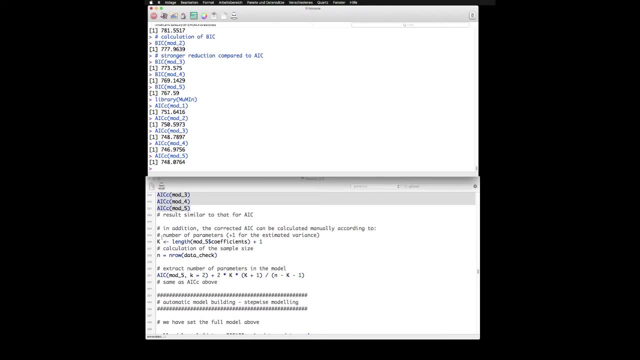 really necessary for the AIC. we have the corrected IIC. we see that leads to the same results. It also shows you the script how you can calculate the corrected IIC- 그러멱sostäHS IIC- yourself, if you don't want to load a new package. it's just dependent on the. 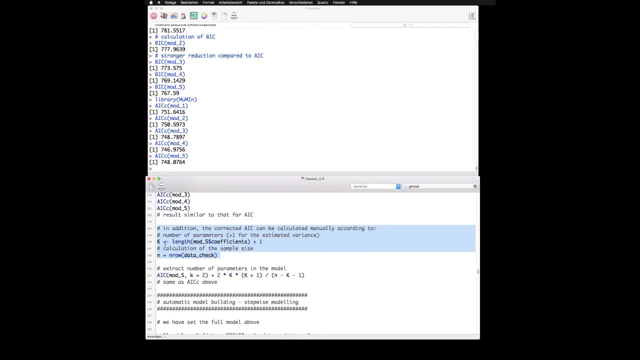 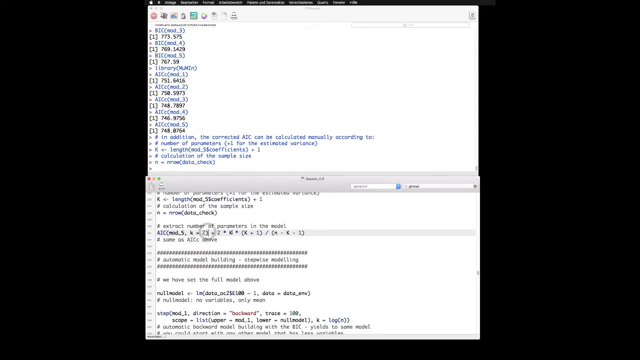 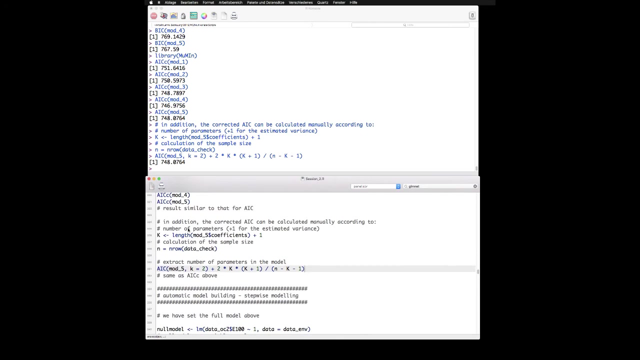 number of coefficients in the model. so that's K and you have the number of data points. then you have the formula here. you have displayed the formula on the slides for the lecture and you obtain the same result as for the as the one that is calculated automatically when running the corrected IIC function AIC. 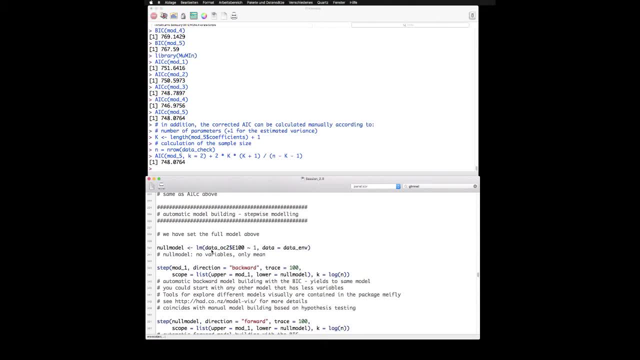 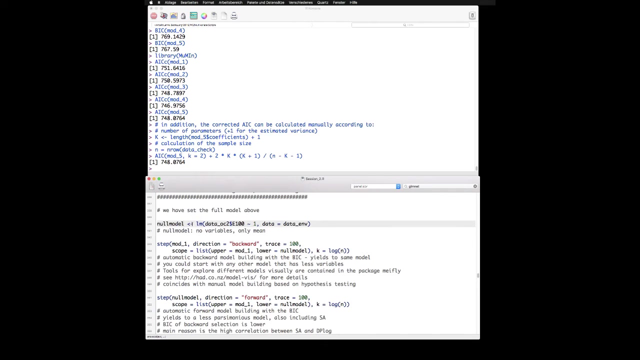 minus C. so that was manual model building and the next step we look at automatic, automatic model building. I have stated- you put several statements of caution on the lecture slides, I'm not repeating them here- should be aware that, not that just running automatic model building is no solution to scientific problems. you need to know what you are doing, why you. 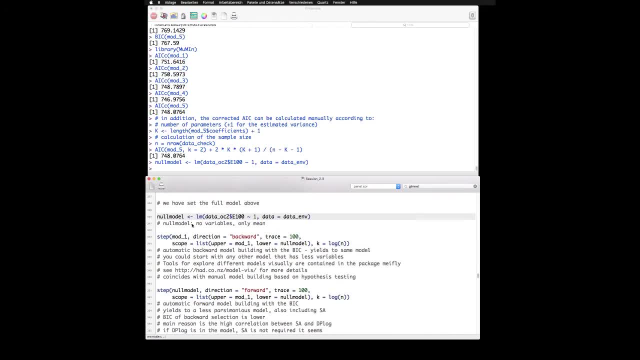 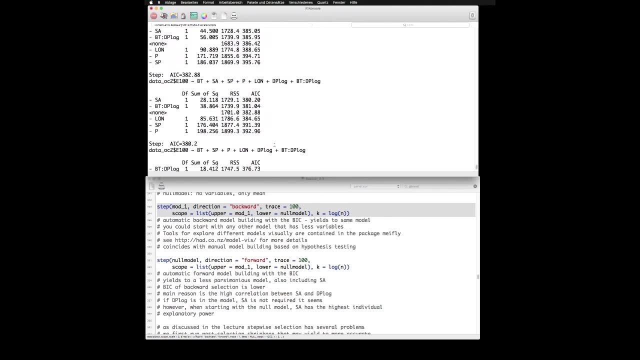 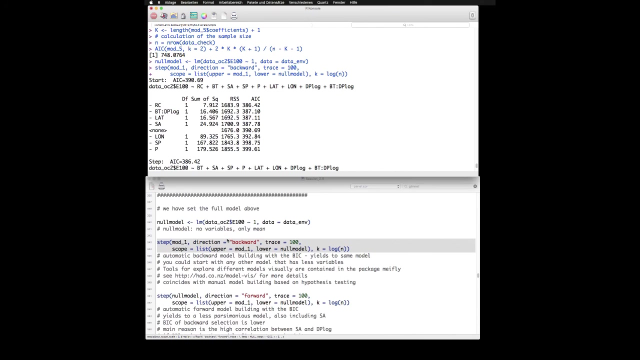 are including variables, and then you can make inference. computer can't decide for you and just tell you which variables are most important, and we'll with also select various ones. so what happens if you run such a model? or let's first again go back to how you set? 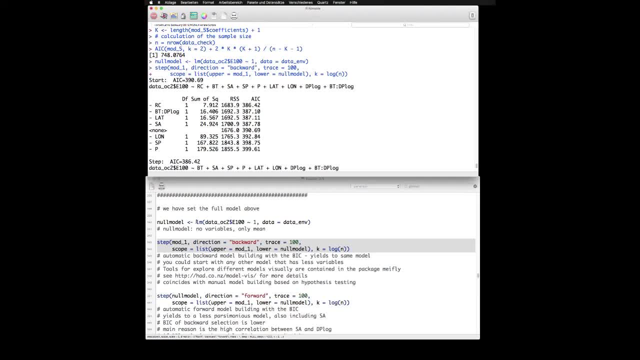 up such a model. first of all, you fit a null model. that's the model that you would say: well, that is the smallest reasonable model that we could assume of. In this case, this is a model without any variables. It would contain only the mean that is fitted by the response variable, tilde 1.. 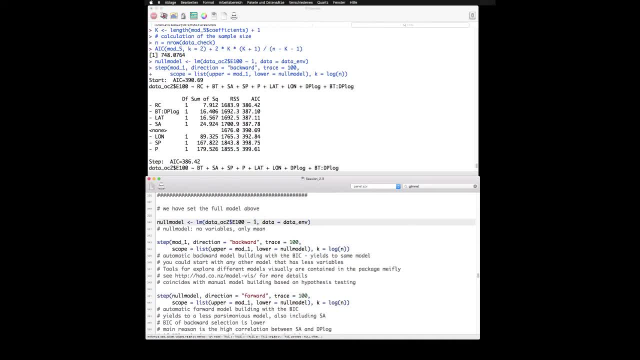 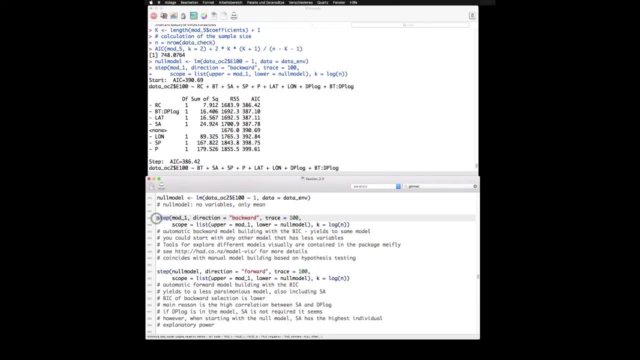 You could also say: well, the null model is a model that contains at least one or two specific variables. I don't want to have any model with less than these variables, because we have solid evidence that these variables are of high importance. Then you have the step function. 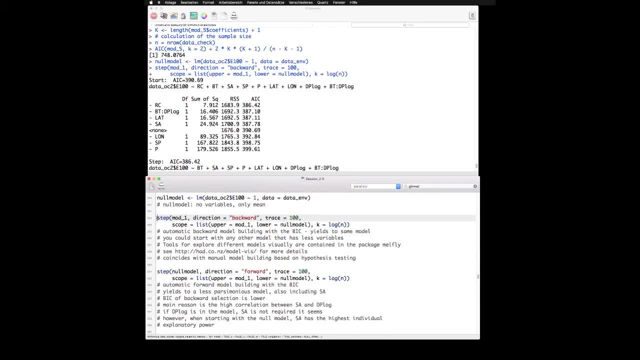 The step function does the stepwise modeling. You have the model that you start with. Then you say which direction You want to run the stepwise regression And you have the scope. The scope here is the upper model, the most upper model that you have to provide. 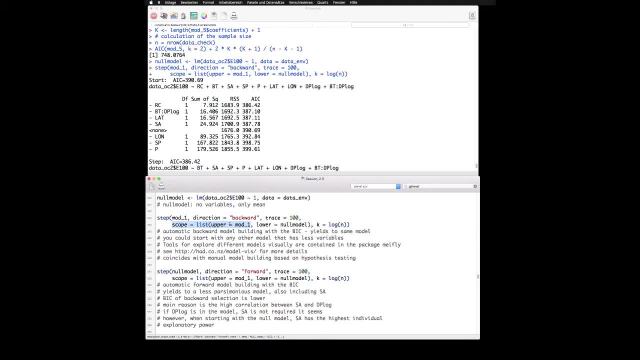 You have to provide this mainly when you do forward and backward entering of variables. Just do this to simplify the code here for the forward modeling. So here we say: well, the upper limit is the model 1.. It shouldn't include more variables. that is contained in model 1.. 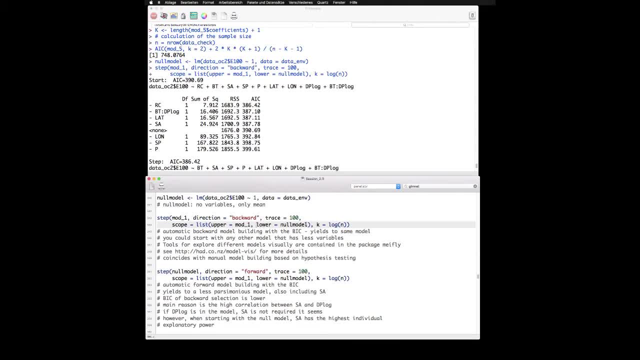 And the lowest model. So that is the model 1.. The upper end is the null model. Note that we use the BIC here. So we want to be more restrictive because we want to find the most posimonious model. So that's k equal log n. 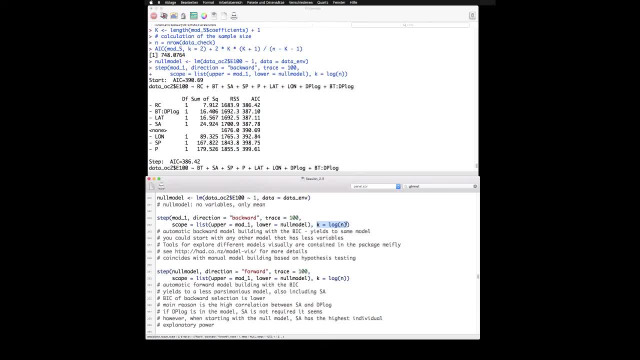 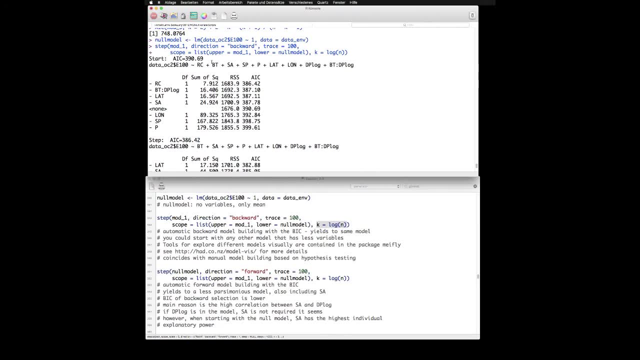 If you leave the default, which is k equals 2, then you would use the AIC And you see The algorithm in R starts, calculates for the initial model, the AIC, And then it checks how the AIC would change if nothing would be done. 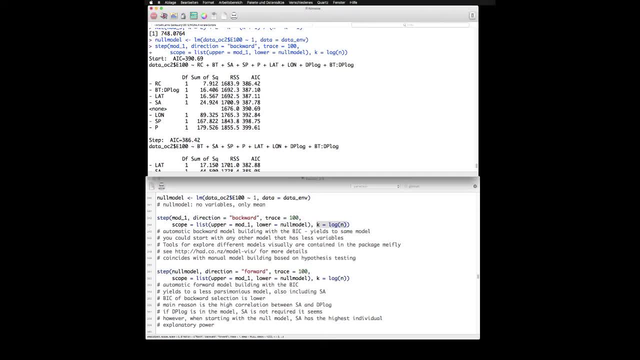 Or if a variable would be removed and compares this AIC to the initial AIC, And as long as this is one of the AICs for removing one of them, Variables or terms that are one of the terms, including interaction terms, leads to a lower AIC. 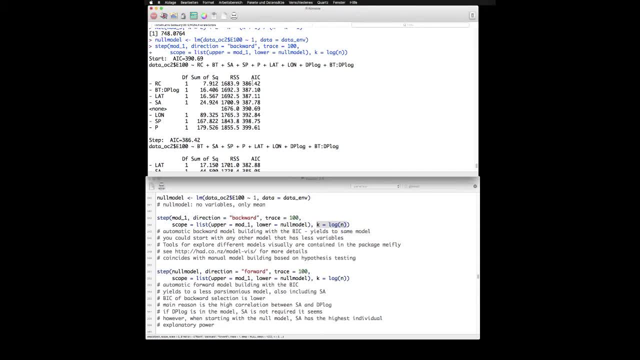 This is executed and it just focuses, of course not on any scientific meaning of the variables, It just selects that one that has the lowest AIC. So we see this is done again and again. First it removes ARC, Fits the model again. 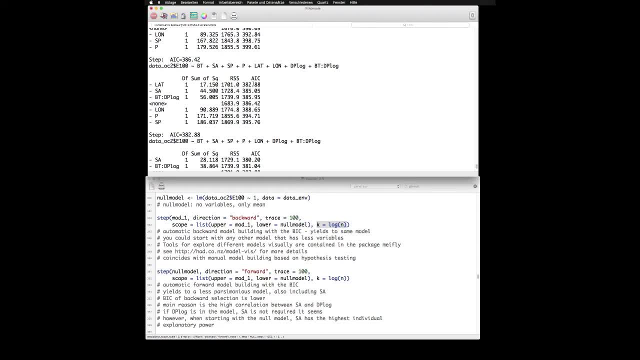 Now without RC, Then checks what happens if another term is excluded from the model And fits the model again after excluding the next term, which is latitude, And this goes on and on until we arrive at the final model that only contains five variables. 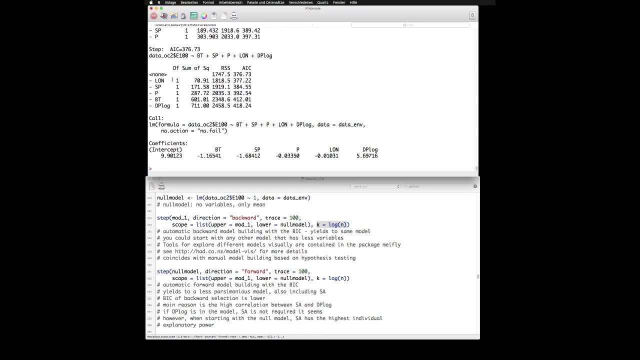 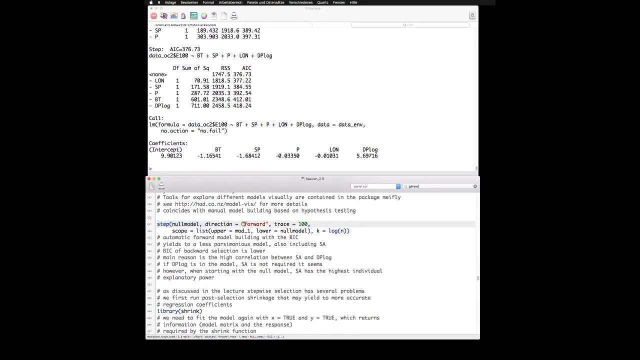 So this is the model where longitude, SPPBT And DPLog are still contained And we get the regression coefficients. here We could also run step function with forward modeling. And what is interesting, here We start with the null model And the first variable. 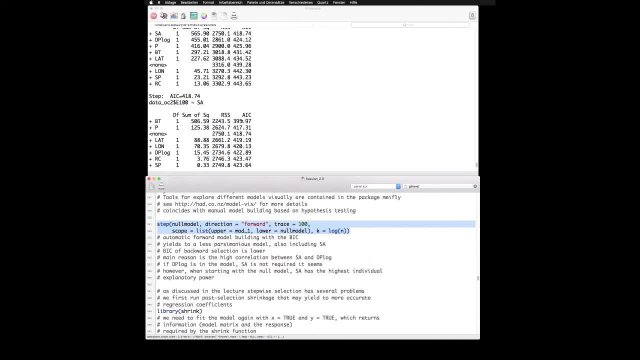 That is, include, is SA. So that means that would be the single most important variable. if we just include one variable according to this procedure And we end up with a different model, It is the same model as the one above, but also including SA. 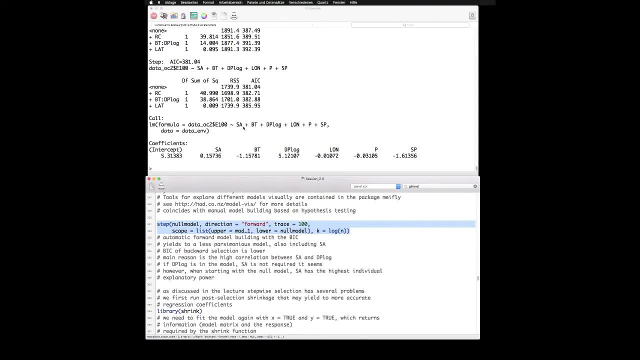 So it contains one variable more. So that should cast some doubt On these procedures as well, Because if you change a different direction of the procedure, You obtain a different model, And the variable that is supposed to be one of the most important alone. 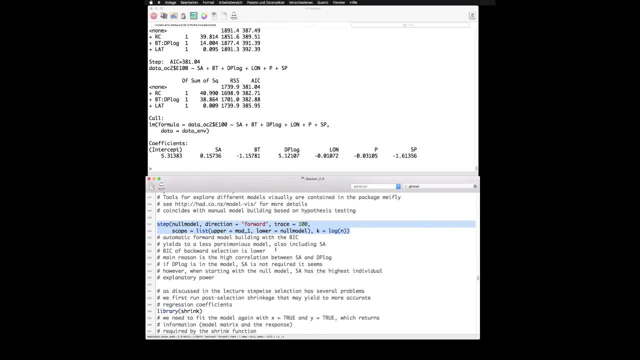 SA is not included in the backward model. You can't say which one is correct or incorrect. As you know, SA is highly correlated with DPLog And we would need salinity And the logarithmic depth Which makes sense, And we would need more information on the system that we are looking at. 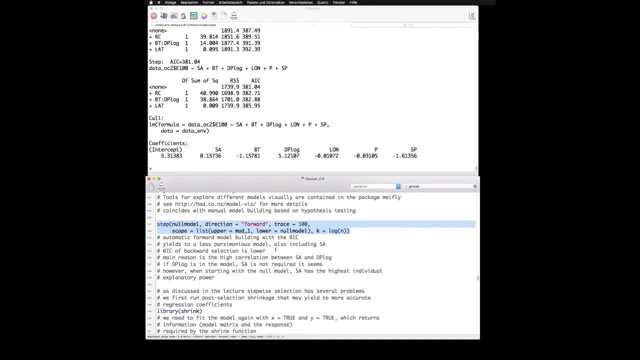 To decide. well, Is this a correlation where actually only salinity is physiologically effective And the logarithm of the depth is just a spurious correlation? It is not that important for the model, It could be removed. Or does depth? 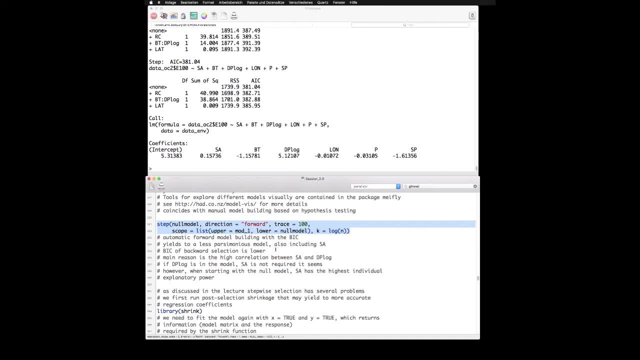 That the logarithm of depth Have an individual important explanatory power. For example, there is less light and less food. That may be another explanation. Well, we don't know Why, we don't speculate, But this shows if you have such results, 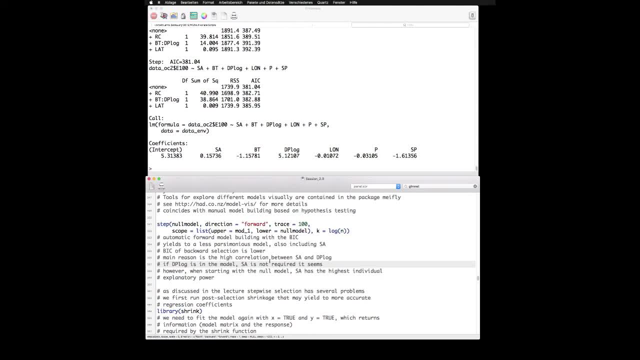 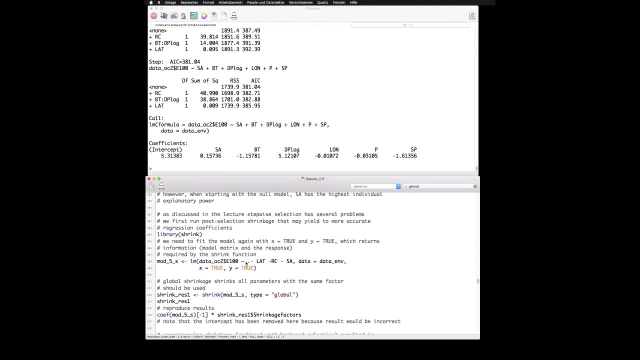 Don't just let the computer decide what is the best model. We discussed in a lecture that There are several problems related to this approach. One problem is that we have regression coefficients That are biased high And one possibility to correct for this. 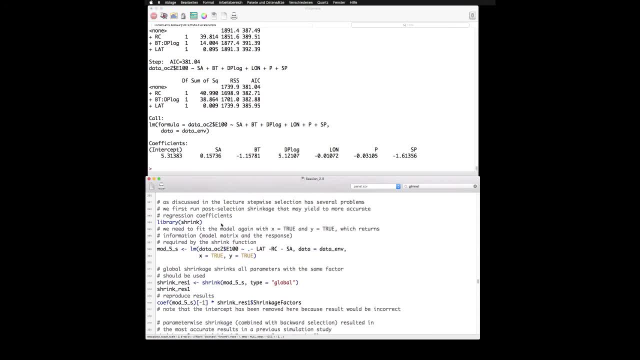 Is to run post selection shrinkage. That may yield to more accurate regression coefficients. For this we use the library shrink. We have two options. We could either shrink the whole model With all variables. The same factor is applied to each variable. 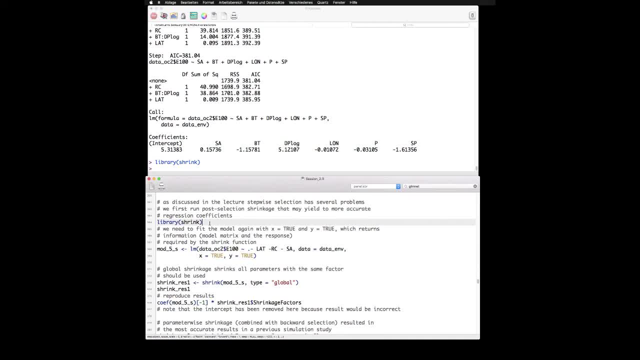 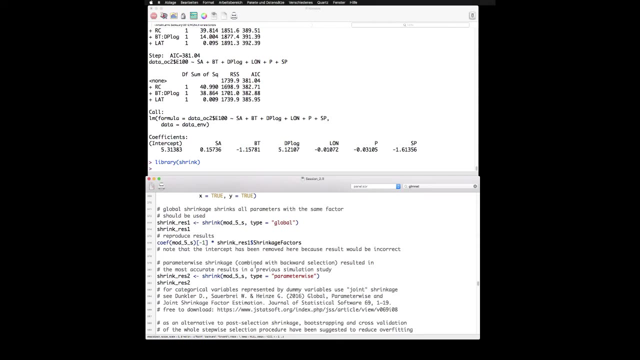 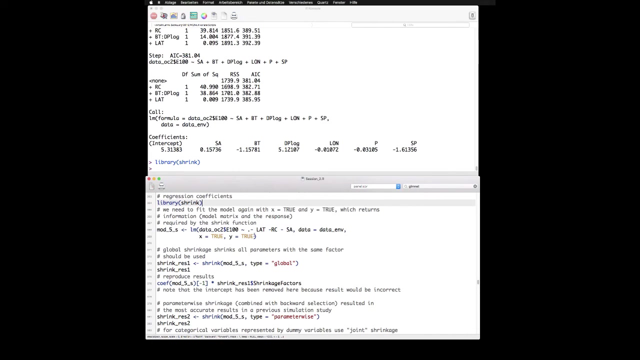 Or we can have parameter wise shrinkage. In some comparison paper, They found that this parameter wise shrinkage is more accurate. Anyway, before we can shrink, We need to remove some variables from the model, And so we need to set up a new model. 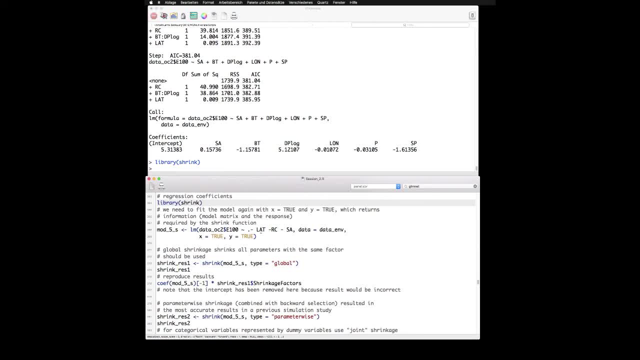 We set up model 5 as shrinkage And one important aspect. We need to provide some matrices That are important, Some elements, Some information for the shrinkage function That is not provided by default By the lm function. So we fit the lm function again. 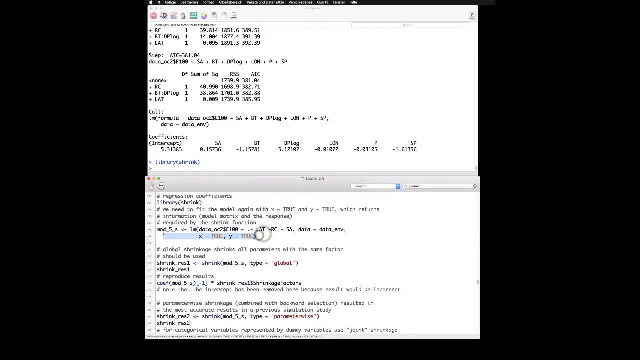 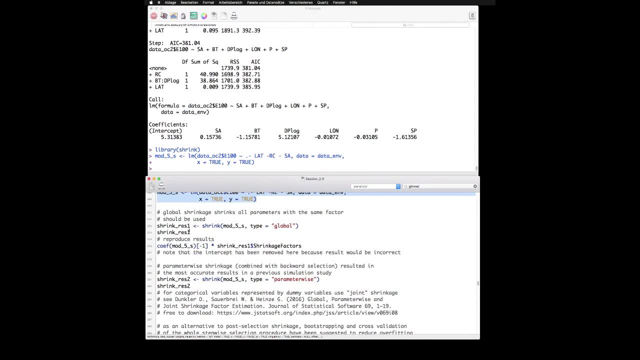 With x equal to and y equal to. If you run the summary function of this, You would obtain the same result, And then we can run the shrinkage function. Let's just shrink the model And the type of shrinkage that you want to use. 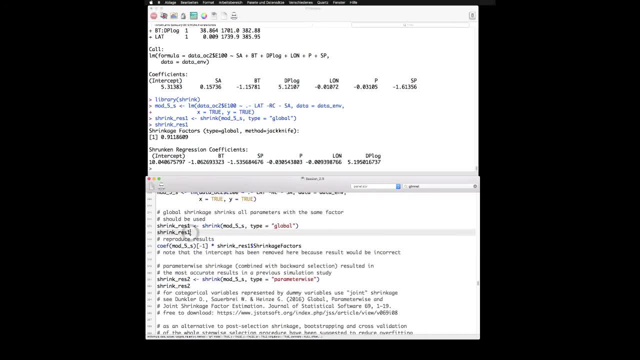 So we shrink the regression coefficients And we see that there is a shrinkage factor That is 0.911.. So approximately 10% of the regression coefficients are shrunk And if you compare this to the original Recursion results, 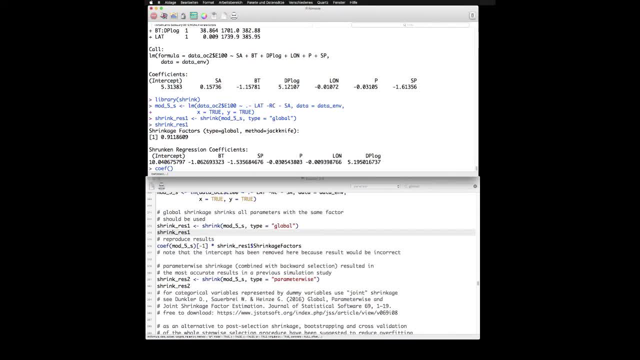 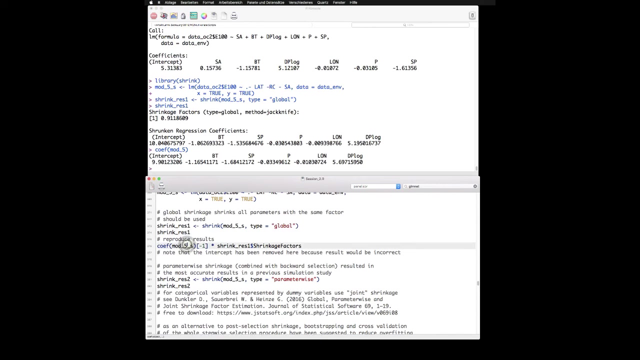 So type F 5. We see that the regression results In the upper row here Are approximately 10% lower Than those of the model 5. That has not been shrunk To reproduce the results, So you see it's. 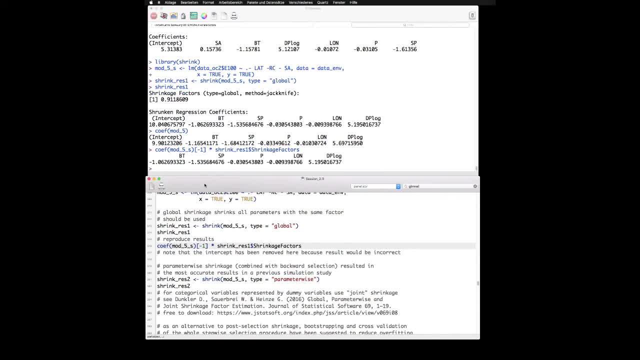 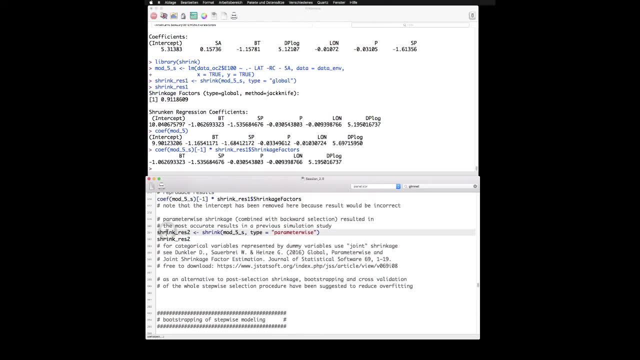 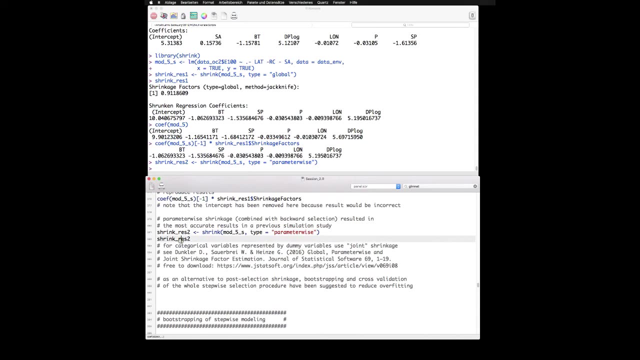 That is how this is calculated. You just take the shrinkage factor, Multiply it with the regression coefficients. Now we conduct parameter wise shrinkage, So each parameter is shrunk individually Based on its importance in the model. So refer to this application. 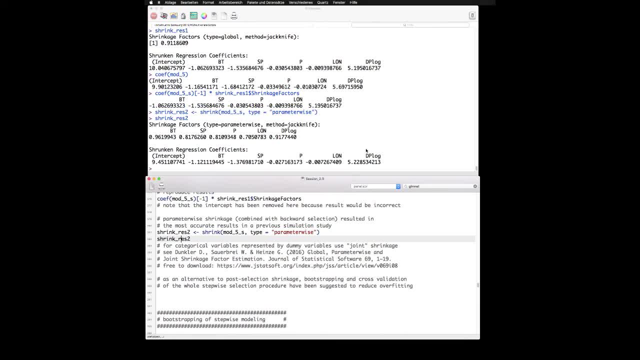 For more information And what we see here now. If we compare this To the original model, Then we see That there is a different amount of shrinkage. For example, S P Is much more shrunk In this model. 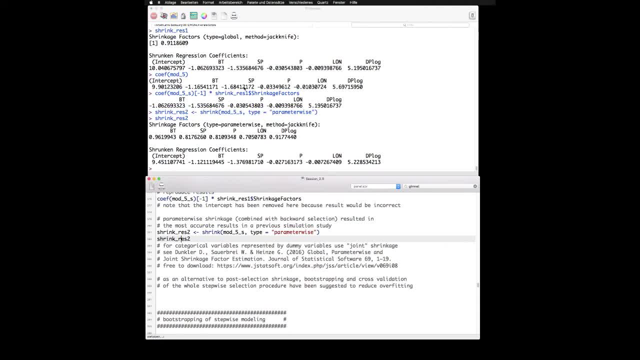 In this model. compared to B T, That is not as much shrunk And longitude Is also shrunk To a stronger extent Compared To a similar extent. That is about 30 percent. okay, Is about A little bit more. 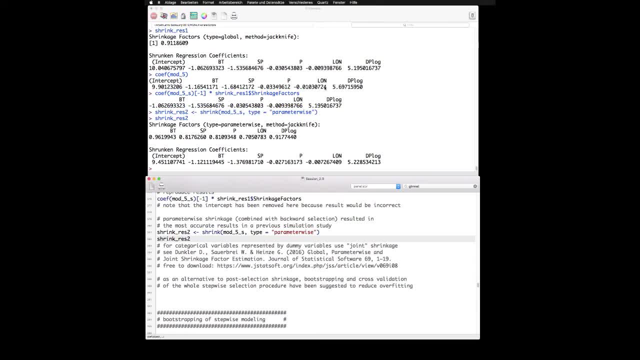 For P. So we see they are different. At least it differs To the extent to which it has been shrunk. So Why do we do this With these shrunk regression coefficients? We would expect That we have a higher. 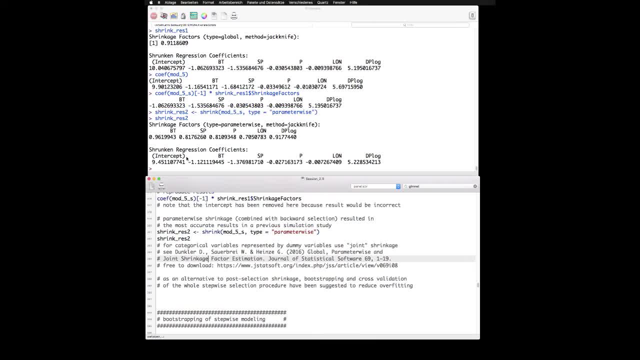 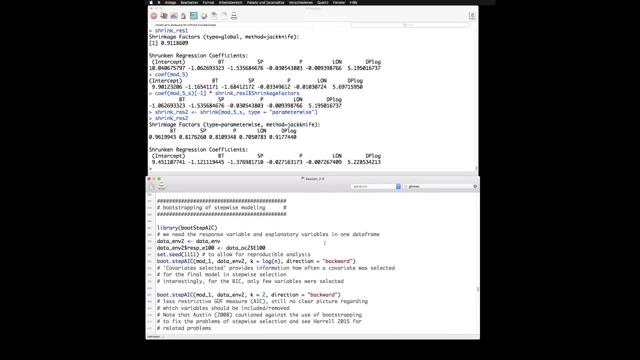 Explanatory power Or higher Predictive power For new data Sets. Another approach To deal with the problems Of Stepwise model selection Is to Put This whole Stepwise model selection Process Into. 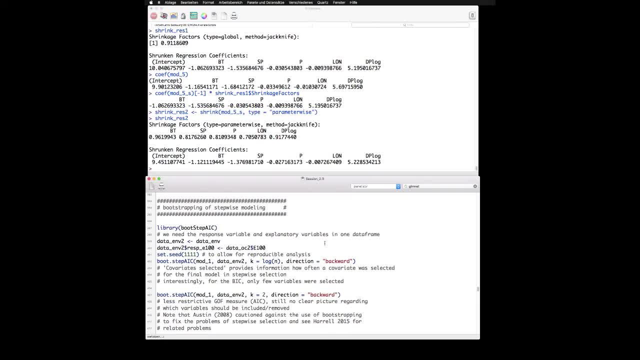 A bootstrap Algorithm. That means We Draw Several Random Data Sets From our Initial Data Sets And We check, If There Is Any, Whether These Sample Data That has. 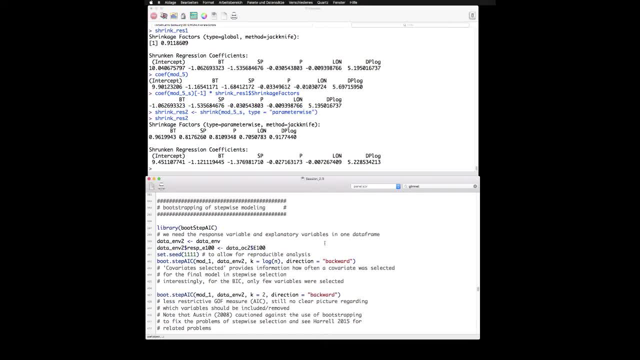 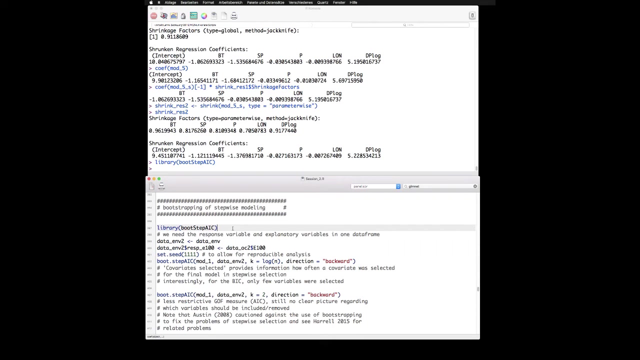 The same Characteristics As The Initial Data, Whether When We Have These Random Different Random Data Sets, Whether The Bootstrap Data And Overall Data Sets, And 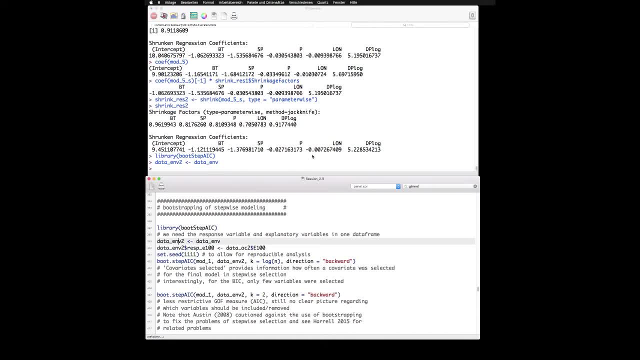 First We Construct A New Data Frame Because In We Need The Response Variable And Explanatory Variable And One Data Frame Later On Some Explanatory. 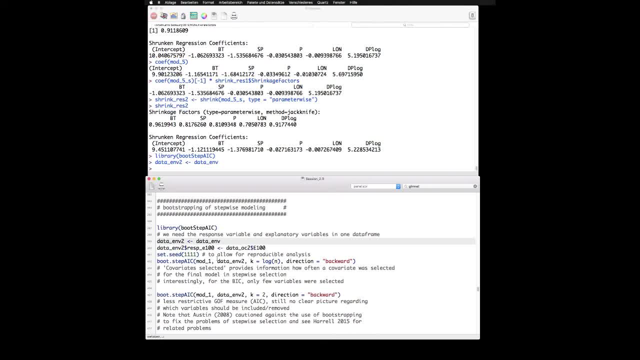 And And The Response Variables, But Are, Or There Are, A Function That You That Uses, That Uses These Input Data, Requires Us To Provide Different. 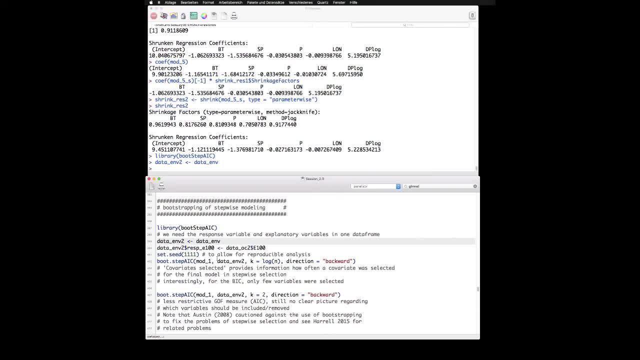 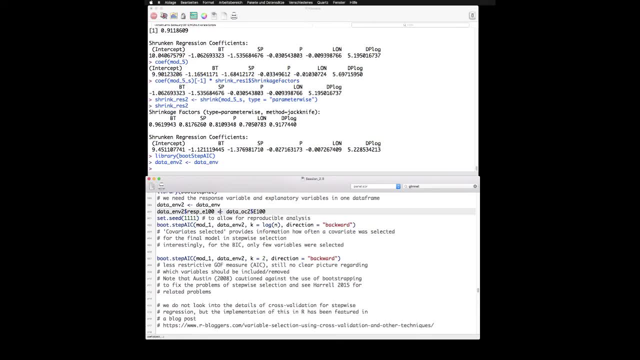 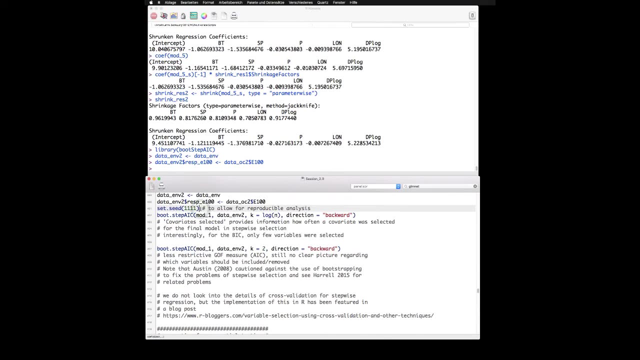 Formats Of Functions To Make Sure That You Always Provide The Correct Type Of Object. So It's Not About The Content Itself In Terms Of 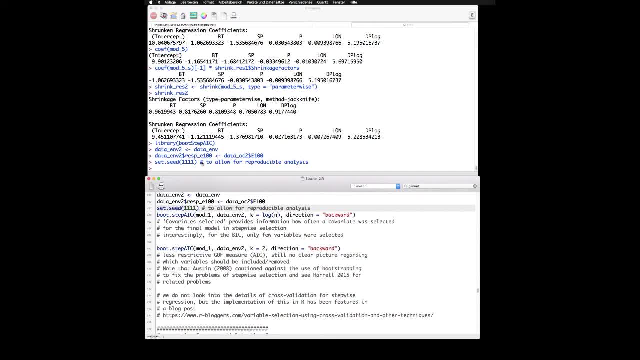 Scientific Content, So We Always Have The Same. As You Know, Computer Can't Be Really Random In A Sense That It's Completely Unpredictable That. 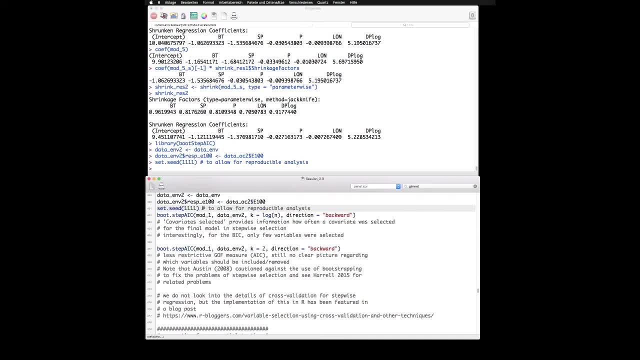 Starts With Some Random Number Generator And Which Random Number Generator And Numbers I Use. Now We Run The Boot: Step A, C Function. So It 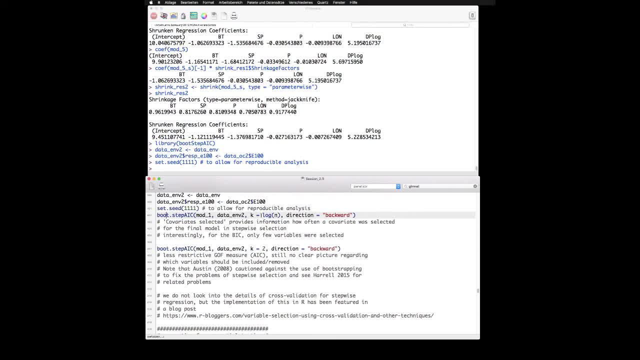 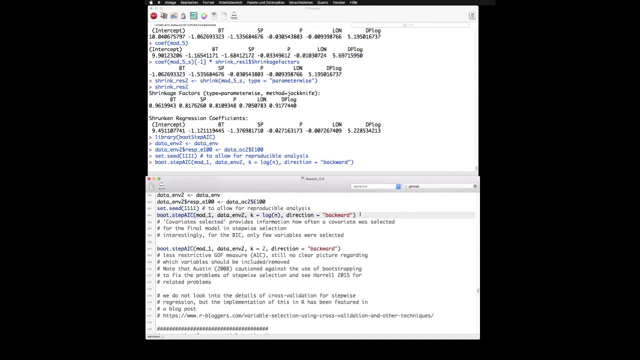 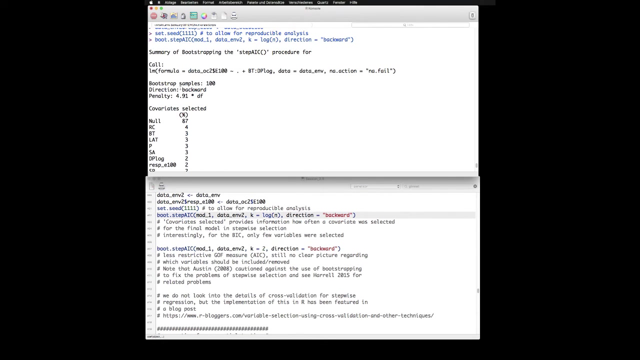 Has As Input The Model And Data Set That Contains All Explanatory And Predictor Variables. Next A Little Bit For This Number Of Variables, And 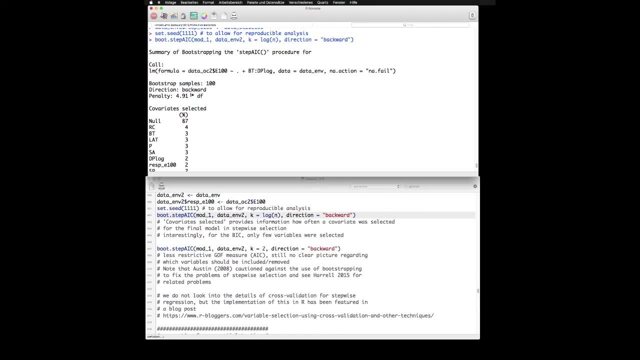 What Is The Output Here? We See The Call To The Function. We See That 100. Bootstrap Samples Have. We See That Most Of The 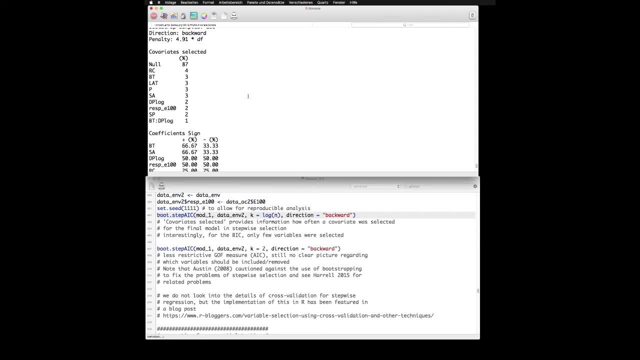 Time, None Of The Variables Has Been Selected, We Can't Really Decide Based On These Results. Here We See The Consistency In The Variable Can. 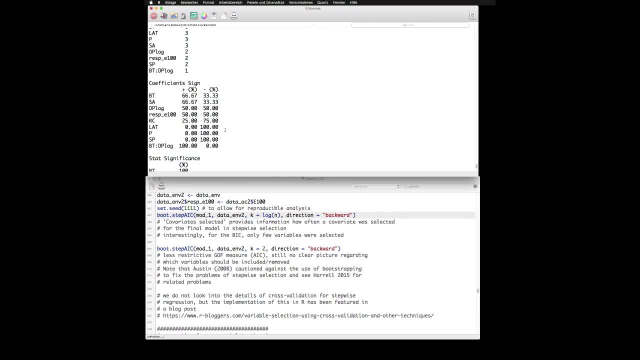 Be Have A Positive Or A Negative Effect On The Response, Which Is A Little Bit Strange, Or It Should Ring A Bell For Caution. 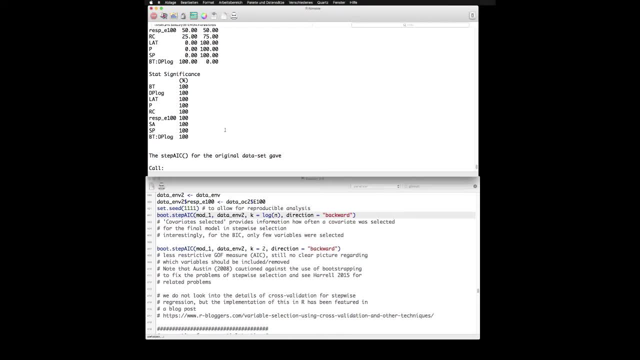 In Interpreting That Of Relationship. Then We See The Statistical Significance For The Variants- One Included In The Model- And The Coefficient For. 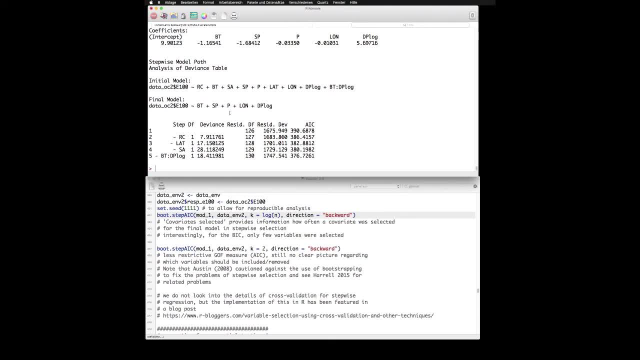 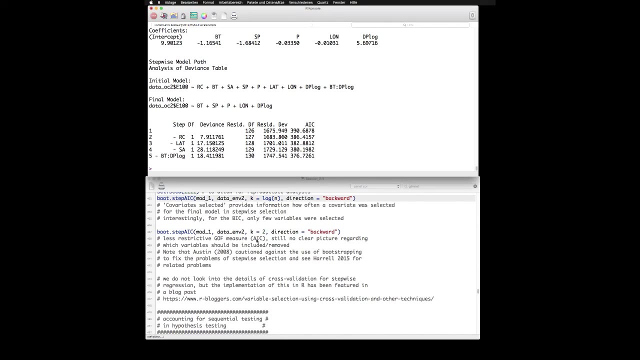 The Final Model Or For The Variables, For The Model Above, So For The B I C, Is A Very, Very Restrictive Model, If We 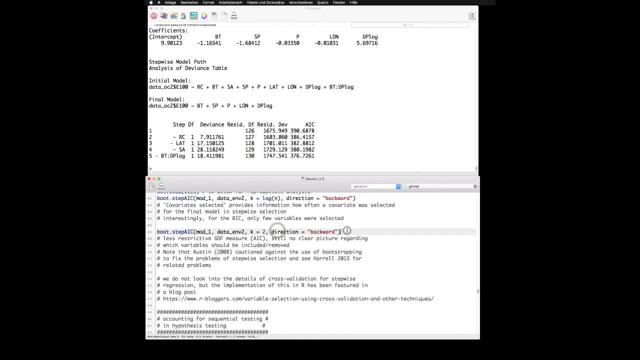 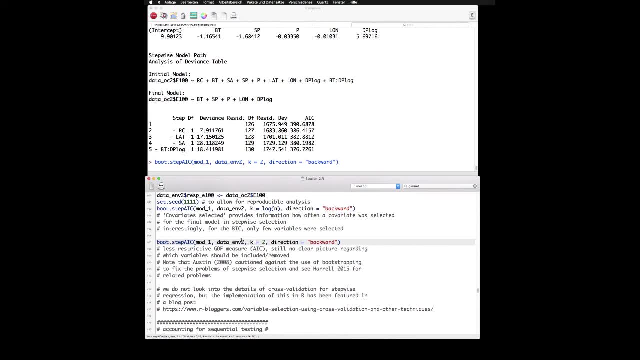 Just Sample Random Data From Our Initial Data Should Cast Some Doubt, At Least In The Model. We Then See That We Select Cooperates Much. 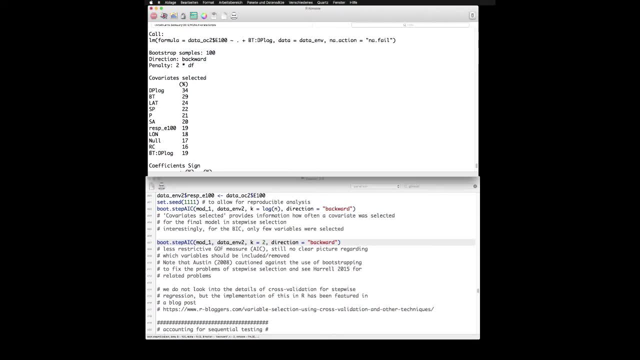 More Often We Have. We Never End Up With A New Model For This Bootstrapping And We See That Continuous Distribution Of The Number Of 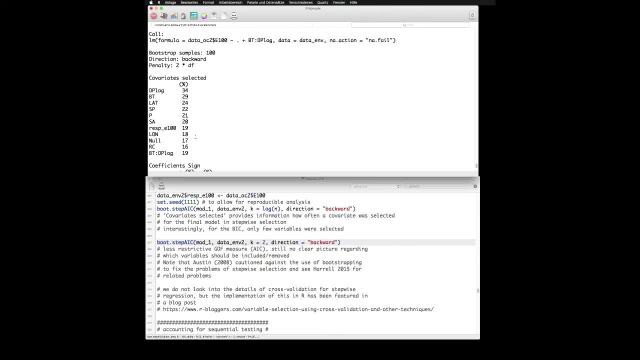 Times, How More Often The Variable Is Selected. There Are No Clear Gaps Where You Could Say: Well, This Model Or This Variable Is Problematic. 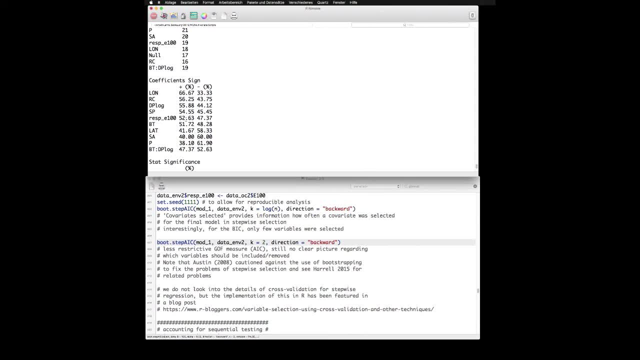 If You Have Fifty Percent Of The Time Of Positive On The Negative Sign, That Should At Least Cast Some Doubt On The Power And 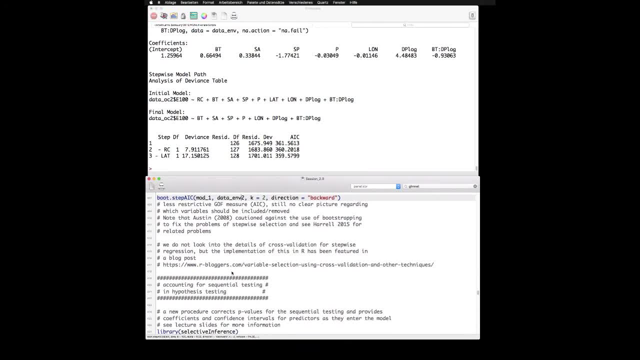 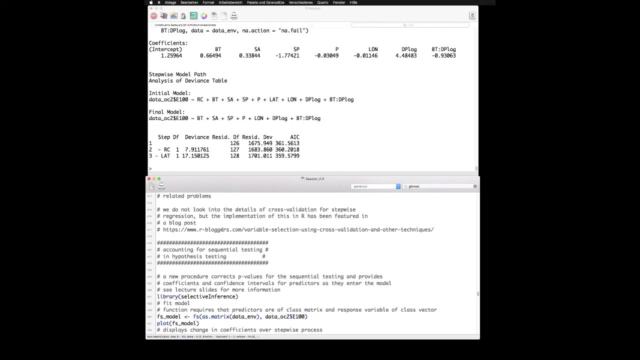 Here The Question Against The Use Of Bootstripping To Fix Problems Of Steps On Selection, And See Harold 2015.. As Well For Related Problems. 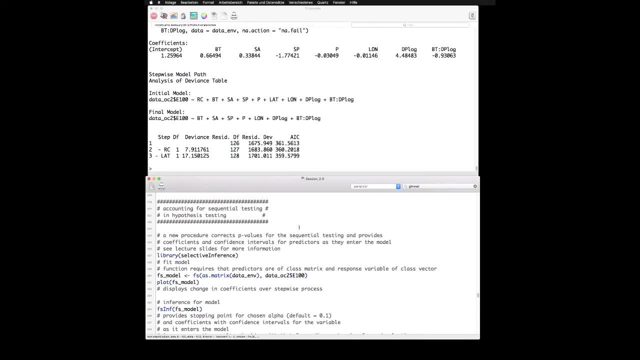 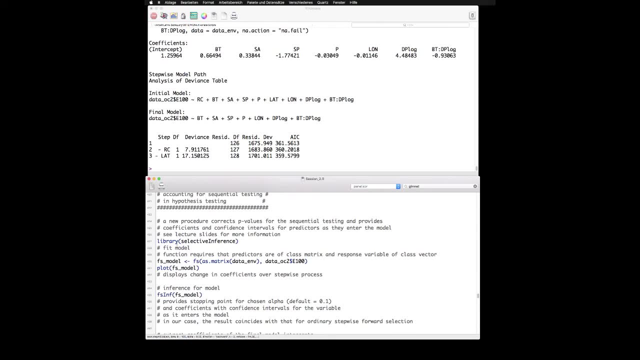 We Don't Look Into Cross Validation How Fixed In The Package, Selective Inference. Again, We Have To Fix The Model Here Again, So We 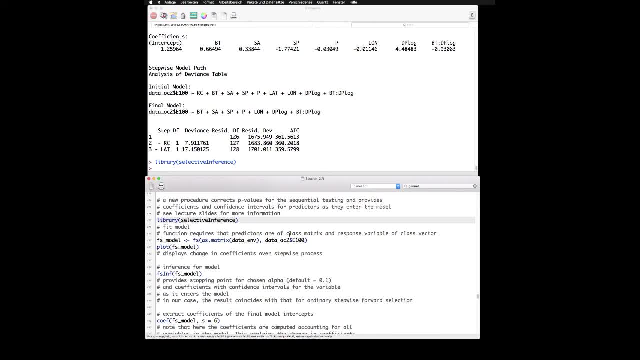 Call The Library Selective Inference, And This Function Requires Again The Different Format And The Position Inside. The Function Has Changed Here, First Explanatory: 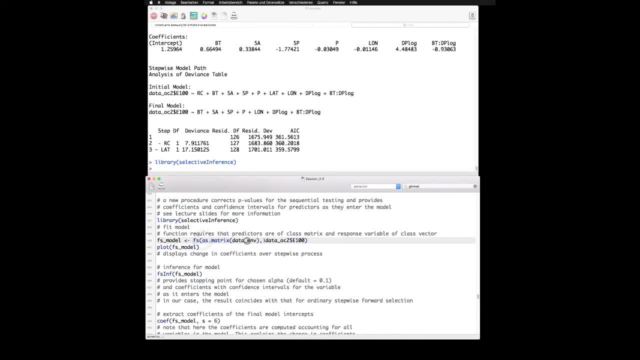 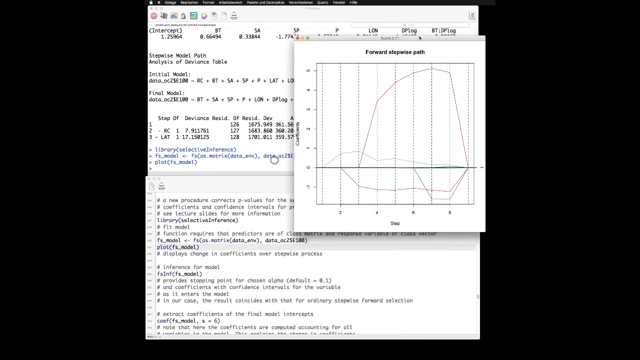 Then Response Variable. We Can Easily Do That Using The As Matrix Function That Converts Our Data Into A Requestion Coefficient. Requestion Coefficient Change. 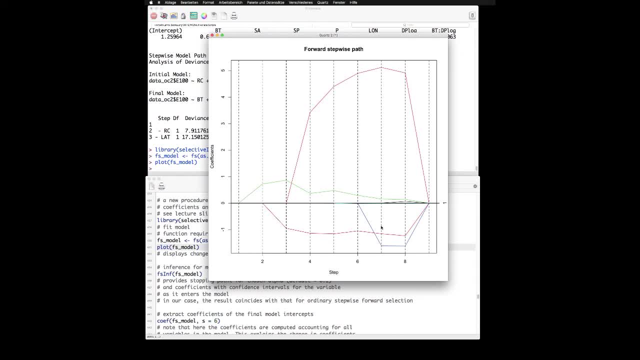 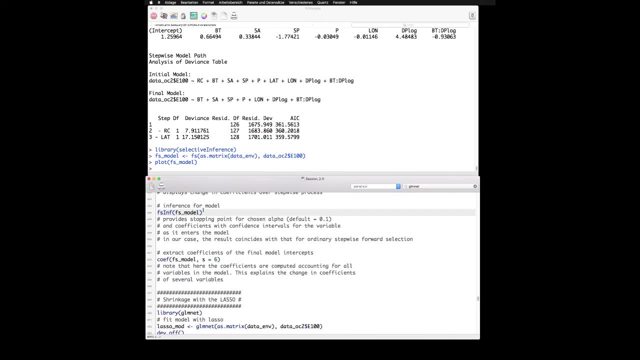 Over The Different Steps, Normal Stepwise Model Building. Now We Want To Draw Some Inference For The Model And Correct For Hypothesis Testing For 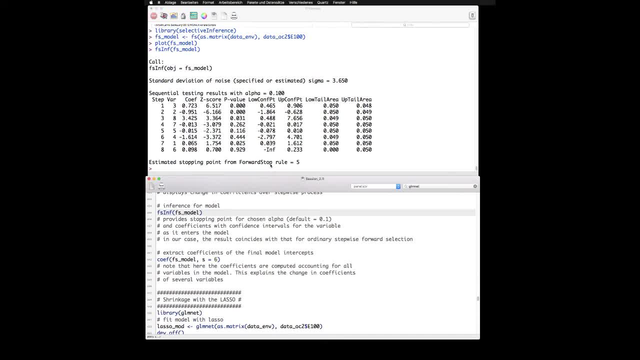 Multiple Results In The Model And We See That Only For Variable Eight, Three And Two We Obtain Statistical Significance. We Can Extract Coefficient From. 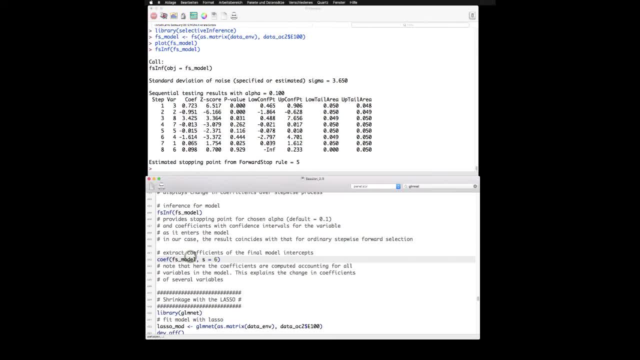 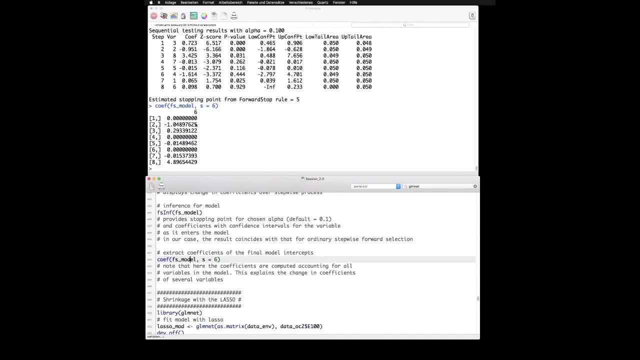 Some Variable From The Model. For Example, Here We Have Four Variable Two, Three, Five, Seven And Eight. These Would Be The Recreation Coefficient We 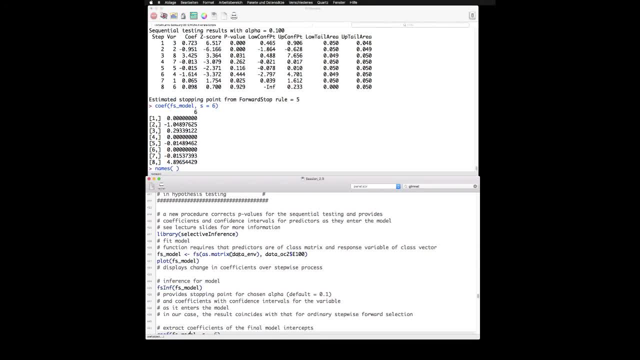 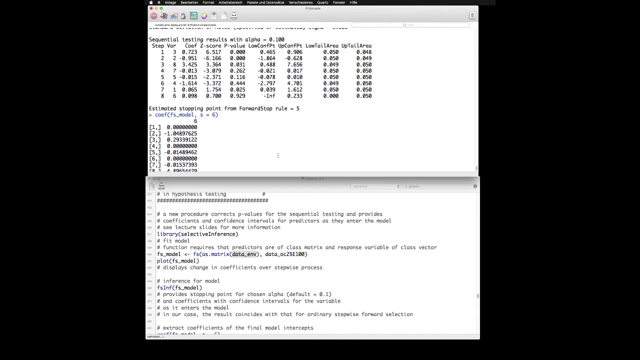 Want To Know What Are The Name Of These Variables We See. R C Would Be Zero, B, T Minus One S, A And So 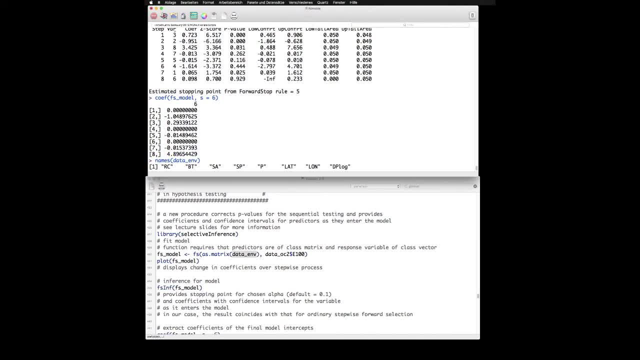 On. We Also See Here: This Is The Position Of The Variable In Column By B, T And Followed By The Depth Logarism. So 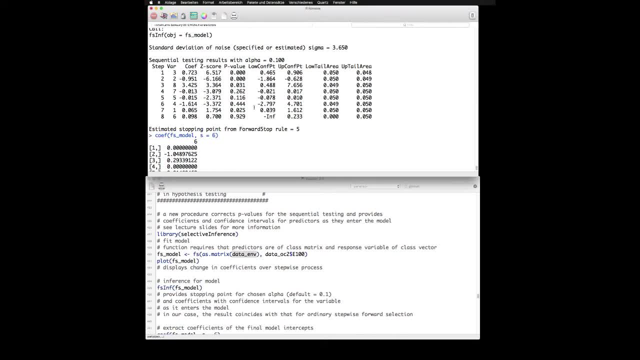 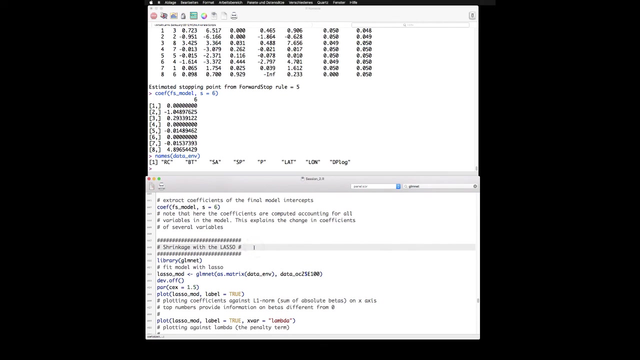 If We Would Just Take The Sequential P Values, We Could Also Argue That Only Three Variables, Namely D, P And A And A And 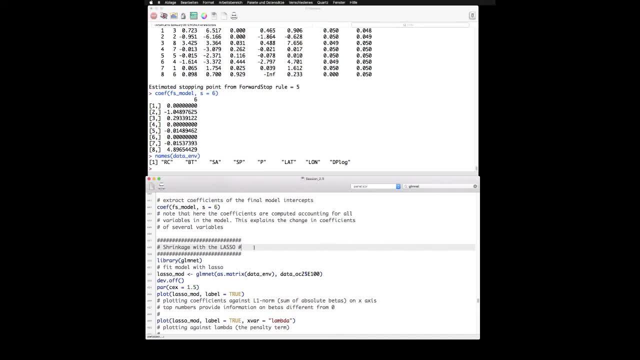 So Much About Stepwise Model Building. As You Know From The Lecture, If You Have To Use Stepwise Model Building, Then Rather Use Backward. 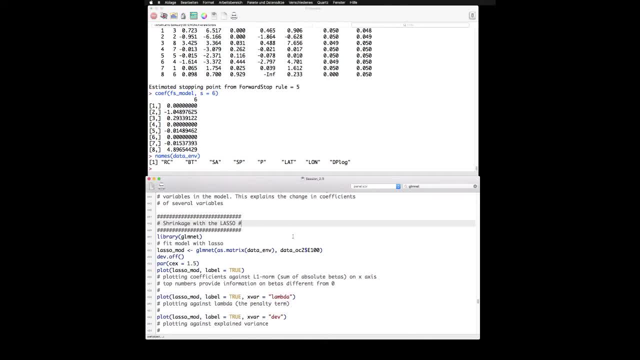 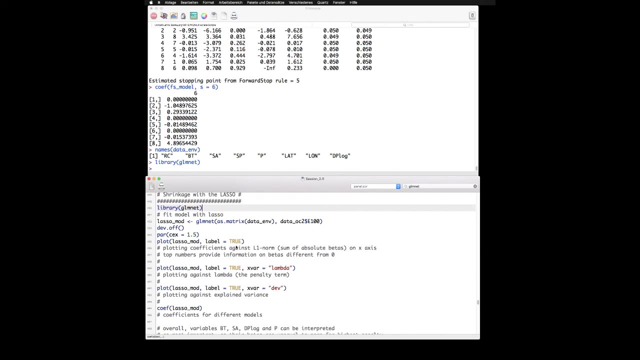 I Would Actually Favor A Different Approach, That Is The Lasso Approach, And I Show You How You Use This Approach Now. First Have To. 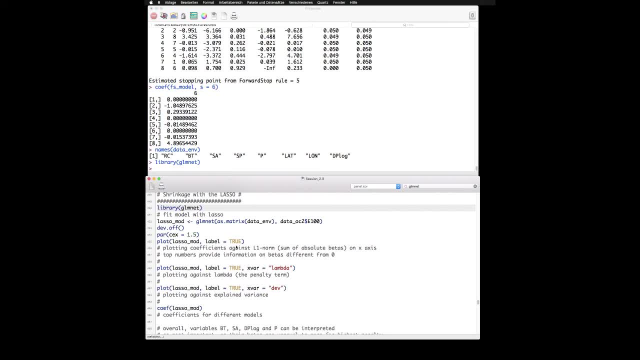 Call The Function G Over Fit The Model And To Have Low Regression Coefficient. So We Have Shrinkage Of Regression Coefficient During Model Fitting. 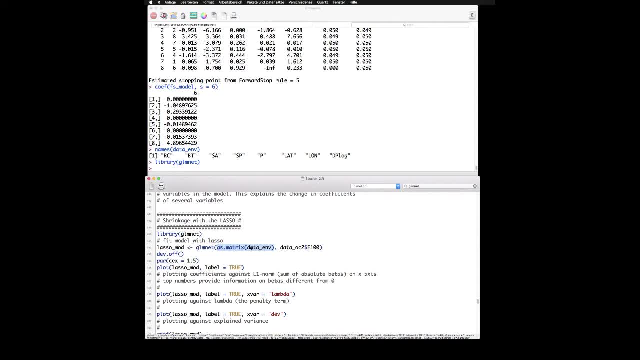 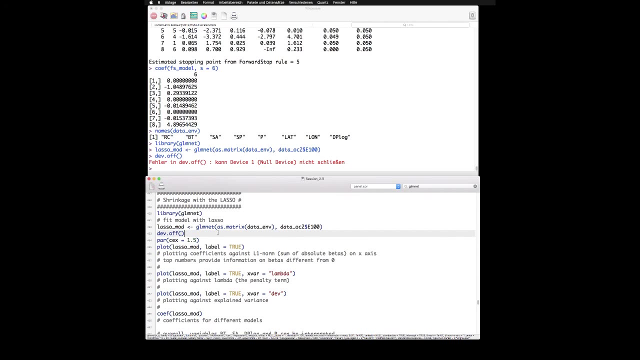 Model Fitting Is Again Done Here Really Easily. Follows The Response Variable: Fit The Lasso, Make Sure That No Previous Device Is Open And 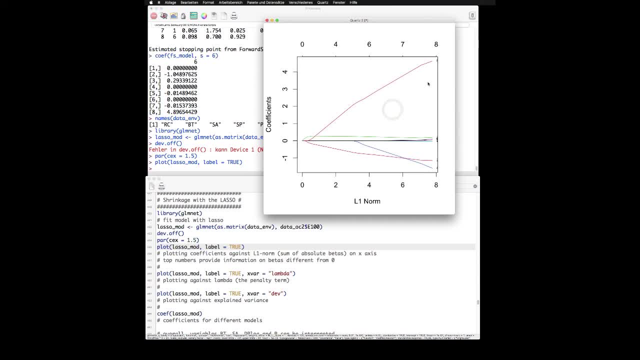 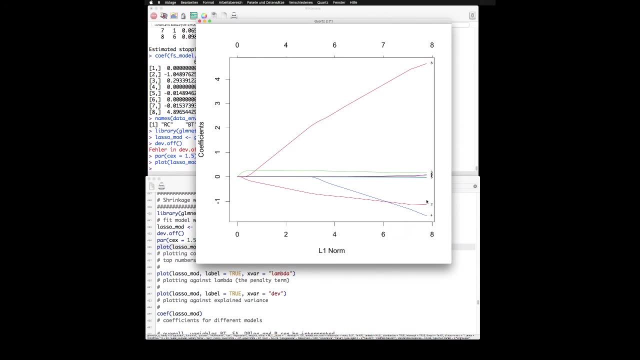 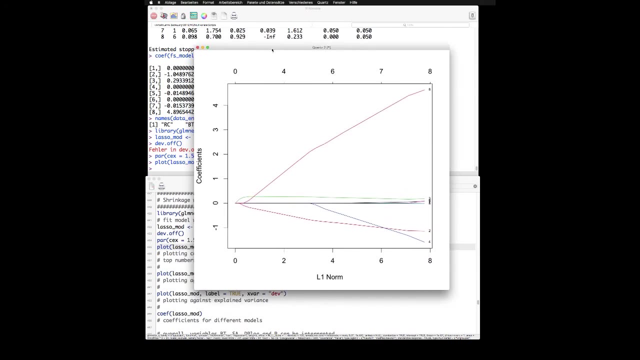 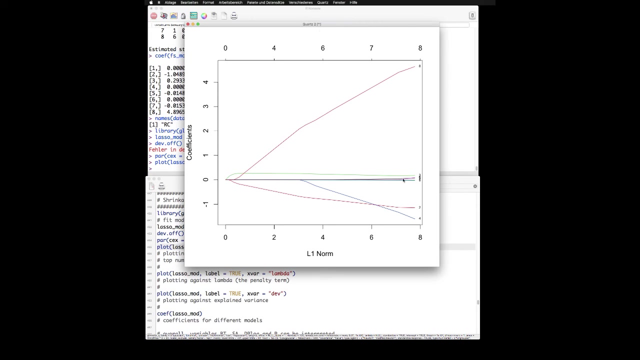 Then We Set New Parameters For The New Device Plot This, And What We See Here And For Is S? P. So We See, That's. 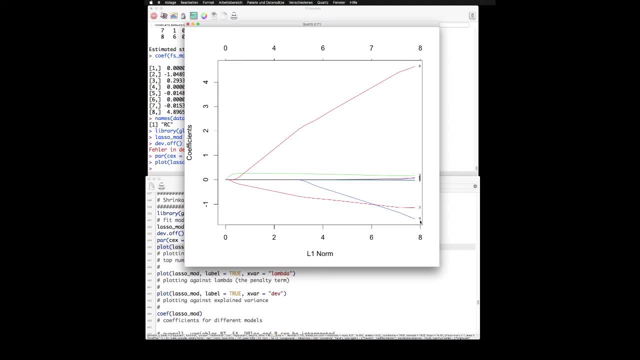 A Slight Difference, But S A Is Also Contained In Model That's Three. That's A Slight Difference Here Compared To All Betas. We. 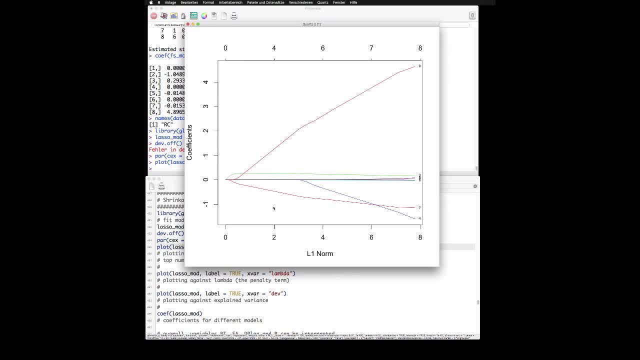 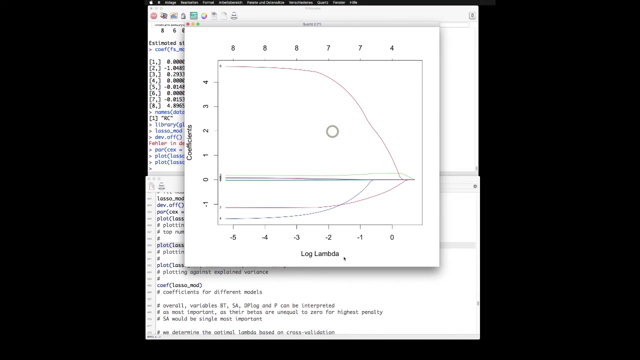 See That The Smaller The Sum Of All Betas, This Leads To Removal Of Variables. What We See Here Is The Number Of Variables In. 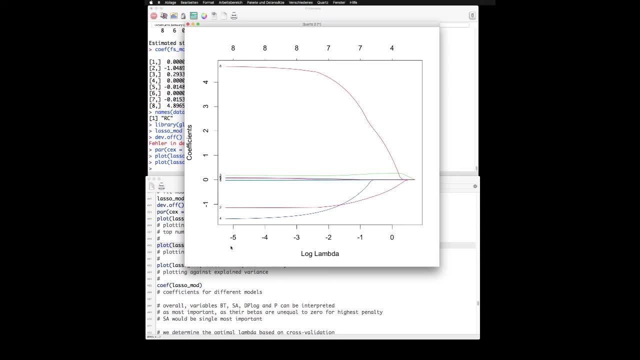 The Model. So The Lower The Lambda, The Less Is The Penalty On The Model. We See, The Higher The Lambda Gets, The Lower The Coefficient. 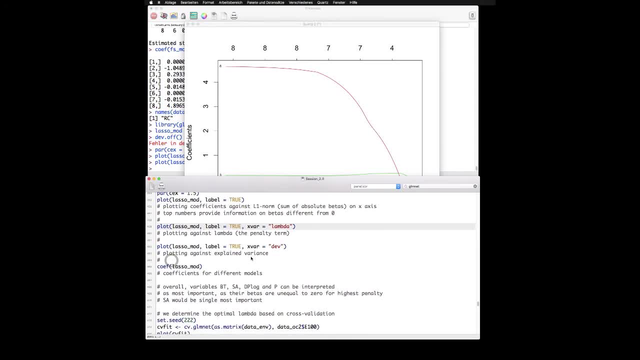 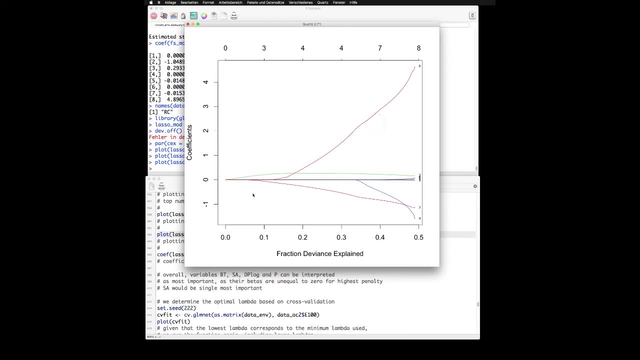 Of The Variables Become Unless Finally We Can. We Can Plot Coefficient Against The Fraction Of Deviants. Explained Deviants Is Just Generalization Of 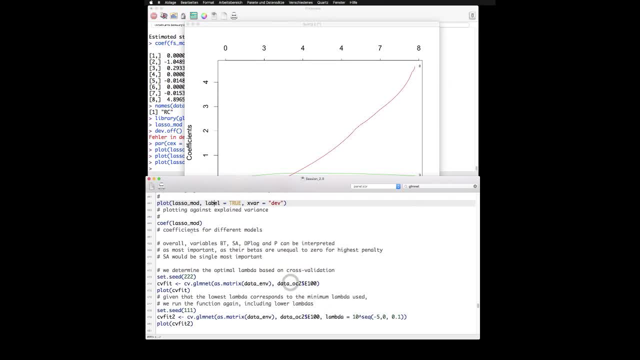 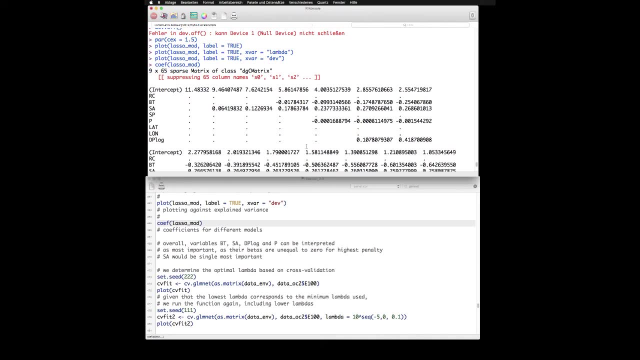 Explained Variants For Generalized Linear Models And So On, Can Extract The Variants Of The Different Models For Different Lambdas And We See. 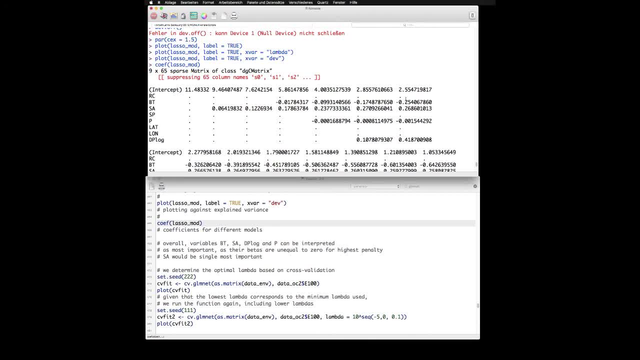 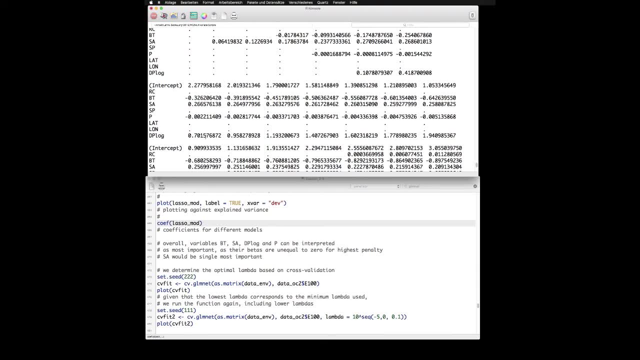 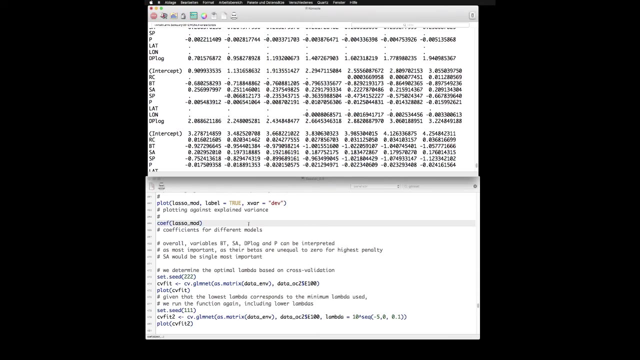 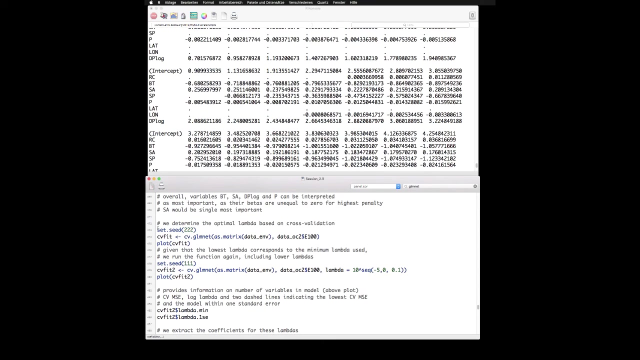 For The Highest Penalty That We Have Only A Model With An Intercept And Then Additional Variables Are Observation. Using Other Techniques We Can Obtain The 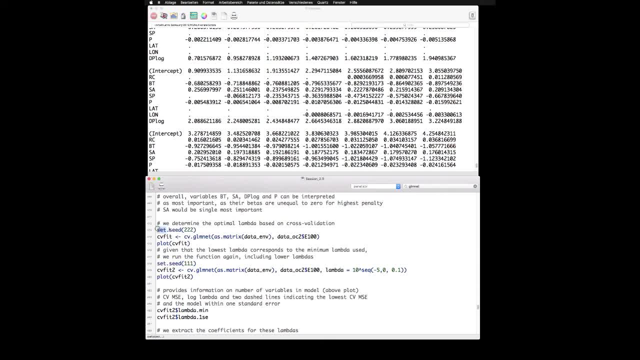 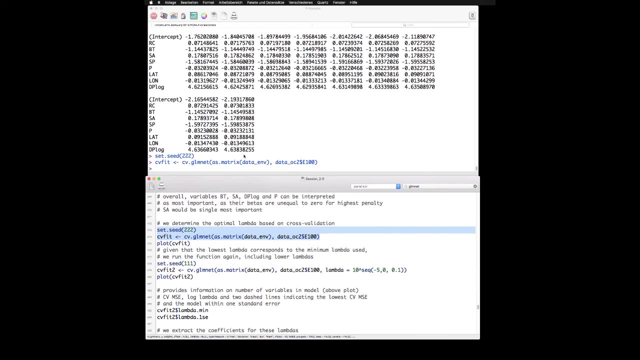 Optimal Lambda Based On Cross Validation. So We Remove Data And Fit The Model Again And Again And Look At The. Everybody Runs, This Obtains. 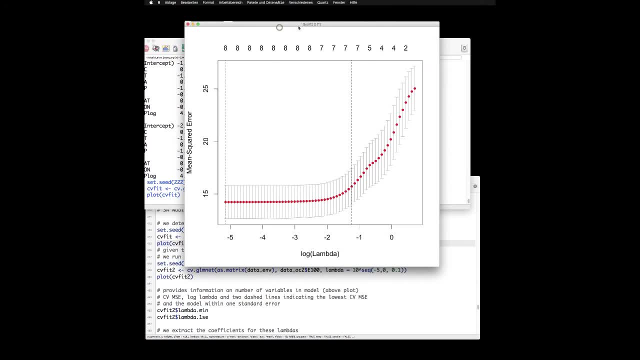 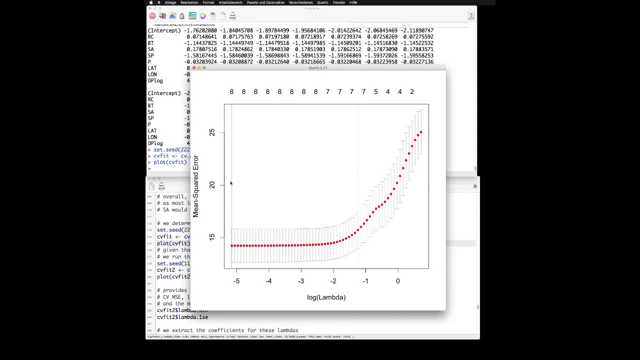 The Same Result. And Then We Plot The Fit And In This Case We Have, On The One Hand We Have The Lowest Lambda, That Is, 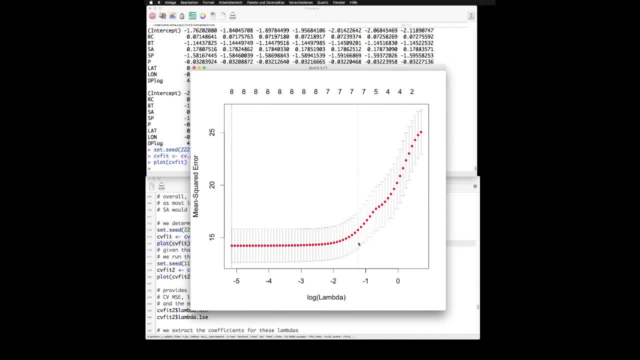 Still Within One Standard Arrow. It's Not Not Very Different In The Mean Squared Arrow, Although It's A Little Bit Higher Than The Original. 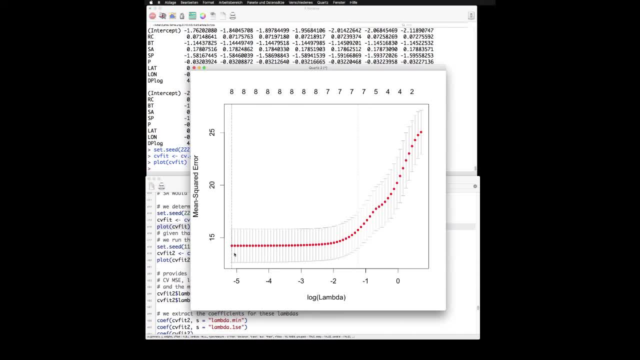 Model And We Fit This Again: Lower Numbers. So That Means We Want To Have More Observations Here, Because It Could Be That Mean Squared. 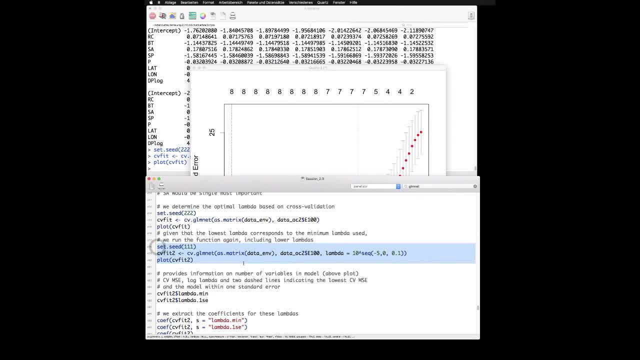 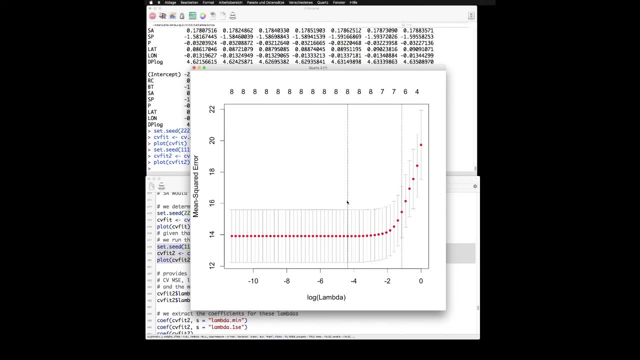 Arrow Drops Much More If We Had Additional Sample Points. The Optimal Lambda Is Approximately At A Lock Lambda Of Minus Four Point Something And 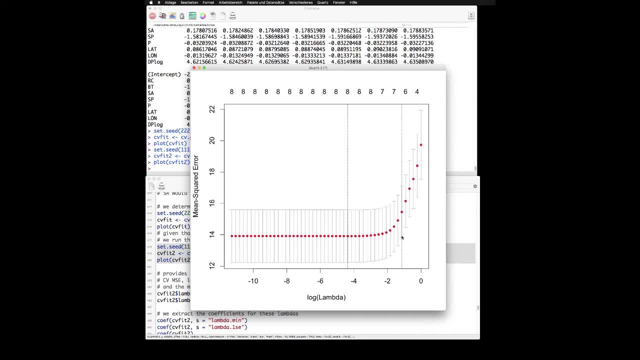 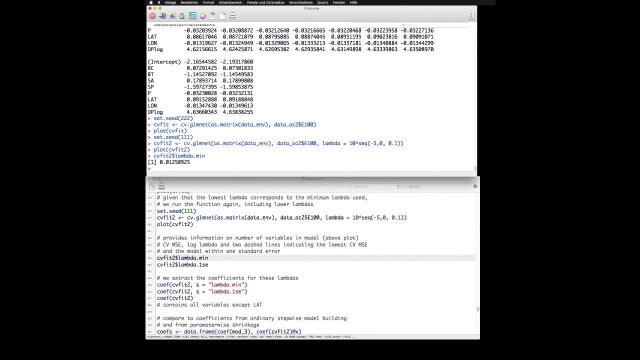 We Have The Optimal Minimum Minimum Within One Standard Arrow, Still Overlapping With The This Above. These Numbers Given Give Us The Number Of Variables. 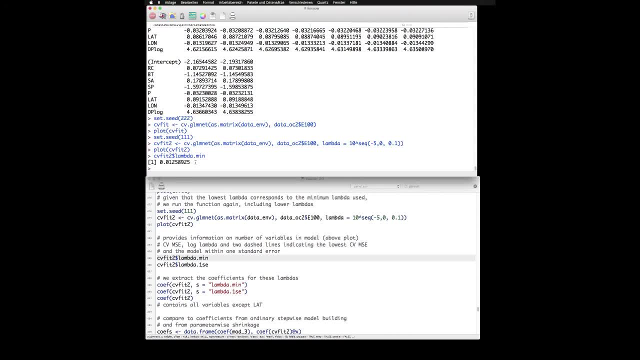 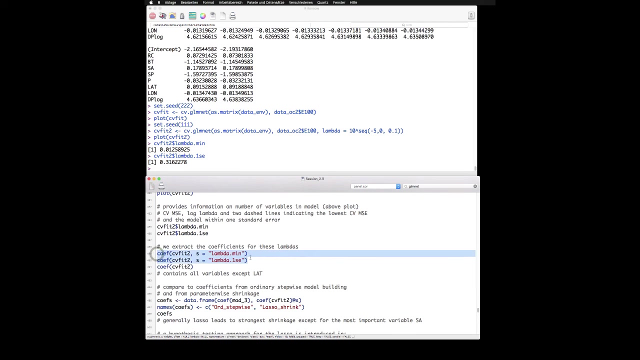 Included In The Model. So If We Go For The Minimum Lambda Here We Have, We Obtained The Minimum In One Standard Arrow Extract. These 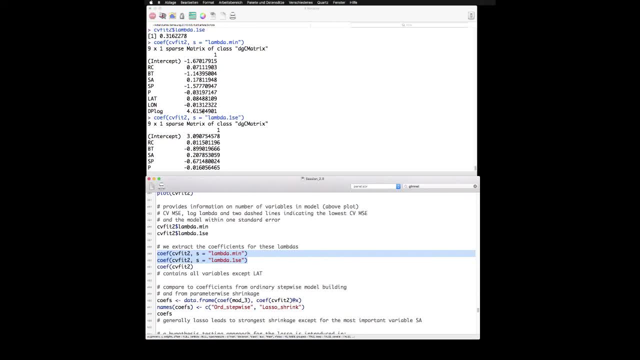 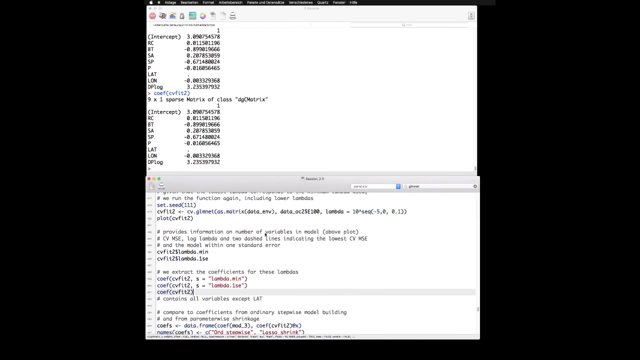 Coefficients For These Models. We See It: On The One Hand We Have All Variables Included, On The Other Hand, For The One Standard Arrow. 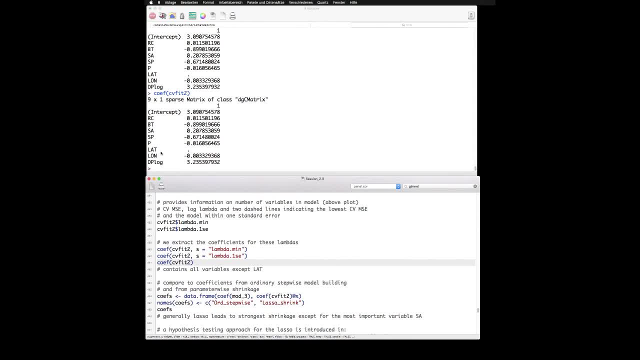 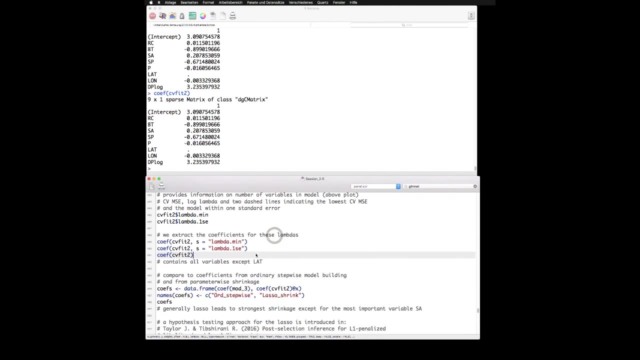 Model. We Have The Standard Arrow Model, Which I Would Suggest That We Have The Most Parsimonious Model. If We Only Exclude Latitude, We 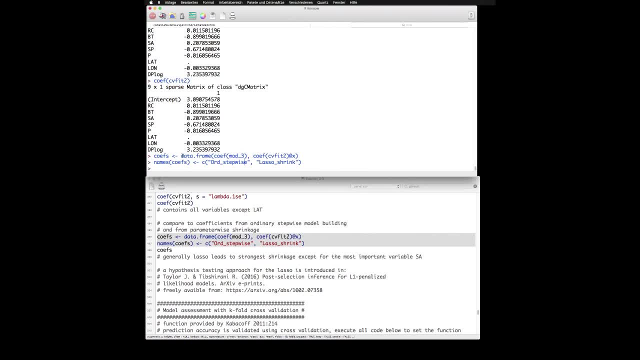 Compare Our Regression Coefficients Structing Data Frame With Our Initial Coefficient. From Ordinary Stepwise Selection We Take The One From Model Three Still. 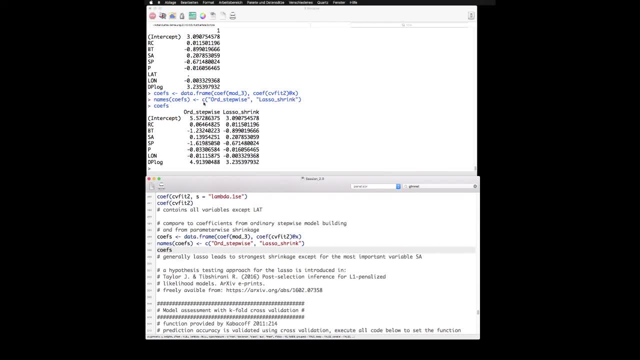 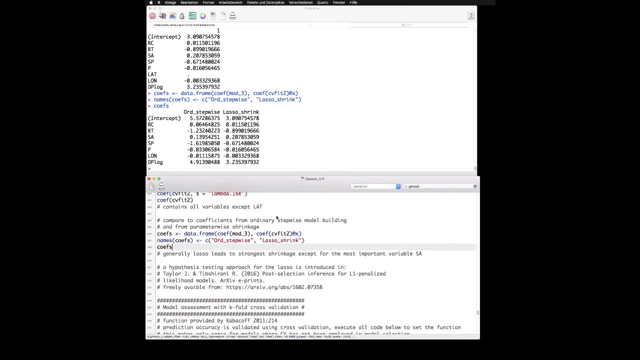 As A Included And Our See, And We Compare This, All Regression Coefficients, Except For S A That Is Considered As The Most Important. 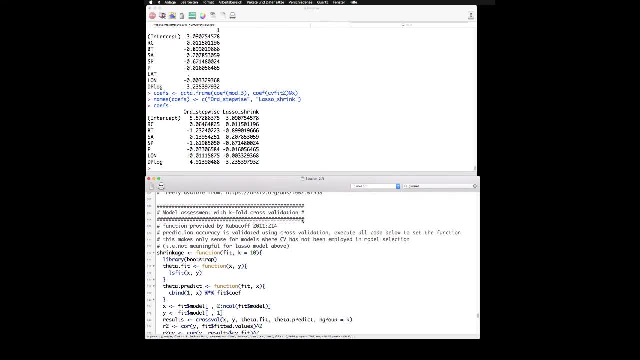 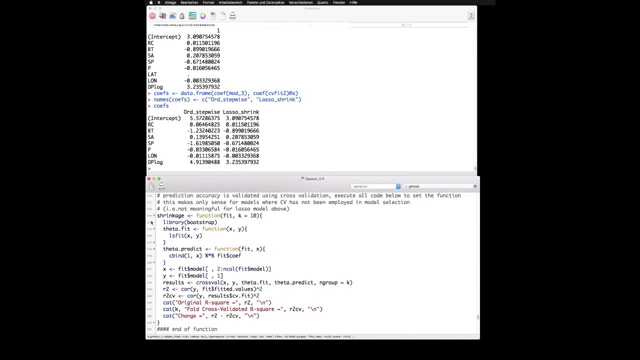 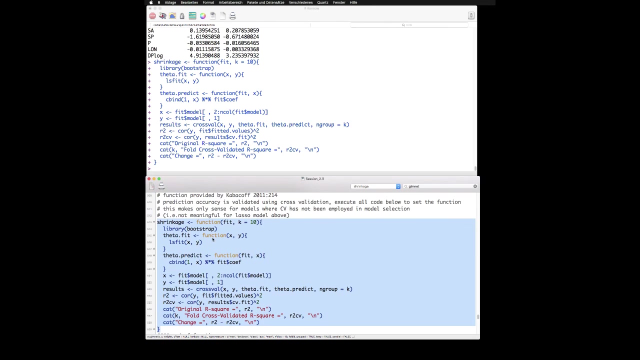 Burn. Yeah, That's It For Lasso. Finally, I Show You If You Had Used A Thing Okay For Cross Validation. You Need This Type Of. 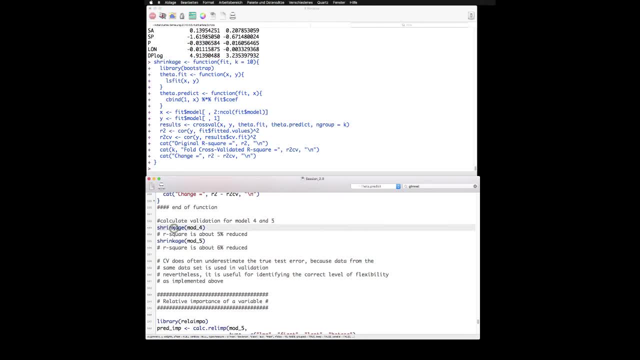 Code For That, And So We Calculate The Validation For Model Four And Five. What We See Is That Value Drops To Four, Zero Point Four. 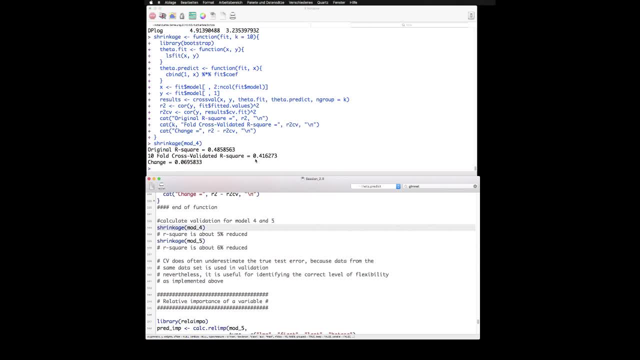 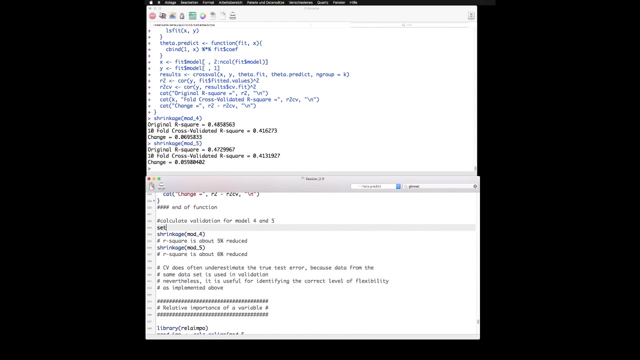 One. So Cross Validation Means That You Remove Parts Of The Data And Try To Predict This Part Of The Data From The Data That Is. 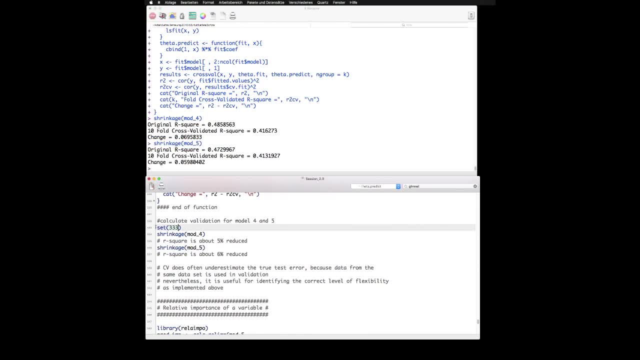 How The Data Are Split Up. We Can Set Seed Here As Well To Have Reproducible Result. So If I Fit This Again, Error. 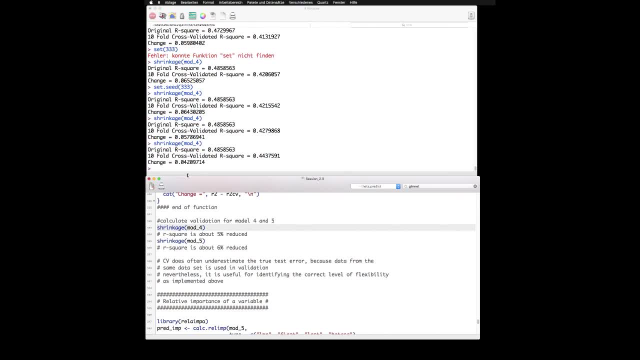 Set Seed With That. So The Shrinkage Is About Four To Six Points, Depending On The Algorand, Depending On Split Of Samples Put Here. 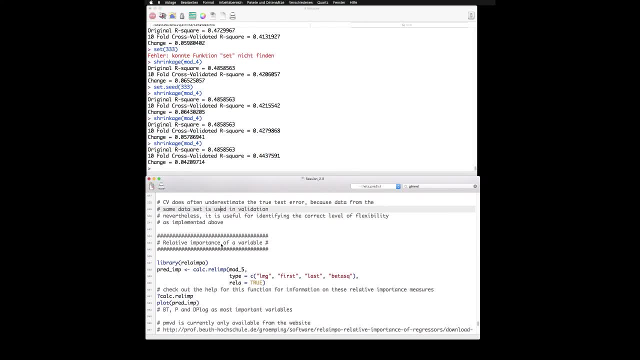 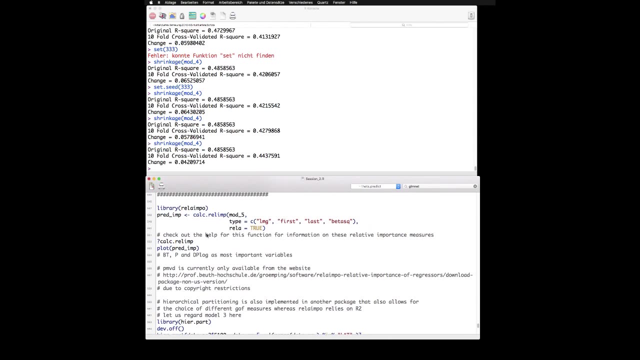 Roughly Five And Roughly Six. Notice That Generally This Has The Same Characteristics As The Data That Has Been Used For Fitting. And Finally, 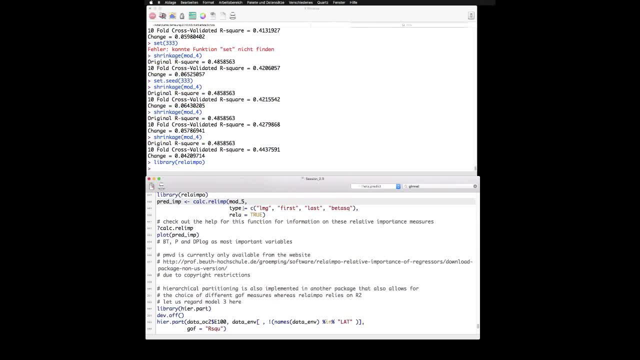 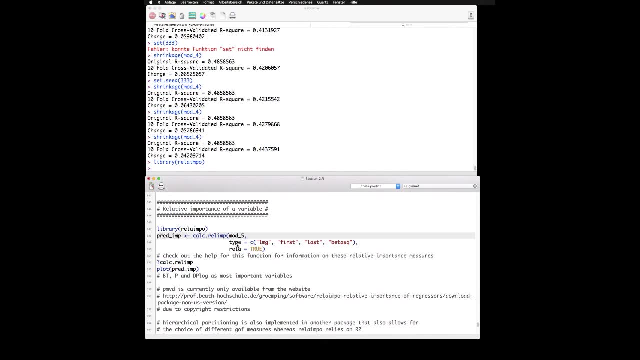 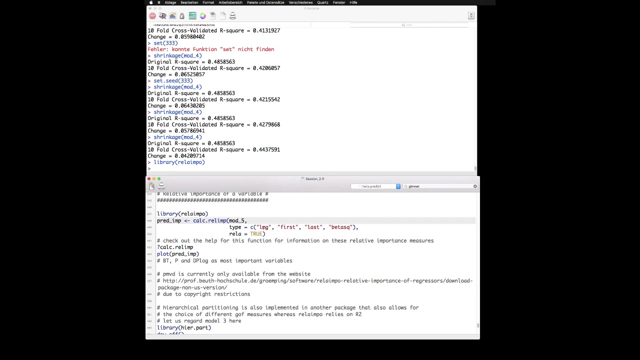 For Relative Importance Of The Variables. We Use The Impo Package. This Function Is Provided For A Data Set That Is Always Here In Terms. 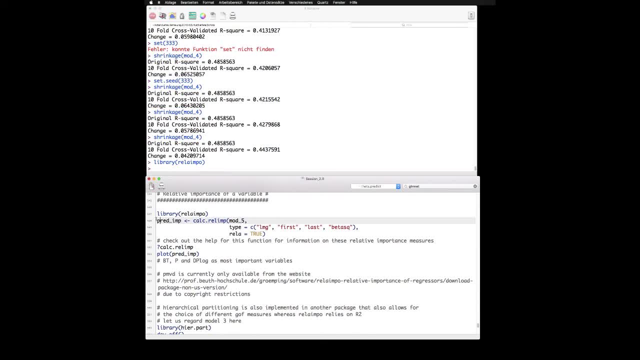 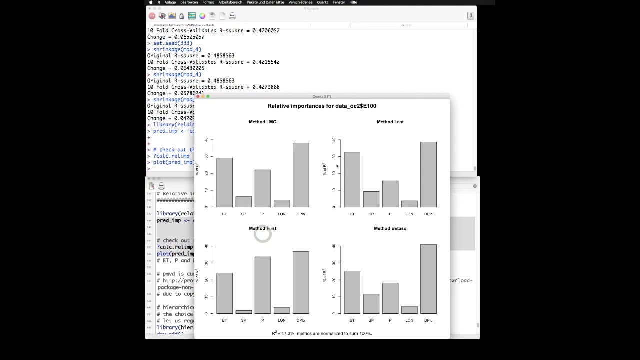 Of R Squared. Please Check Yourself The Help To This Function To Find Out What These Difference Variable Or That's For Hierarchical Partitioning. It's. 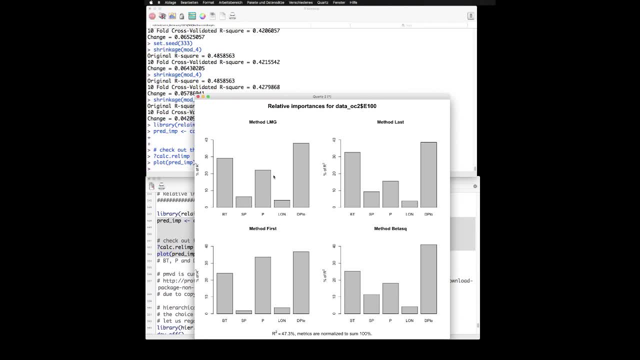 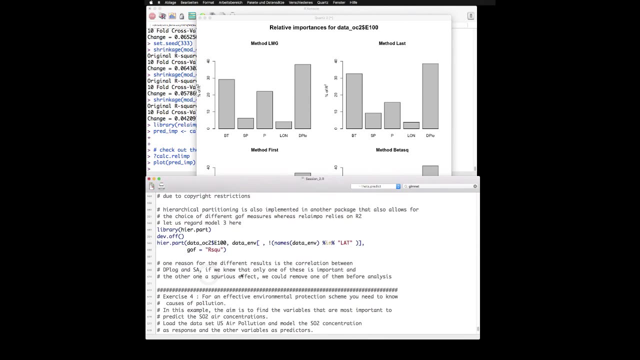 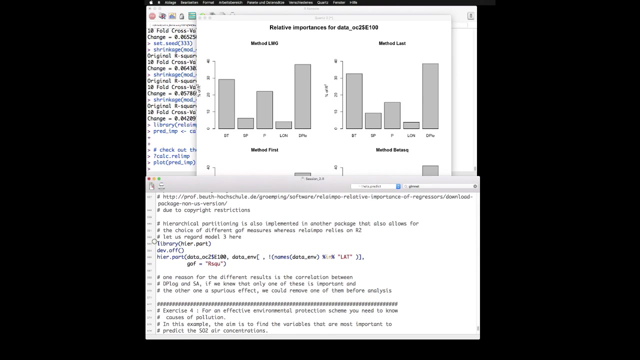 Probably The Method That Is Most Reliable, Especially If You Look At The R Squared. And Then We See Here That B T, Model Three. 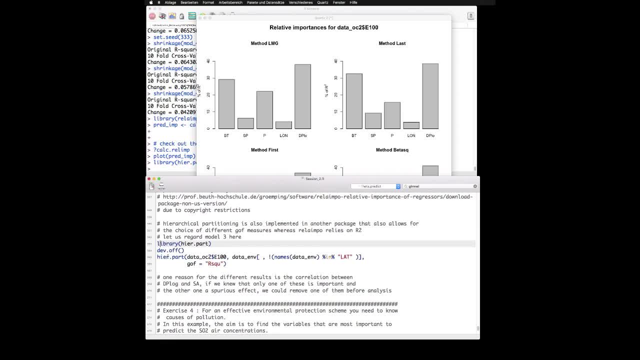 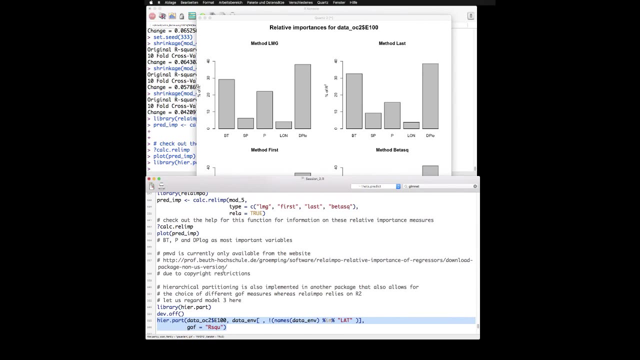 Is The Function. The Library Part Contains A Function, Called Here Part That We Execute. So It Has More, Less A Similar. It Has A Little. 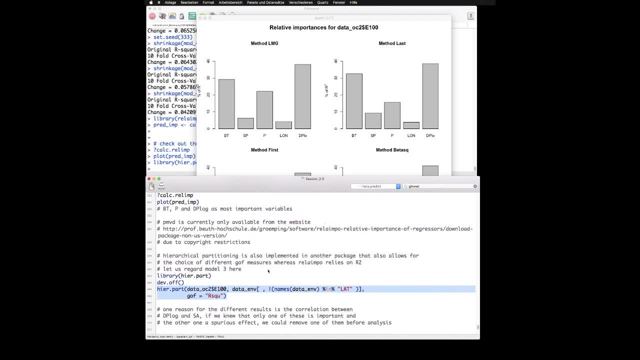 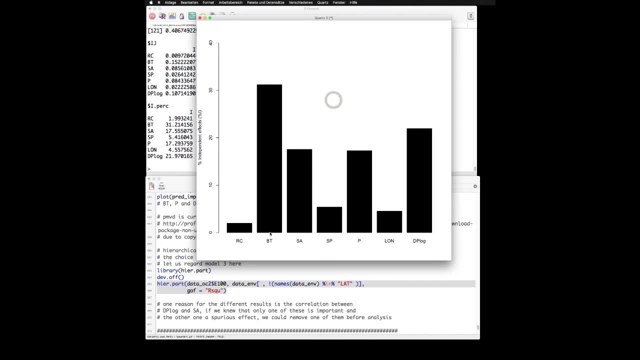 Bit Different, Actually Different. Good, Most Aficionado Fit Measures Can Be Used For This Function And The Result We Have The Model That Would Be. 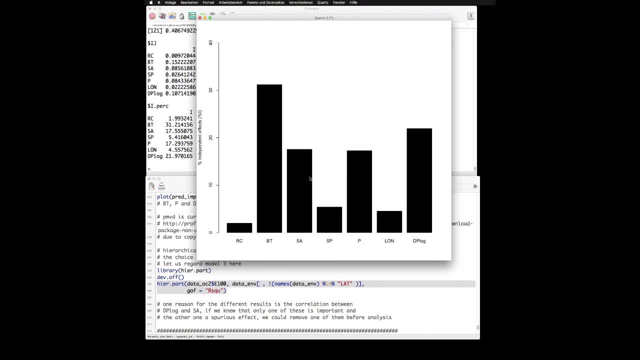 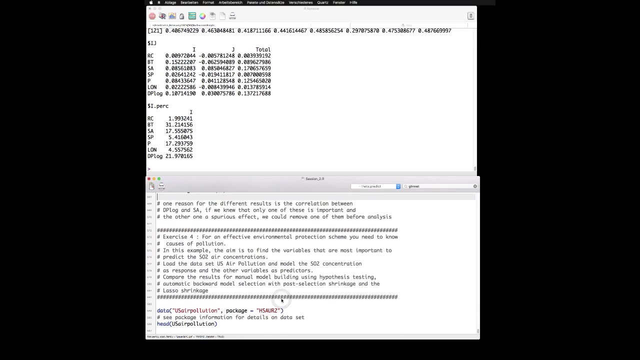 The Optimal Lasso Model, And We Again That These Four Variables Are Most Important, Which Was Our Initial Question. With That We Are At The 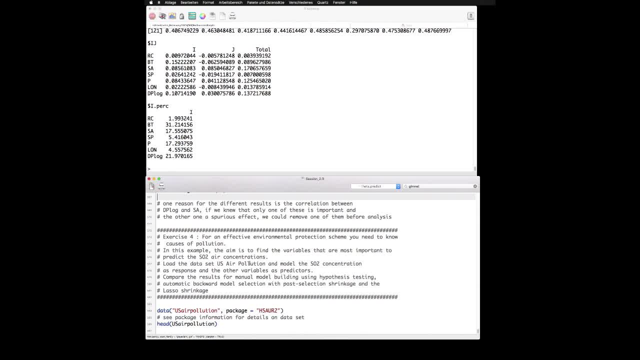 End Of This Screencast. I've Showed You Many Different Techniques To What You Should Do Is, Of Course, To Tend To Look At. 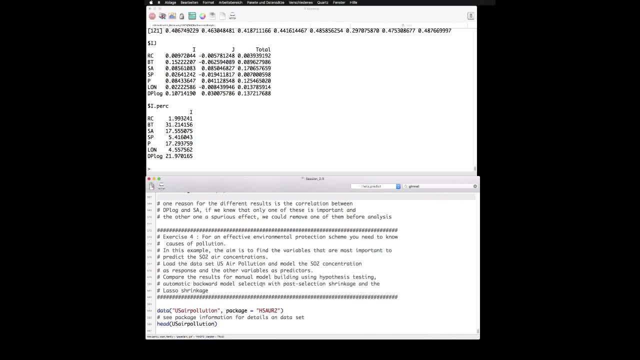 The Data Before, Whether You Have Culinarity- That Is Problematic- Whether You Have Differences In The Distribution, Then Compare This To The Lasso Results.